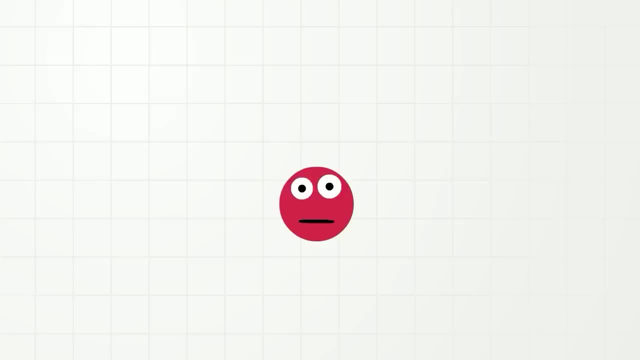 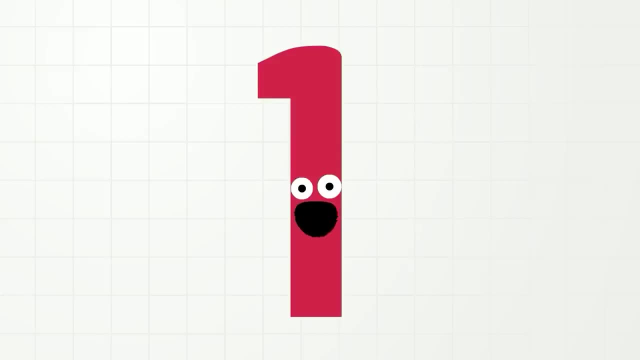 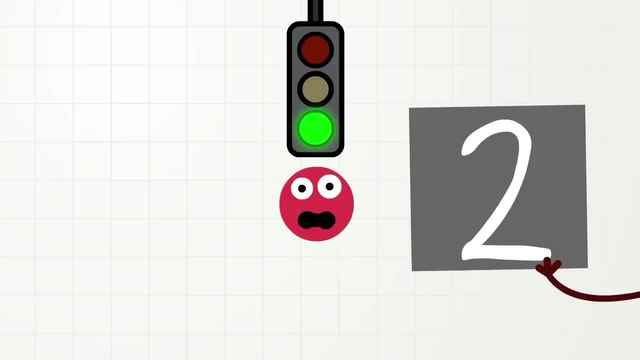 Go: 1,, 2,, 3,, 4,, 5,, 6,, 7,, 8,, 9, 10.. Wow, And you can write it like this. And you can write it like this: You did such a good job. I think it may be time to celebrate. Yay. Ok, That's enough. 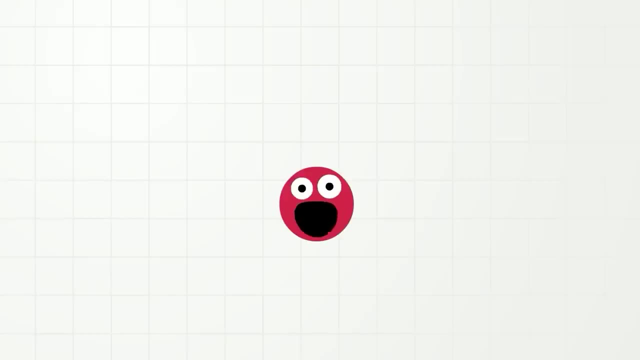 So we can say numbers And we can write numbers, But did you know we can also use numbers to count actual things we do everyday? Ho, ho, yes, we can. Let us use an example. Oh, what should we use? Hmm, heh, I know How. about spaghetti? 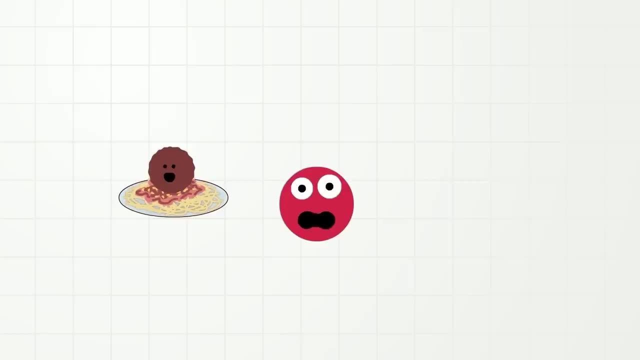 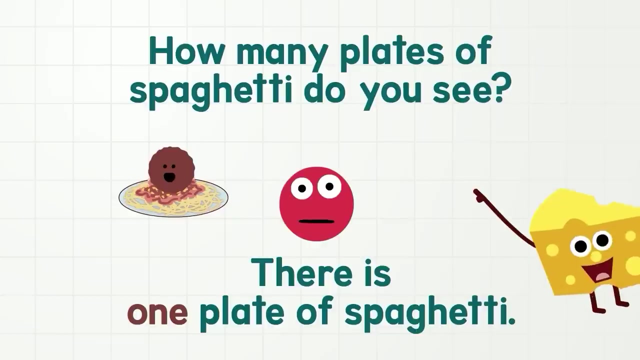 Spaghetti- Wow, that is a big meatball. Okay, so if I ask you, how many plates of spaghetti, do you see? what would you say? That's right, there is one plate of spaghetti. We can say the one one. 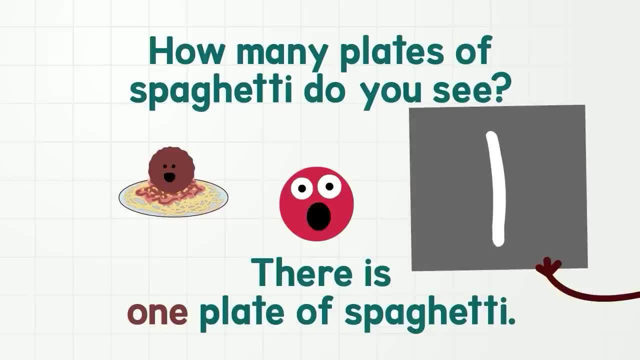 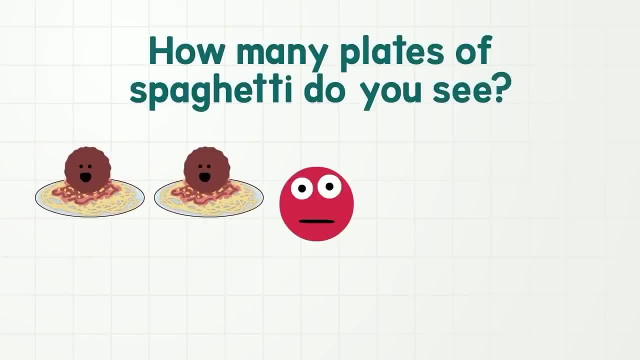 We can write the one, And there is actually one plate of spaghetti. See, one. Now, how many plates of spaghetti do you see? That's right. there are two plates of spaghetti. We can say two, two. This is how we write two. 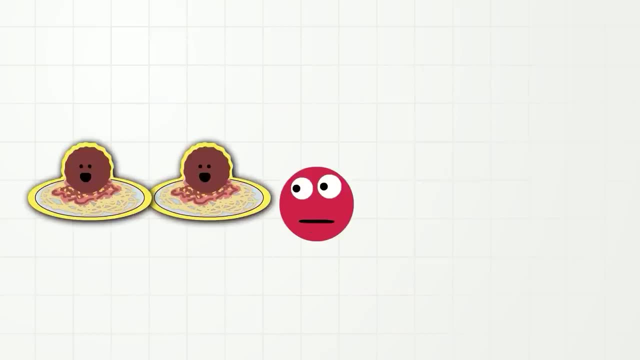 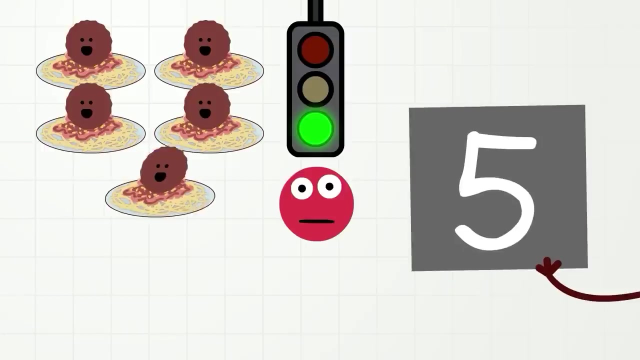 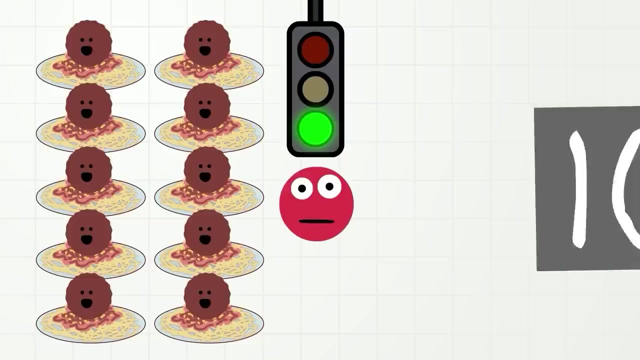 And there are one, two plates of spaghetti. So now let's count to ten again together, while watching the plates of spaghetti. Okay, ready, Go One, two, three, four, five, six, Seven, eight, nine, ten. 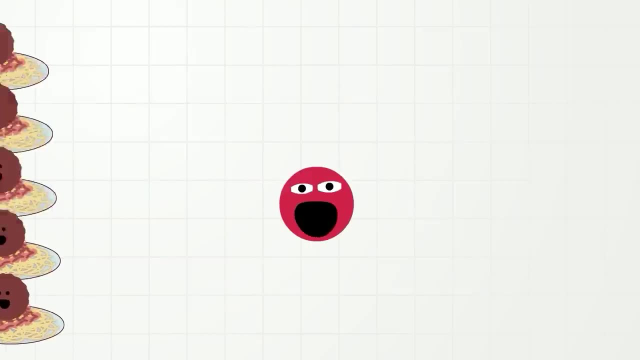 Oh great, I think you really like spaghetti. Now let's count something else. Hmm, how about the letter X? I said letter X. Say hi to the letter X. How many letter X's do you see There are? let's count. 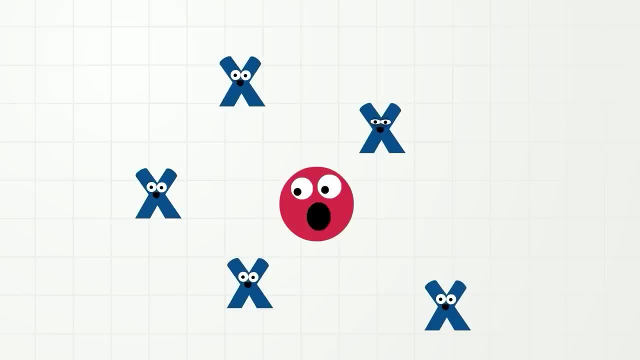 One, two, three, four, five. There are Five letter X's. We can say five, Five And we can write five, And we know from counting them. there are actually five letter X's, See One, two, three, four, five. 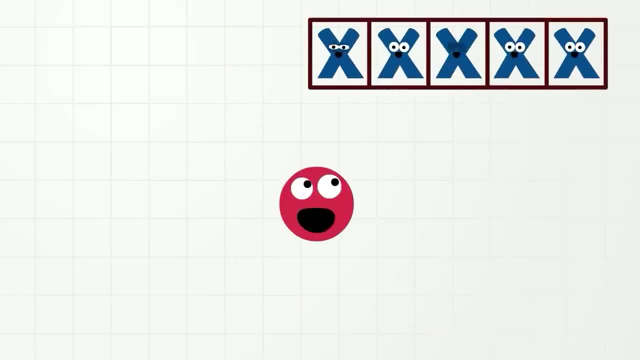 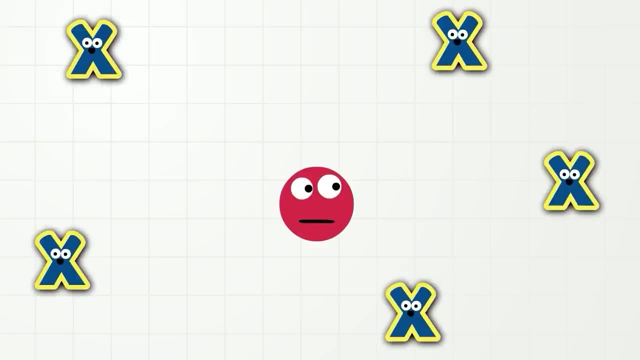 So, even if the X's go all the way over there, there are still five, One, two, three, four, five. And even if they are spread out, there are still five, One, two, three, four, five. 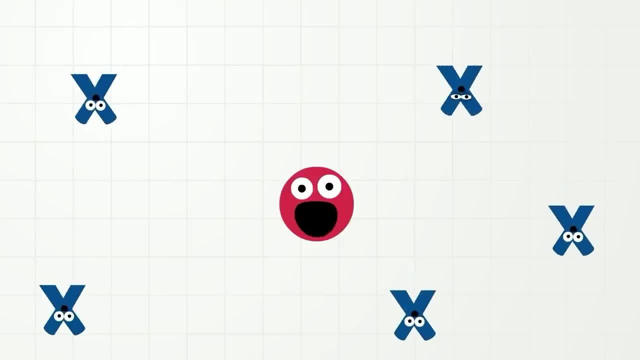 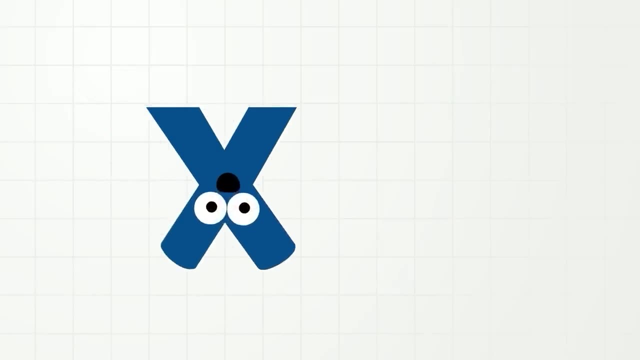 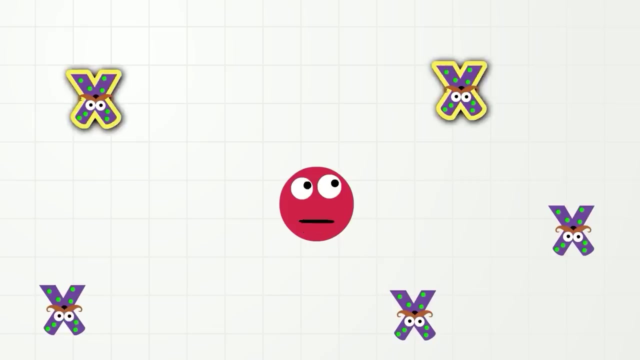 Even if they are upside down, there are still five. One, two, three, four, five. Even if they are upside down, purple, with green polka dots and all with mustaches, there are still five. One, two, three, four, five. 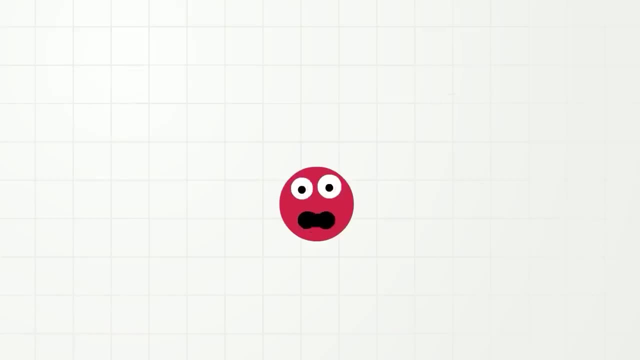 Ho ho. good job counting. I think it may be time to celebrate. Yay, I think that's enough. Now let's find something else to count. Hey, do you know what this is? Is it a plate of spaghetti? 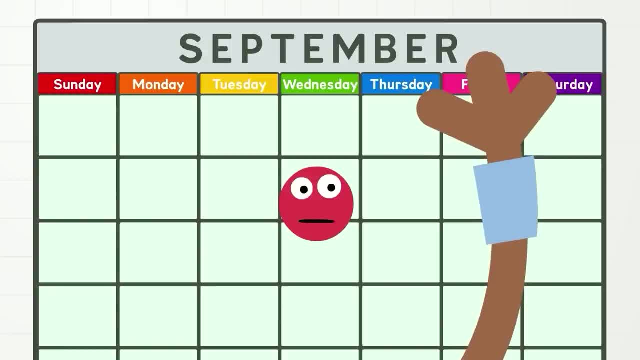 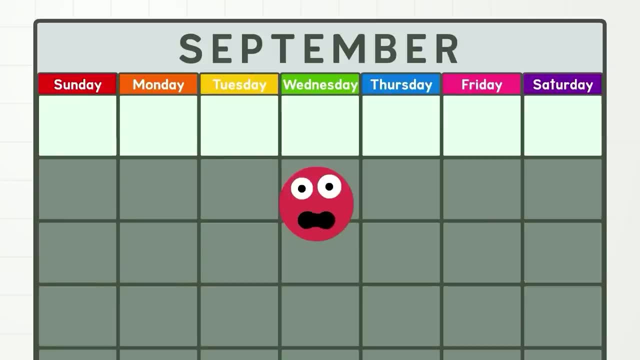 No, It is a calendar. Uh, that's what I said: A calendar. No, you did not. Anyway, a calendar shows you all the days and all the weeks of a month. Let us look at just one week and try and count the days. 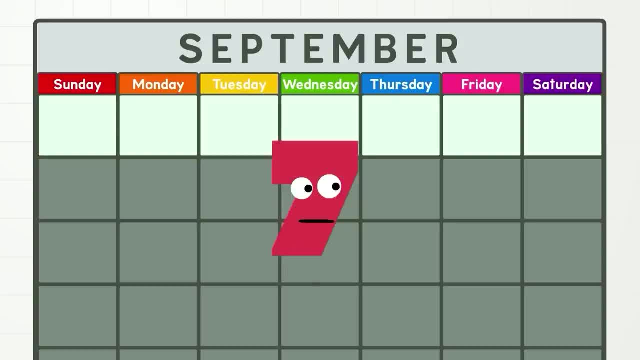 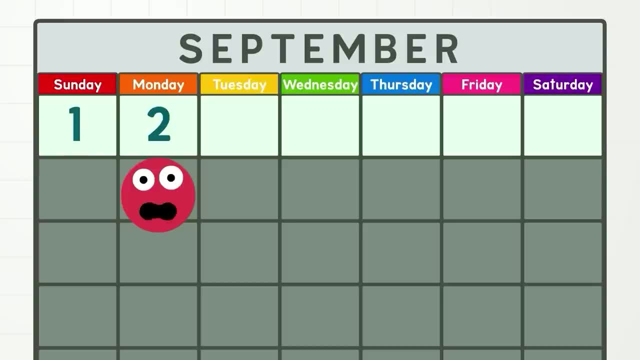 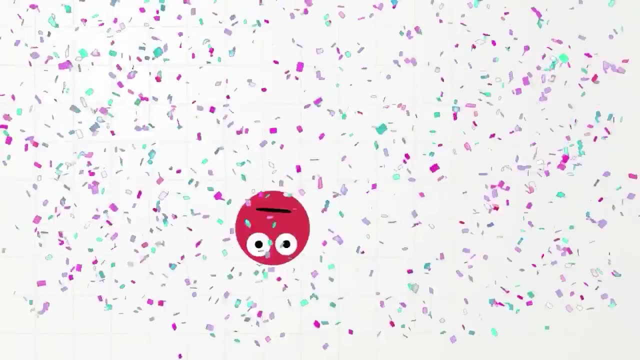 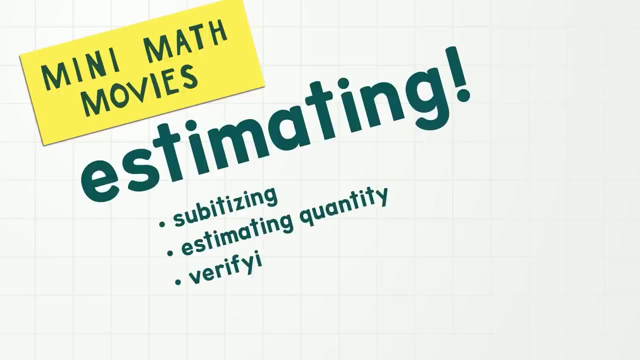 Ready Go: One, two, three, four, five, six, seven. Wow, you did so great that I think it may be time to celebrate Yay. Okay, that's enough. It's my turn now. Let us start right here. 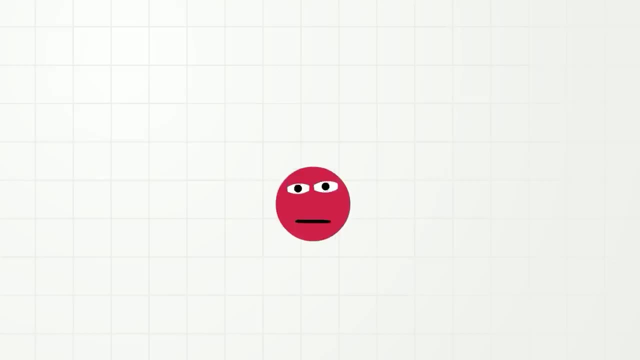 Here we go, Here we go, Let's go. Oh, hi everybody. Today I'm going to talk to you about numbers And counting And estimating, And maybe even bananas. I really like bananas, Okay. so one thing we use numbers for is when we are counting. 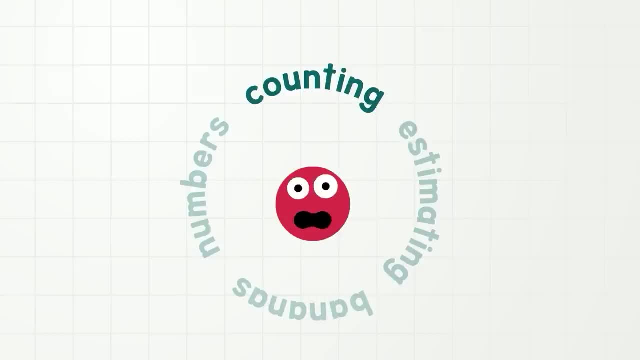 And sometimes, when we are counting, we don't really count. Sometimes, when we are counting, and especially when we have to count something quickly, we use estimating, Estimating. Estimating is kind of like guessing. You all know what guessing is right. 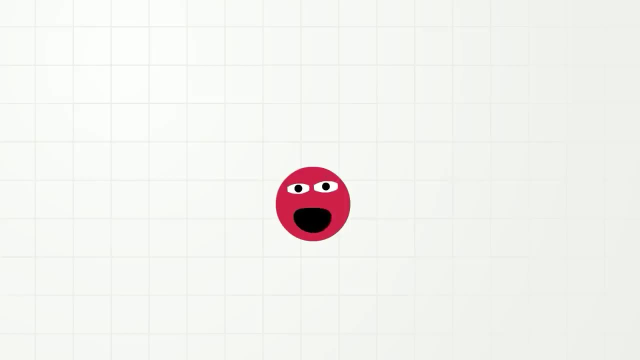 Let's try Right now. I want you to guess what is behind me. I will give you a hint: It is a fruit, and it is long and yellow. Can you guess? That's right, It's a banana. Yay, Because you did such a good job, it is now time for a break. 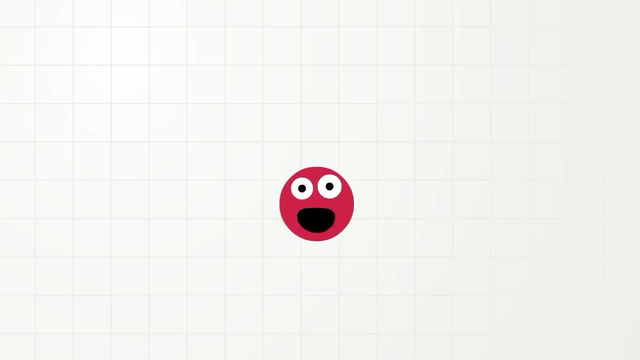 Okay, that's enough. So when we want to guess something that is about numbers, we call it estimating, Estimating. In a minute I am going to show you some more bananas, Bananas, And you are going to guess or estimate how many bananas there are. 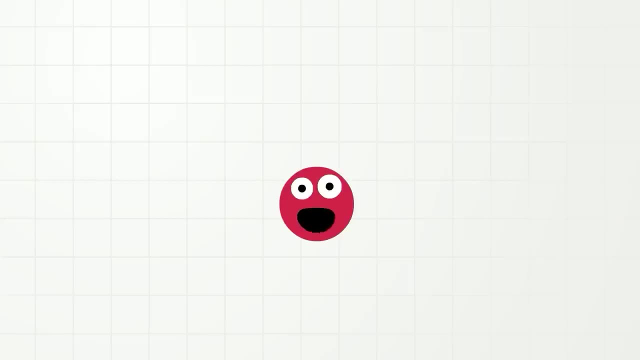 Bananas. You already said that. But first let us make sure we all know the numbers from 1 to 10.. Let's all count to 10 out loud together. Okay, ready, Here we go. 1, 2, 3,, 4,, 5,, 6,, 7,, 8,, 9,, 10.. 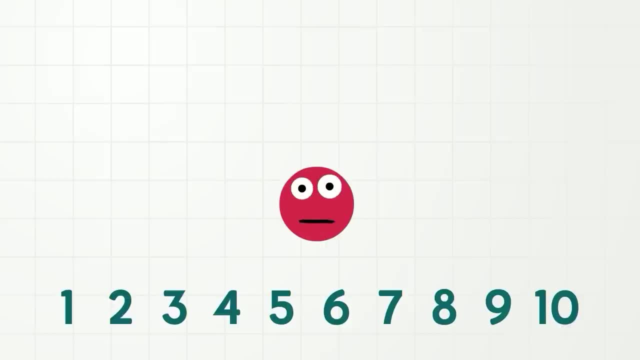 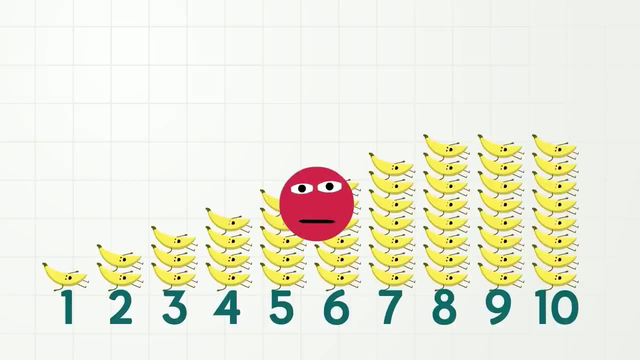 Ha, Good job. So these are all the numbers, or numerals, from 1 to 10.. And did you know that we can also show numbers using bananas? Oh, Yes, we can. For example, this is what 2 bananas look like. 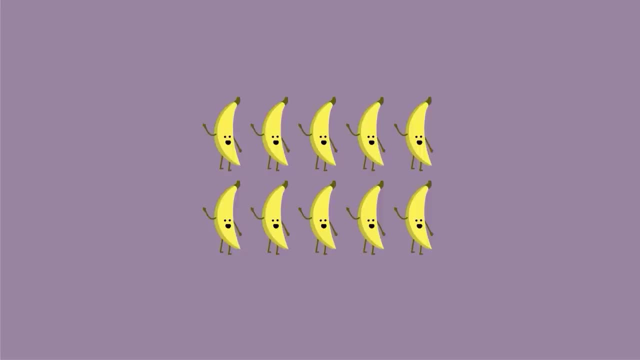 This is what 5 bananas look like And this is what 10 bananas look like. I will show you again. This is what 2 bananas look like: 1, 2.. This is what 5 bananas look like: 1,, 2,, 3,, 4,, 5.. 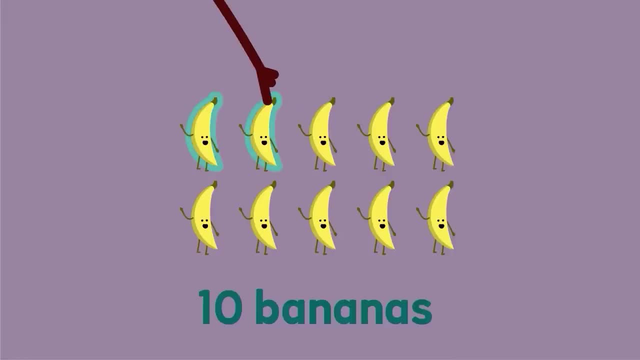 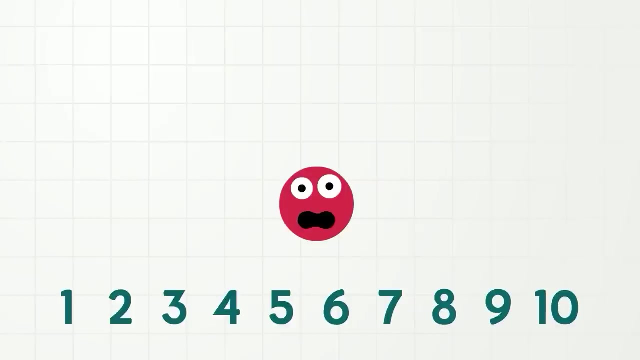 And this is what 10 bananas look like: 1,, 2., 3., 4., 5., 6., 7., 8., 9., 10.. So I am going to quickly show you some different bananas and I want you to estimate how many. 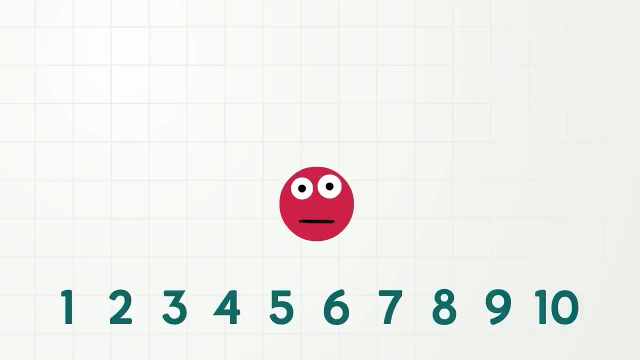 bananas you think there are And remember, because you are estimating or guessing, it is okay if you don't know the exact number of bananas. Are you ready to see some bananas? Of course you are. Yeah, Here We Go. 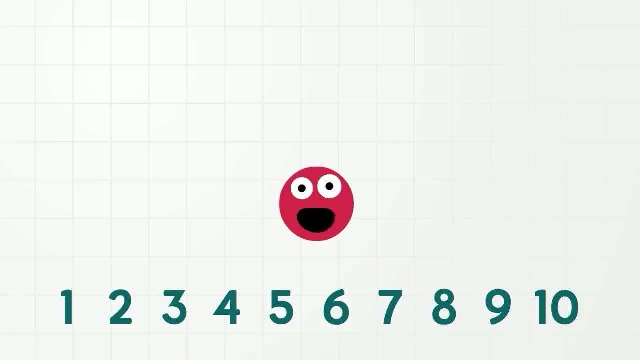 Okay, That was a pineapple, not a banana. Who put that pineapple in there? I did Sorry. Okay, Let's try again. Ready, Here We Go. So what was your estimate of how many bananas there were? 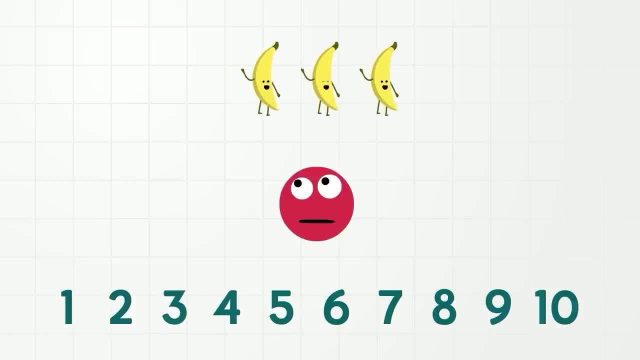 Let's count and find out. Bananas. I said bananas, 1. 2. 3. Bananas, Remember two bananas look like this. so if we add one more, we know that 2 plus 1 is 3.. 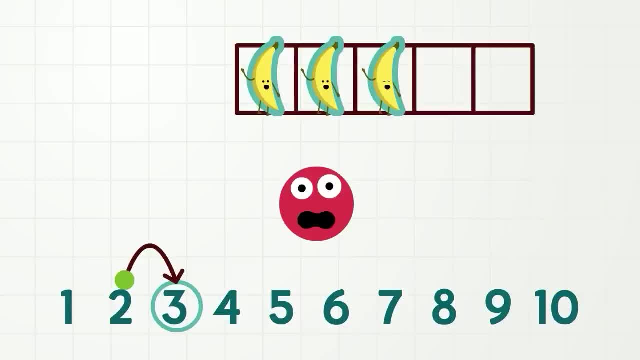 3 bananas. Bananas. Okay, You did such a good job, Let's take a quick break. Okay, That's enough. Now let us do some estimating. again with a different number of bananas Ready, Here We Go. 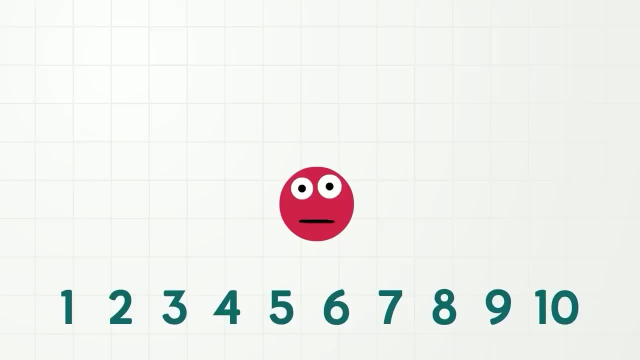 So what was your estimate of how many bananas there were? Let's try again: 1., 2., 3., 3., 4., 5. 6. Bananas, Yes, bananas, That's correct. In fact, there were seven bananas. 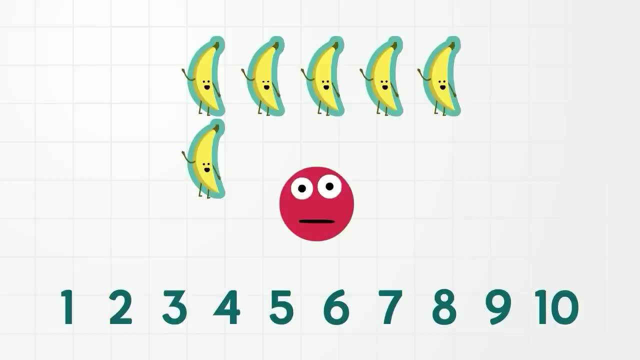 How many bananas there were. Let's count and find out: 1., 2., 3., 4., 5. 6 bananas. Remember that five bananas look like this, so if we add one more, we know that 5 plus. 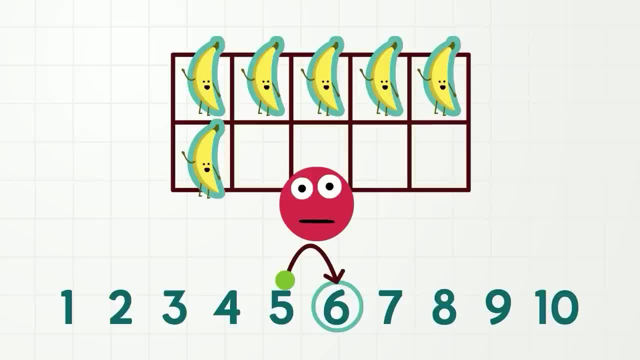 1 is 6.. 6 bananas- Bananas. If you estimated that there were six bananas, Good job. If you estimated that there were five bananas, that is right. Yes, there were five bananas. There were more bananas- Yes. 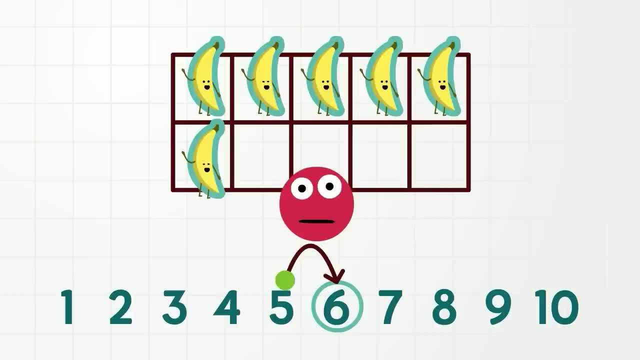 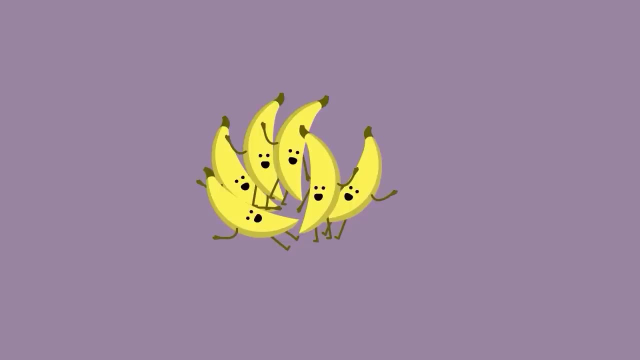 Bananas. You're right, 5 bananas, Yes, bananas. Five bananas also. good job, because five is close to six. Want to know something? Of course you do. Six bananas don't always look exactly like this. They could look like this, and there would still be six. 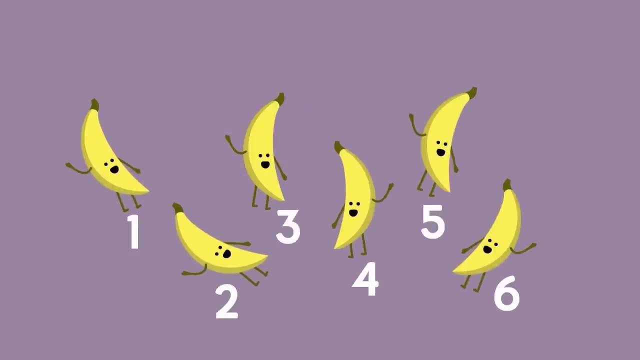 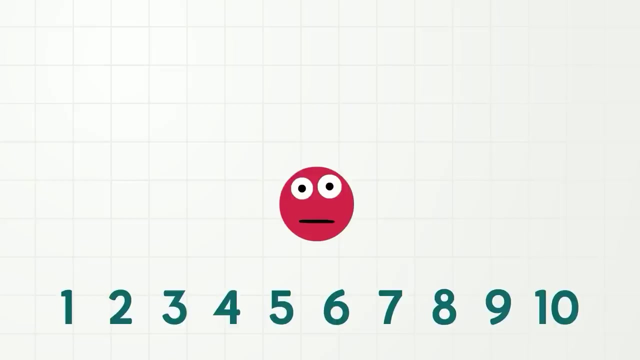 They could also look like this, and there would still be six. They could also even all have funny hats, and there would still be six. Okay, let us do some estimating. one last time, with a different number of bananas Ready. Here we go. 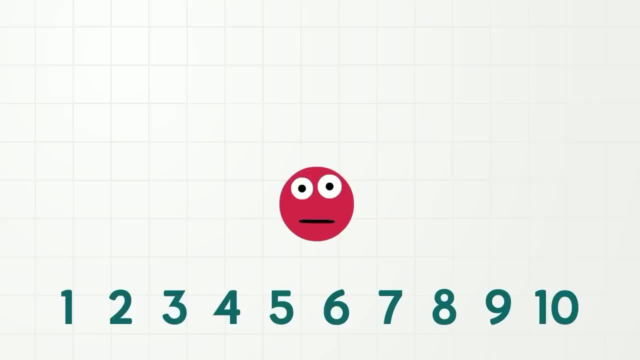 So what was your estimate of how many bananas there were? Let's count to find out: One, two, three, four, five, six, seven, eight bananas. Remember that five bananas look like this: So if we add three more, we know that five plus three is eight. 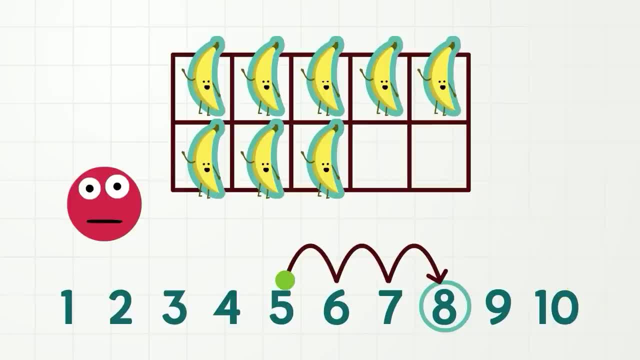 Eight bananas- Bananas, But maybe you estimated a different number and that's okay. For example, remember that ten bananas look like this: So if you take away two bananas, we know that ten minus two is eight Eight bananas. 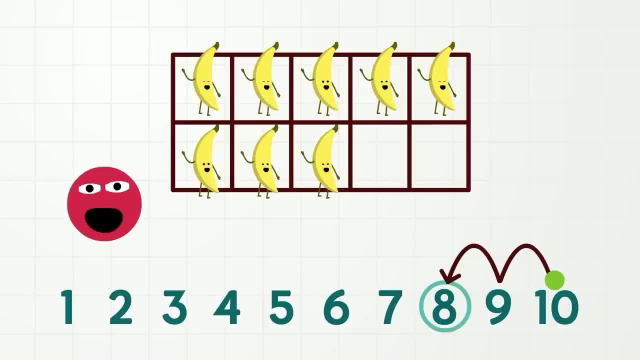 Bananas. If you estimated that there were eight bananas, good job. If you estimated that there were five or ten bananas, also good job, because five is kind of close to eight and ten is also close to eight too If you estimated that there were 100 bajillion triple bananas. 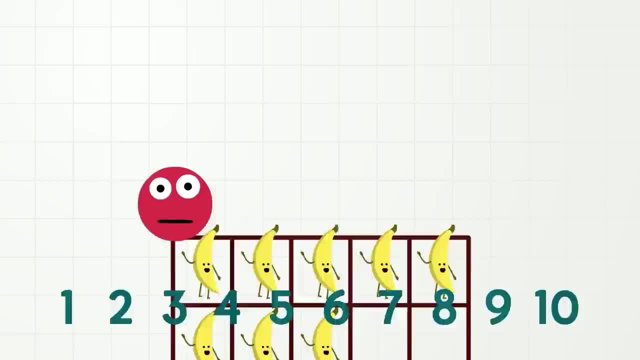 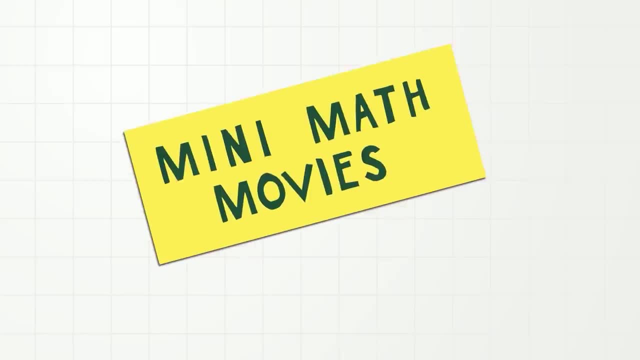 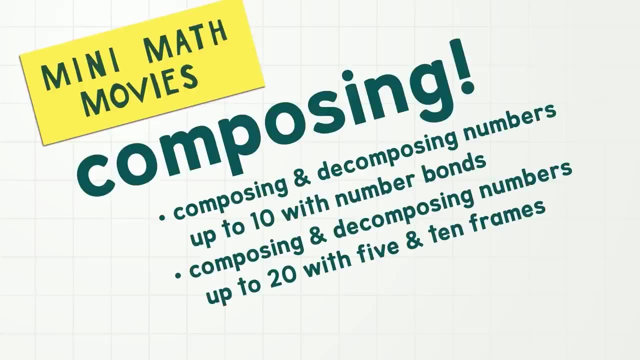 that is not so good, because that is not even a real number. Okay, that is all the time we have today for estimating. If you have any questions, feel free to ask them in the comments and we will answer them in the next video. 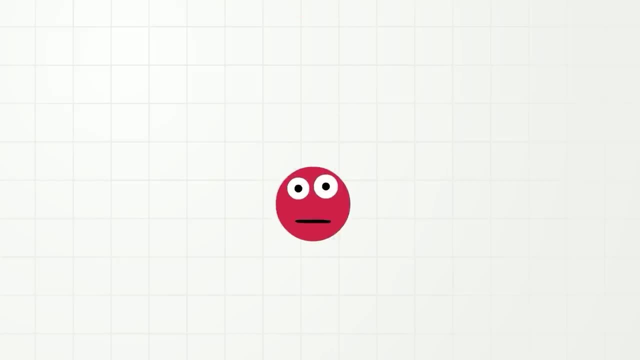 Oh, hi everybody. Today I'm going to talk to you about numbers and composing and decomposing numbers, and maybe even apples- Oh, I really like apples. So composing is a large word, Composing- And it's what happens when little numbers come together to make a bigger number. 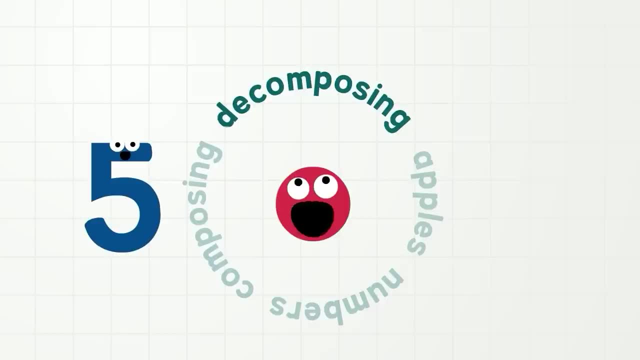 And decomposing is an even larger word, Decomposing- And that is what happens when a bigger number is taken apart into little numbers. And there are many, many, many different ways to put numbers together and take them apart. I will show you with an example. 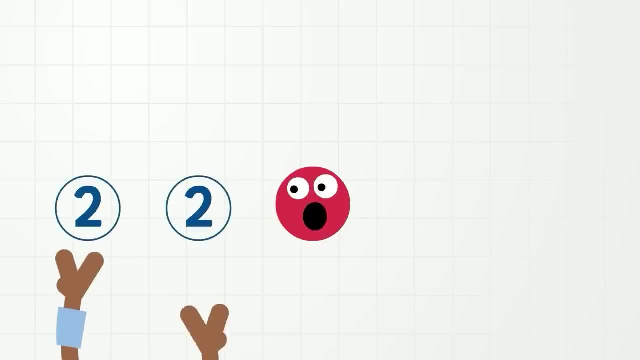 Here we have the number two and there is another number two. What happens if you put two and two together? That's right, you get four, Four. This two and this two came together and made the number four. So four is made up of two and two, which means four can be taken apart into two and two. 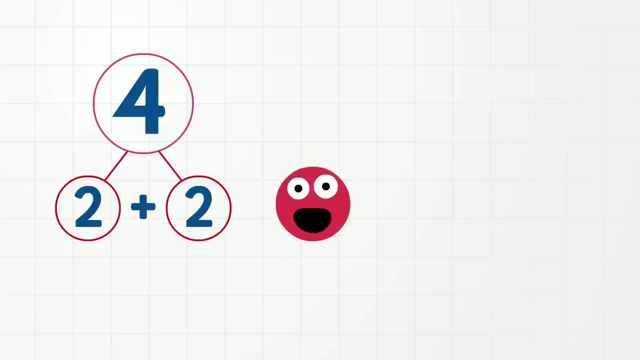 Wow, We can put together and take apart the number four with totally different numbers. No, it's true. Watch, Here we have the number three and there we have the number one. What happens? What happens if you put three and one together? 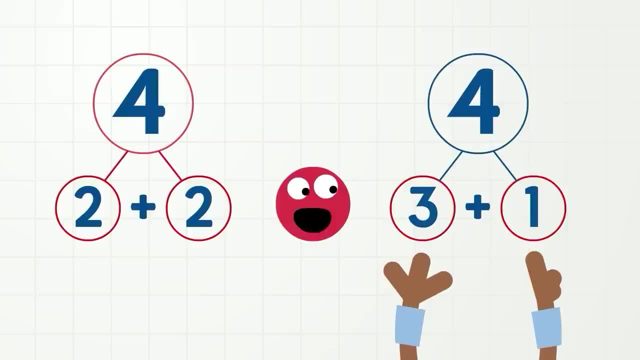 That's right, you get four, Four. The three and the one came together and made the number four. So four is made up of three and one, which means that four can be taken apart into three and one. Wow, So there are at least two different ways to put together and to take apart the number. 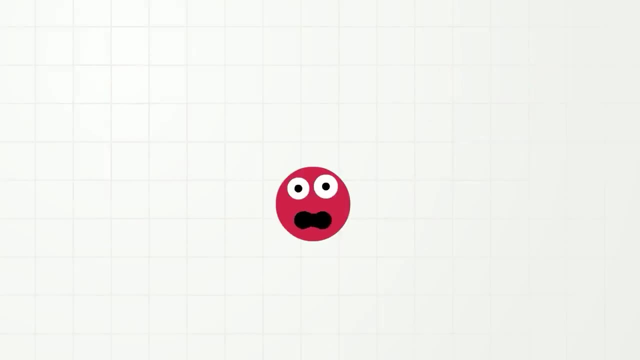 four: OK, you are doing such a good job listening, you can now watch a movie. OK, that's enough. This may be easier to explain if we have something to help us. Ah, I know, apples. I said apples. 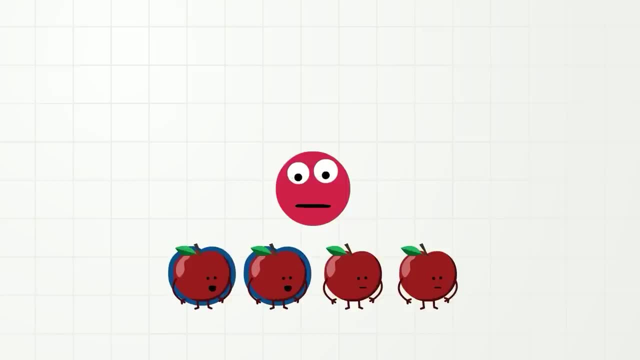 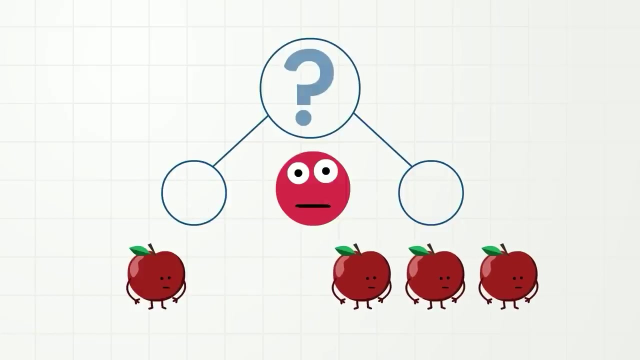 OK, look, we have one, two, three, four apples And we can take them apart or they can move. so we have two apples here and two apples there, But we still have four apples. And what happens if one apple moves? 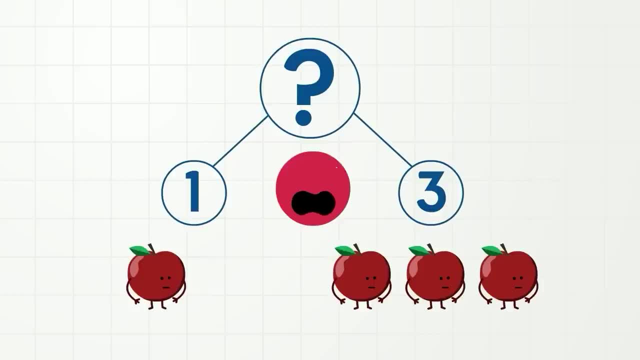 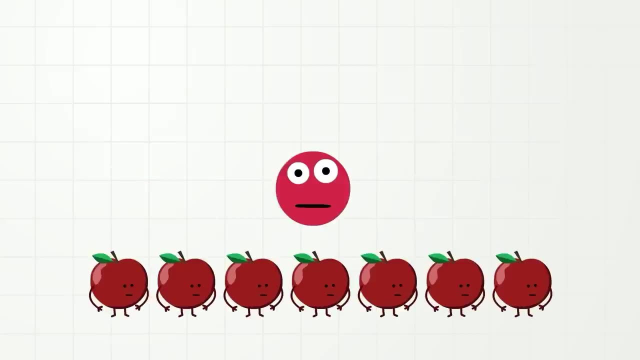 Well then, we have one apple here and three apples there, but we still have four apples, Apples. OK, let us start again with some more apples. Now we have one, two, three, four, five, six, seven apples. 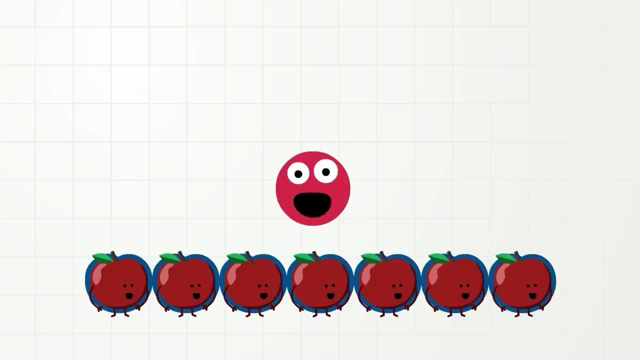 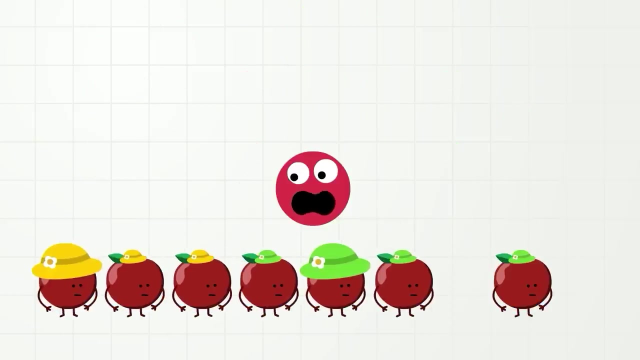 Apples. Let's see how we can take apart and put together these seven apples. Maybe we should use something to help us organize them. Hmm, Oh, I know How about funny hats? Ha, Now let's have all of the apples with yellow hats go over here and all of the apples with 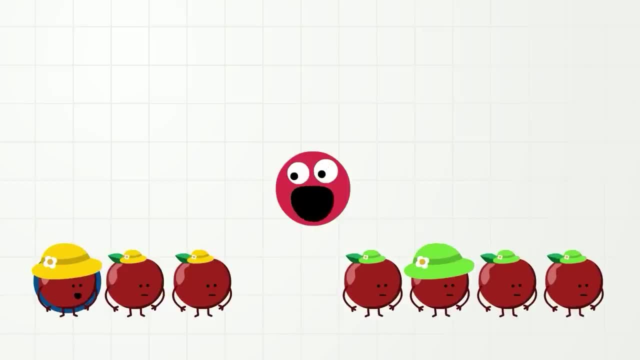 green hats go over there. So now we have one, two, three apples with yellow hats and one, two, three, four apples with green hats. Add them together and we have seven apples. So the numbers three and four make the number seven. 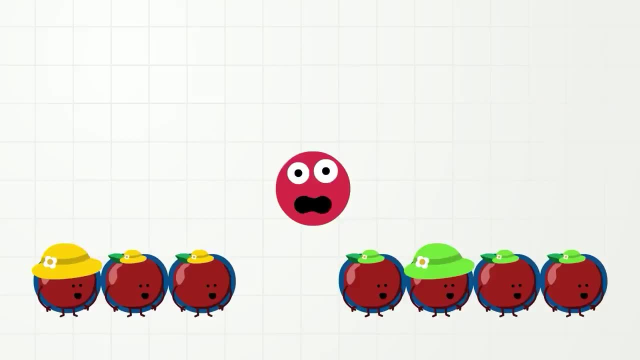 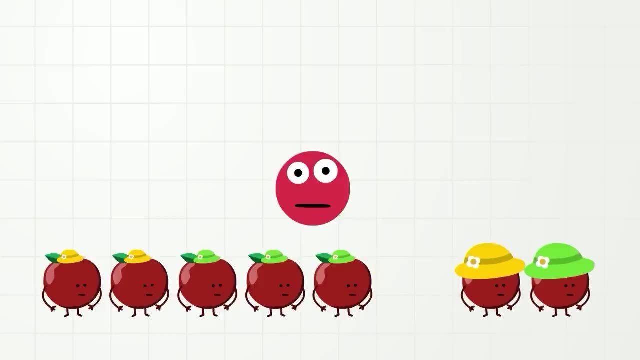 Seven. Now let's have all of the apples with little hats go here and all of the apples with big hats go over there. So now we have one, two, three, four, five apples with little hats and one, two apples. 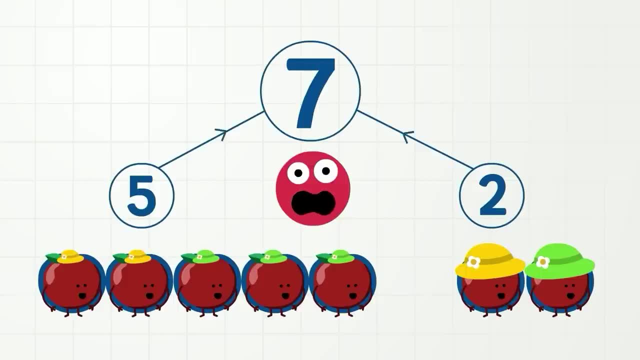 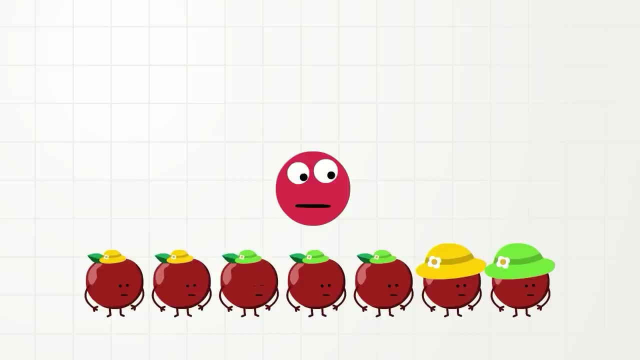 with big hats. Add them together and we have seven apples. OK, So the numbers five and two also make the number seven. Wow, Seven. OK, One more. How about all of the apples that have a bite out of them go over here and all of the what's? 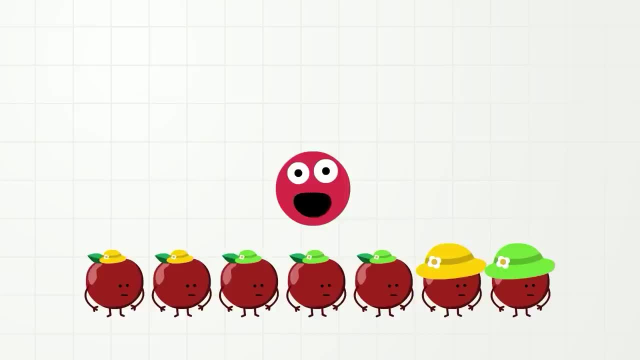 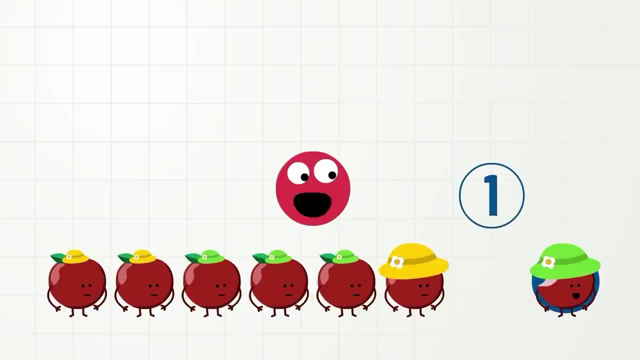 that None of the apples have a bite. Oh well, we have to fix that. As I was saying, all of the apples with bites go over here and all of the apples without bites go over there. So now we have One apple with a bite and one, two, three, four, five, six apples with no bites. 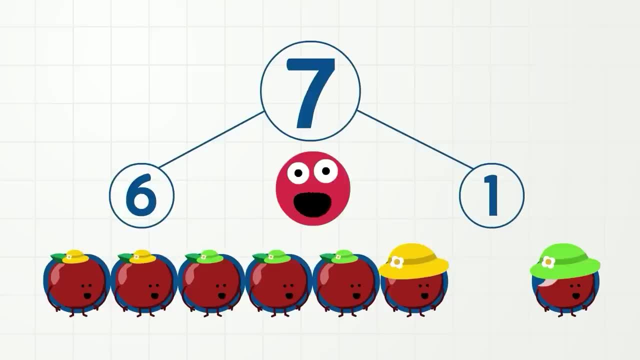 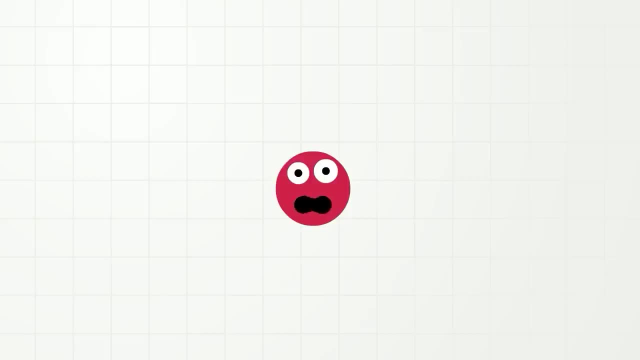 Add them together and we have seven apples. So the numbers one and six also make the number seven Seven. OK, Let's take a break and watch a movie. OK, that's enough. Last one with even more apples, but this time no funny hats. 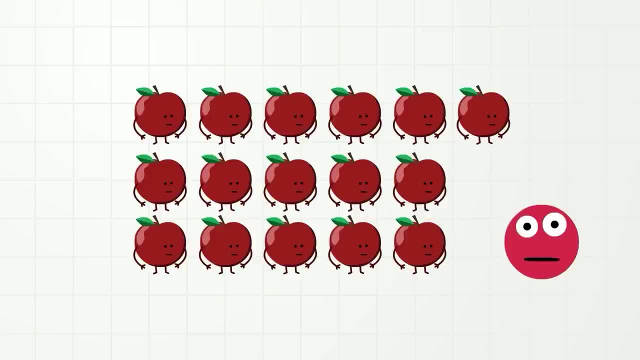 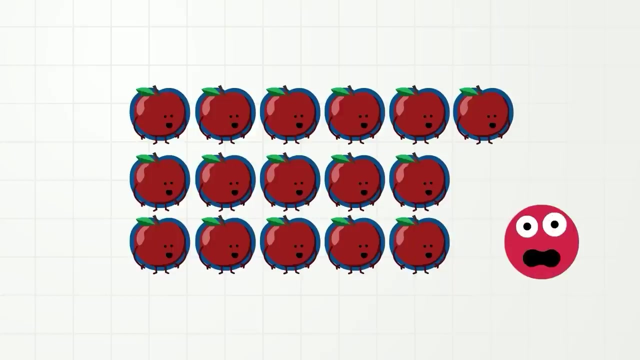 Wow, so many apples. How many? Let's count: One, two, three, four, five, six, seven, eight, nine, ten, eleven, twelve, thirteen, fourteen, fifteen, sixteen apples, And there are many, many, many ways to compose or put together sixteen apples. 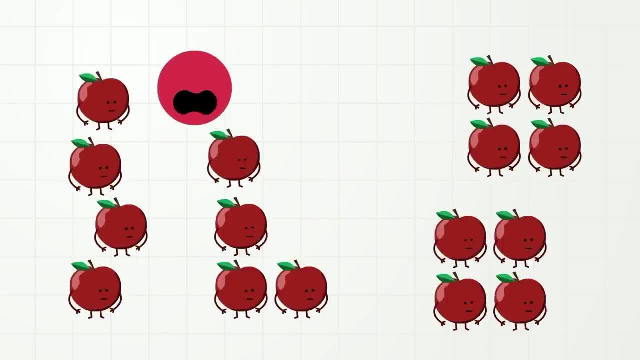 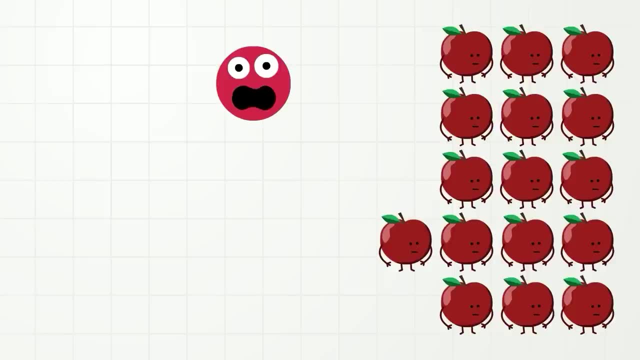 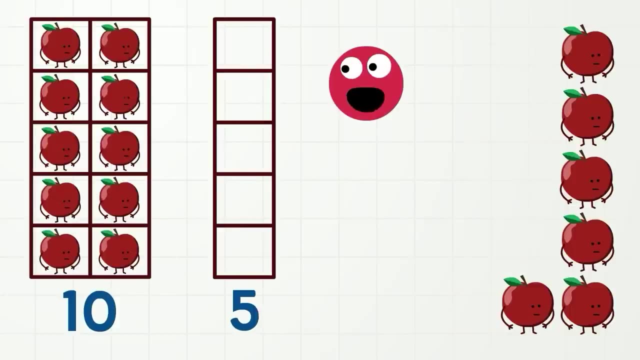 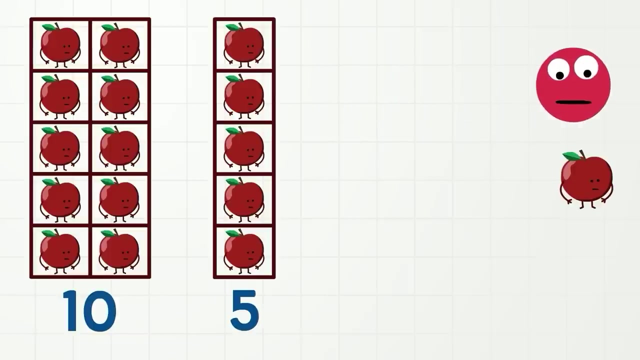 OK, OK, apples. and also to decompose or take apart the 16 apples. Let's try some. Sometimes, when we are thinking about numbers, it can be easier to think about the numbers 10 and 5.. So if 10 apples go here and 5 apples go there, how many apples do we have left? 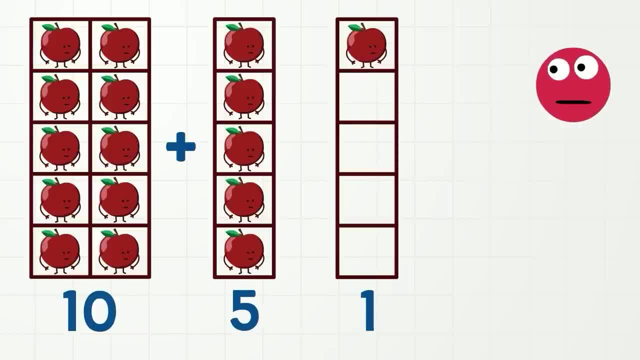 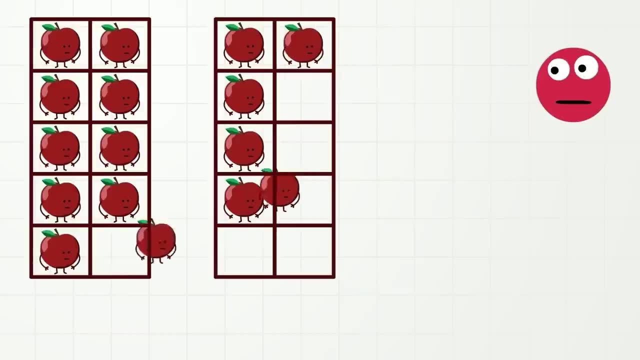 That's right. 1, 10, plus 5, plus 1 is 16!. So the number 16 can be made up of the numbers 10 and 5 and 1.. Cool, Let's try again. apples move. 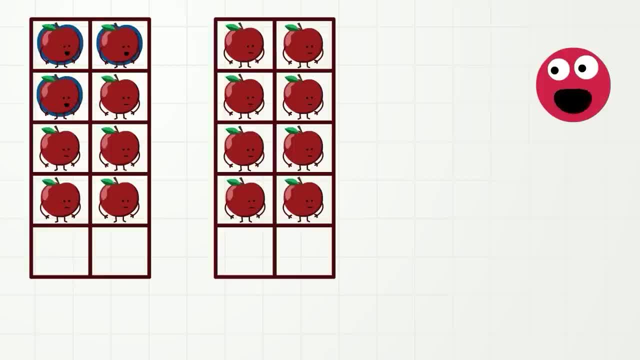 Oh, wow. now we have 1,, 2,, 3,, 4,, 5,, 6,, 7,, 8 apples over here And the same number of apples over there. 8 plus 8 is 16!. 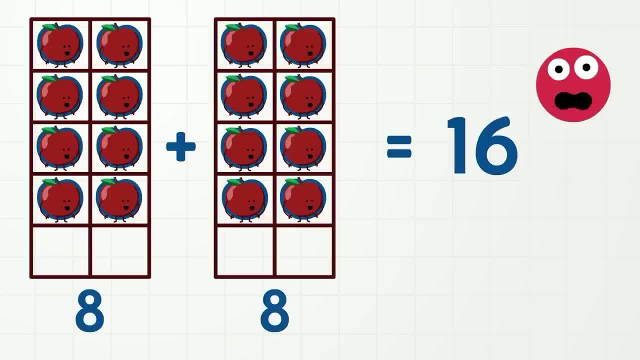 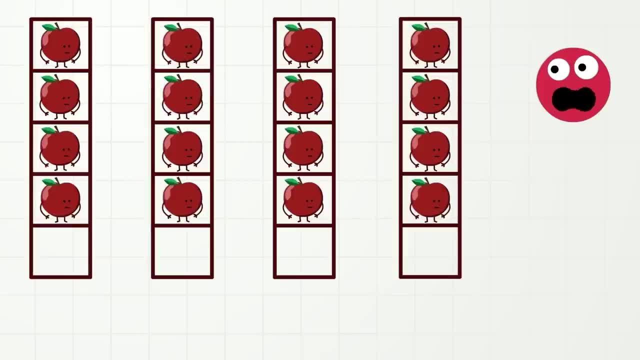 So the number 16 can also be made up of the numbers 8 and 8.. OK, one last time. move apples. Oh cool, Now we have 1,2,3,4, apples here and the same number 4 apples here and the. 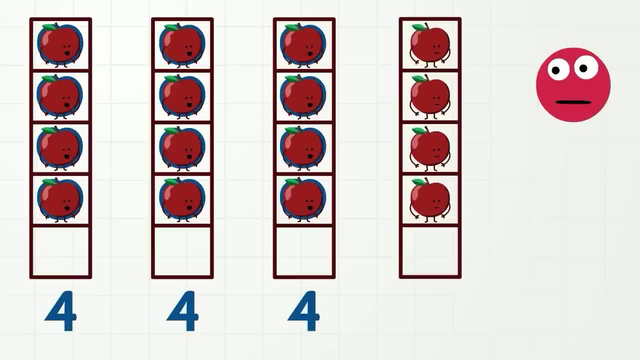 same number: 4 apples over here. same number: four apples here and the same number: four apples here. Four groups of four. Four plus four plus four plus four is sixteen. So the number sixteen can also be made up of the numbers four. 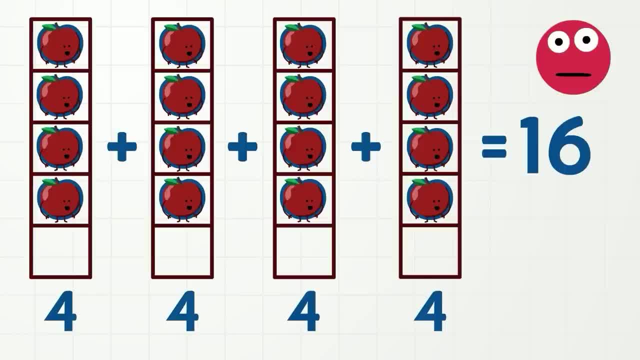 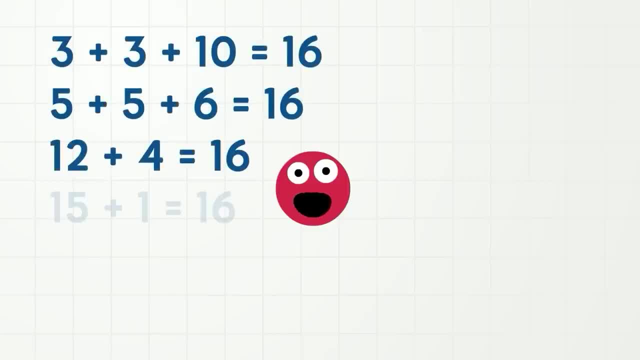 four, four and four, And guess what? You can also make up and take apart the number sixteen with other numbers that we haven't even practiced yet. No, it's true. Okay, that is all the time we have today for composing and decomposing. 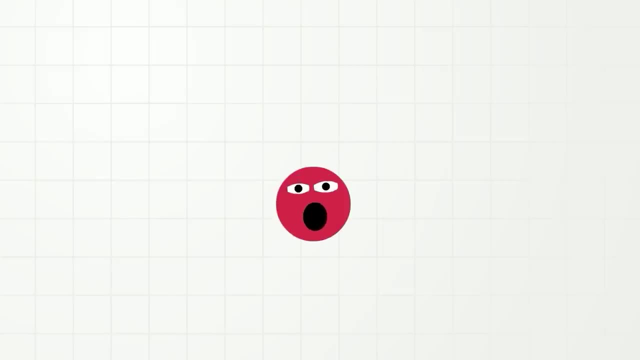 Oh hi, everybody. Today I am going to talk to you about numbers and I'm going to show you how to write them. So let's get started. Oh hi, everybody. Today I am going to talk to you about numbers and I'm going to show you how to write. 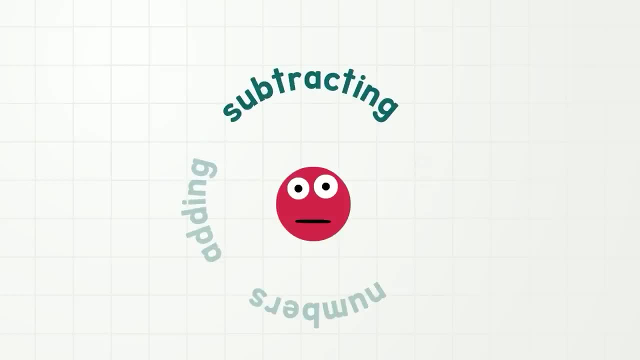 numbers and I'm going to show you how to write numbers. and I'm going to show you how to write adding and subtracting numbers, and maybe even doughnuts- I really like doughnuts. So we all know that numbers can be joined together to make bigger numbers. We call this. 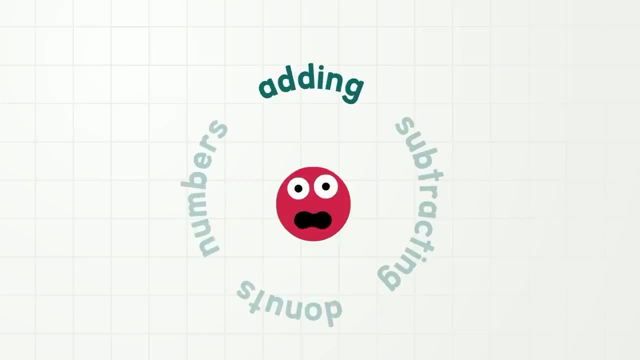 adding, And we also know that we can take away numbers from bigger numbers to make smaller numbers. We call this subtracting. Let us use an example. We need a volunteer. How about sloth? It says sloth, Okay, here is a sloth And we see that sloth has two doughnuts. 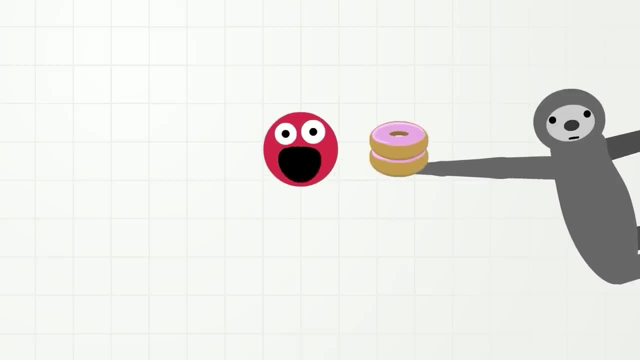 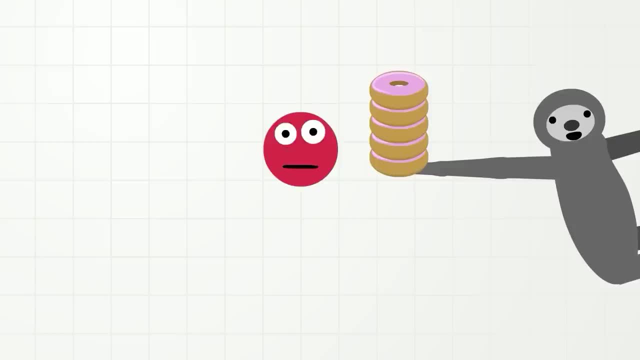 three, two and three together, we get fivefive doughnuts. Now what happens if we subtract one? Now what happens if we subtract one, two, three, four doughnuts from sloth- Yes, that's right. four doughnuts from sloth- Yes, that's right. 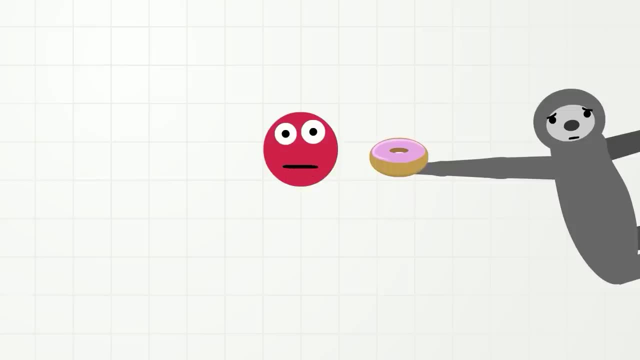 sloth gets sadder. But also mathematically, if we add five and subtract four. if we add five and subtract four, we only have one left: One doughnut. Wow, you did, such a guest, Such a good job adding and subtracting. it's now playtime. 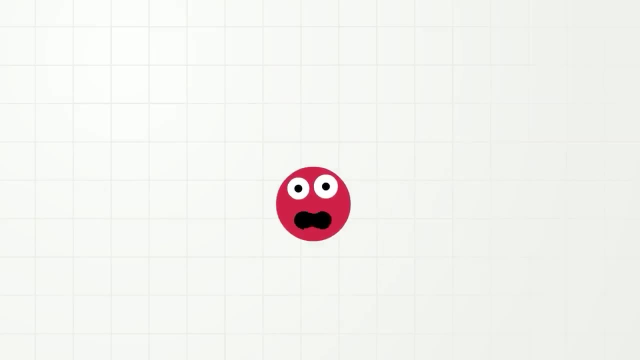 Ok, that's enough. So we can add and subtract with donuts. but did you know that we can also add and subtract with writing? No, it's true, We can do it by writing the numbers or numerals and also by writing with signs. 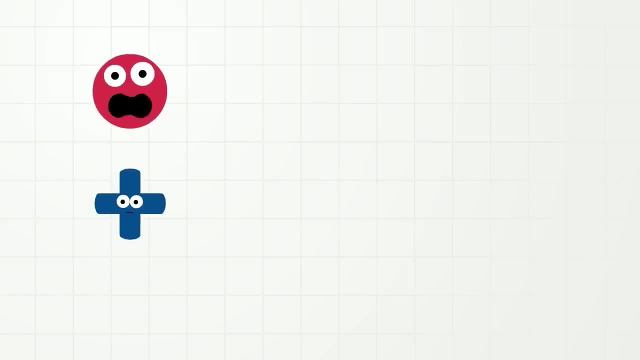 This is a plus sign, This is a minus sign And this is an equal sign. And this is a monkey riding a unicycle sign. but we never used that one in math. Please go away. monkey riding a unicycle sign. Ok, great. 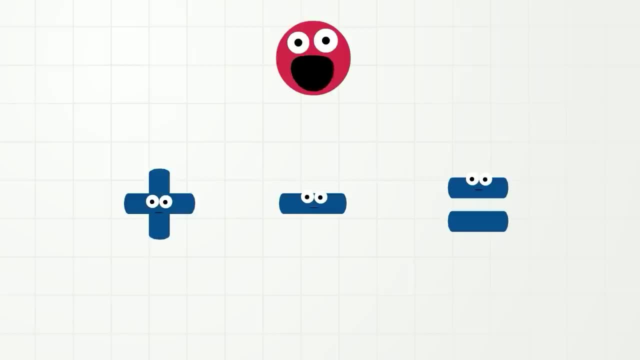 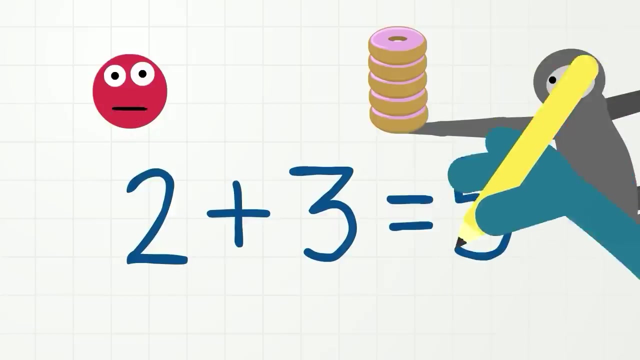 So let's add and subtract the same number of donuts with sloth, but this time also write the numbers and the signs. Ready, Of course, you are Ok. Sloth, Sloth. Finally, First, the adding Two donuts plus three donuts equals five donuts. 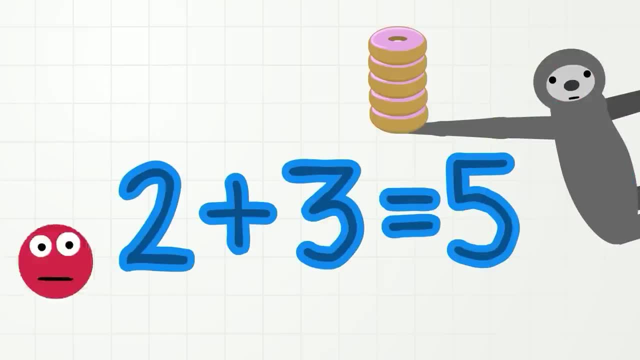 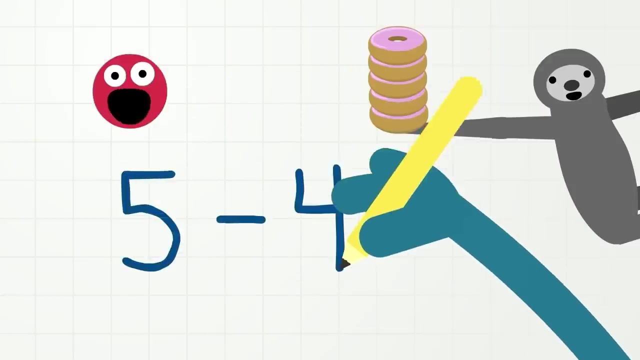 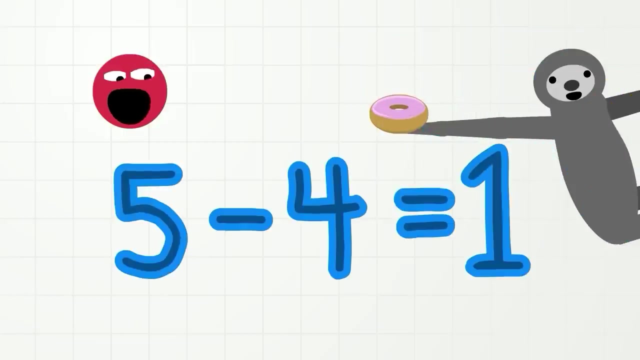 Two plus three equals five. Two plus sign three equals sign five. Happy sloth. Now, subtracting Five doughnuts minus four doughnuts equals one doughnut. Five minus four equals one. Five minus sign four equals sign one. Sad sloth. 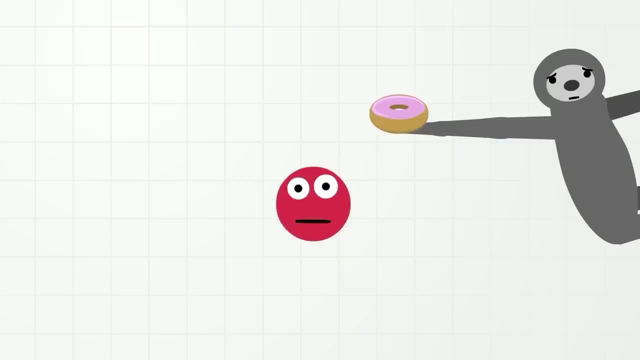 OK, let's do another one, but with some different numbers and different doughnuts, Oh, purple. So let's see, We have one, two, three, four doughnuts and we add one, two, three, four, five doughnuts. 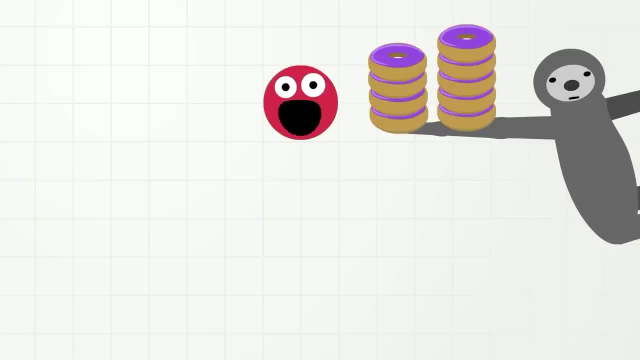 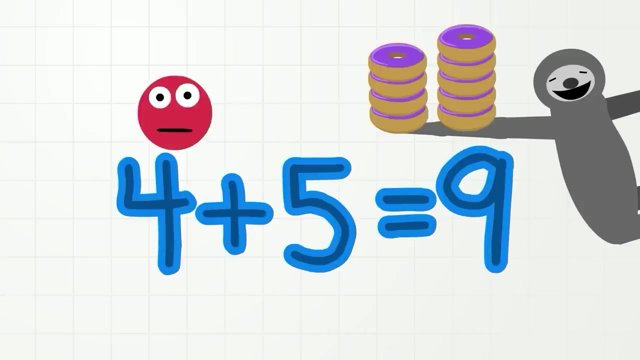 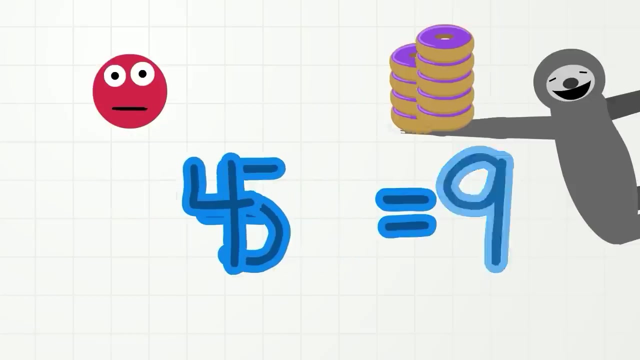 So we have anybody know, That's right. nine doughnuts. Four plus five equals nine. Four plus sign five equals sign nine. Super happy sloth. So I have a question: What do you think happens if we switch the four and the five like this: 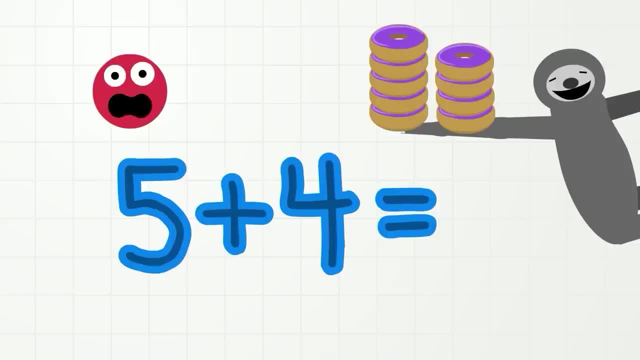 Now, how many doughnuts do we have? That's right, the same number of doughnuts: nine doughnuts. So four plus five equals nine, and five plus four also equals nine. Four plus five equals nine, and five plus four equals nine. 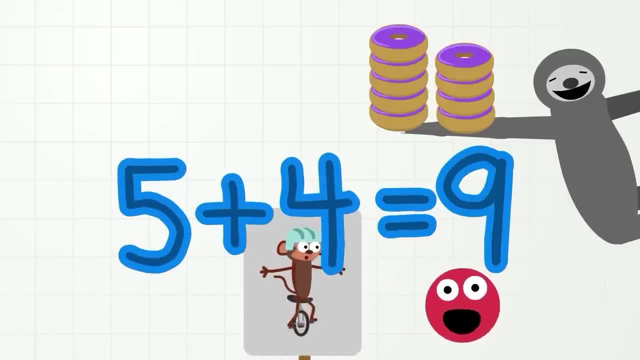 Everybody. four plus five equals nine, and five plus four equals nine. Happy sloth. Four plus five equals nine, and five plus four equals nine. OK, that's enough. Hey, you want to know something? Of course you do. 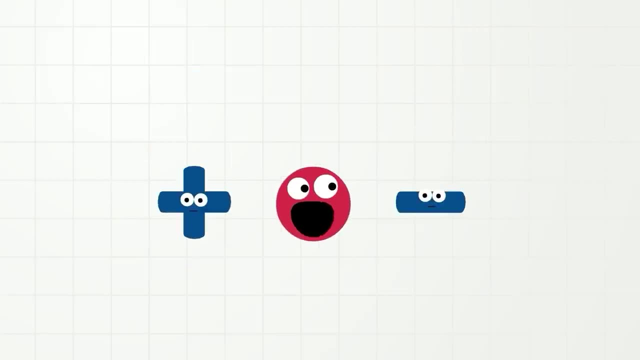 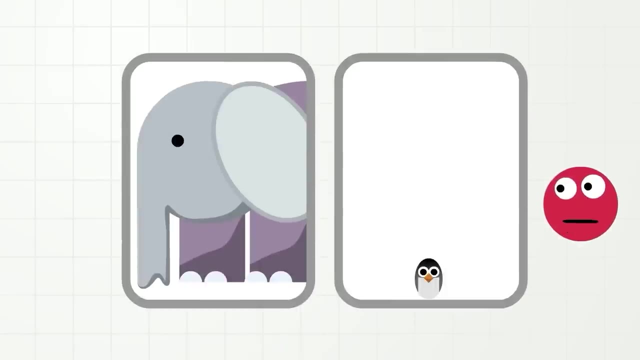 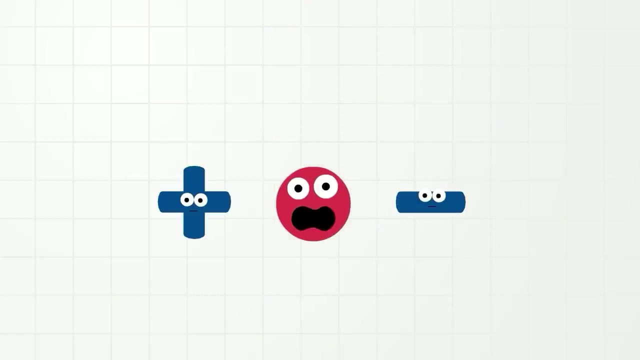 The plus sign and the minus sign are kind of like opposites, You know opposites, Just like happy and sad, Big and small, And daytime and nighttime, Opposites, Opposites. And we can use the plus sign and the minus sign in opposite ways with the same numbers. 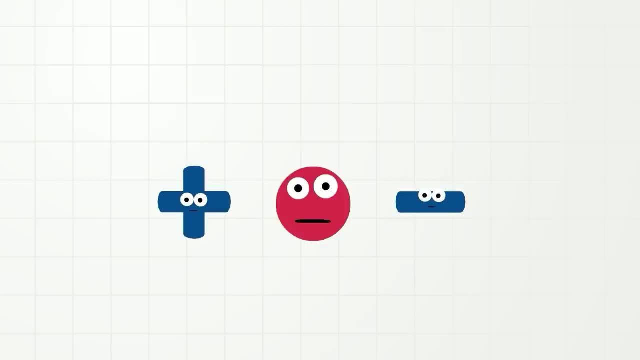 to check if our math is correct. No, really watch. If five plus four is equal to nine, then nine minus four is equal to five. Same numbers, different order and different signs, But both are correct. Five plus four equals nine. 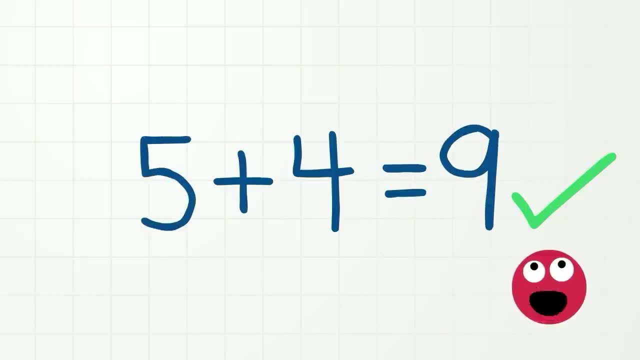 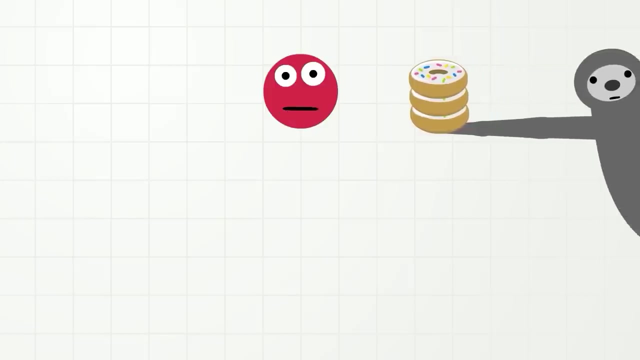 Correct. Nine minus four equals five- Correct. Five plus four equals nine- Correct. Nine minus four equals five Correct. Five plus four equals nine. Correct. Nine minus four equals five Correct. OK, that's enough. OK, let's do one last example of adding, but with some different numbers and different. 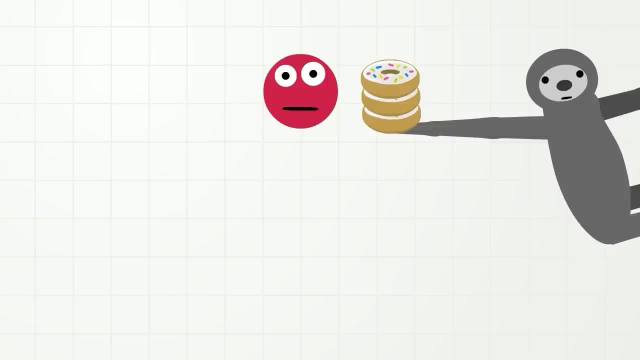 donuts. Oh, sprinkles, Wow. So this one may be a little tricky. We have one, two, three donuts and we add: uh, no more donuts. So now we have- anybody know That's right- three donuts. 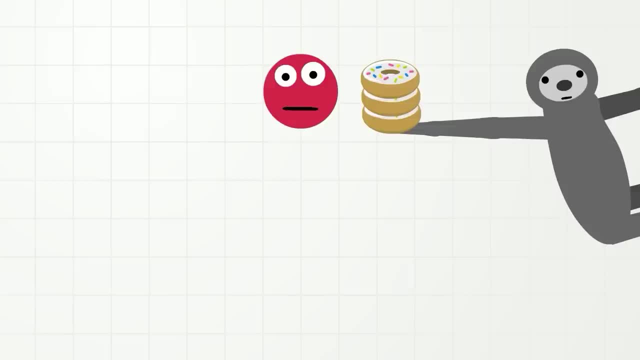 Do you know what is the number we use when we don't have anything? That's right. Zero, Zero, Yeah, So that means three plus zero equals three, Three, Three. And what if we had four donuts and we added zero? 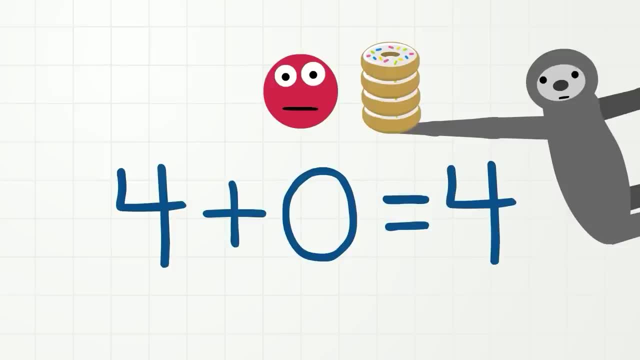 That's right. Four plus zero equals four, And so even if you had a really, really, really high number of donuts, like seventeen, and added zero, you would still have seventeen donuts. Yay, OK, you did such a good job adding zero. 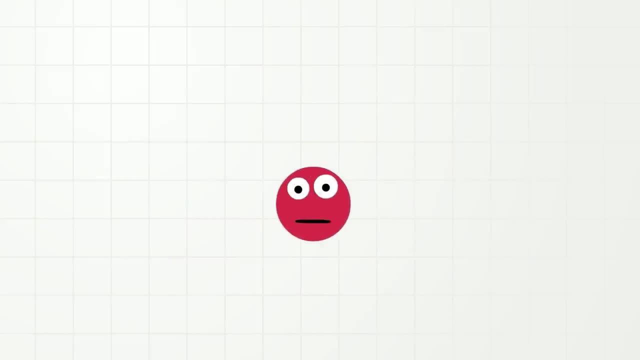 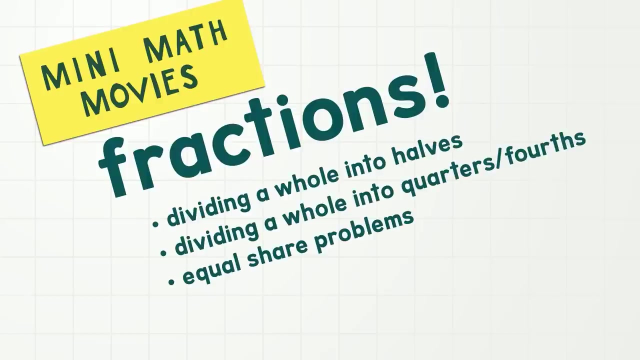 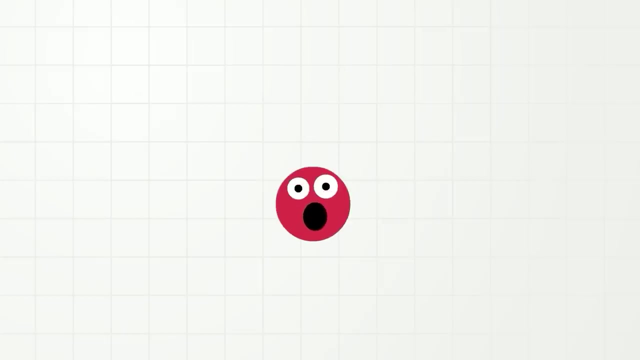 It is now play time. OK, that's enough. That is all the time we have today for adding and subtracting. Oh, hi everybody. Today I am going to talk to you about numbers and fractions, and maybe even Kevin. Huh, I really like Kevin. 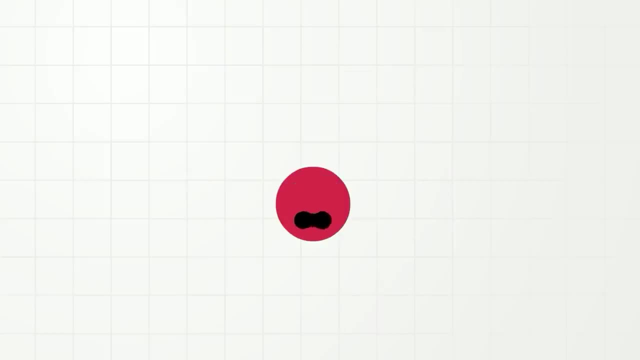 OK, So we all know how to count things right? Yes, of course you do, But do you know how to count parts of things? I will show you. First, we need something that we can count and also divide into equal parts. 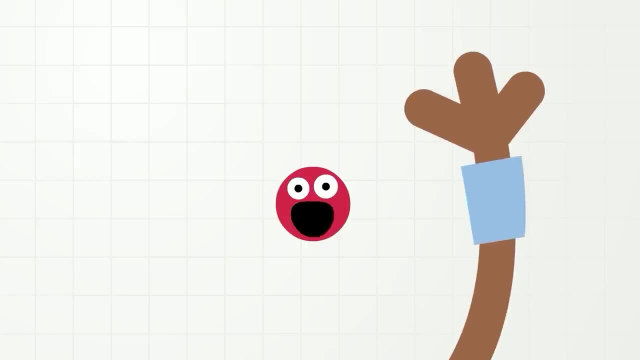 Uh, how about a pizza? Oh, no, not another pizza example. Hmm, we need something else. How about me? Oh, good idea. OK, Now how many me's do you see? That's right, There are one, two, three me's. 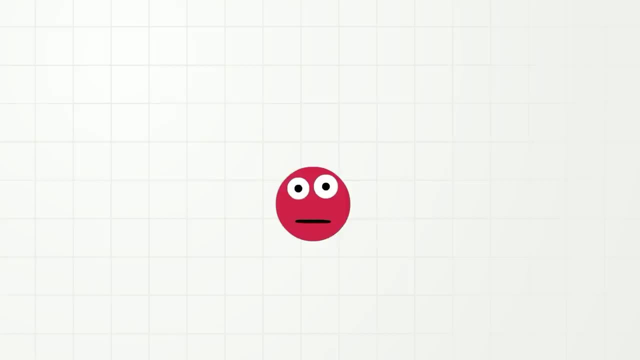 And now, how many me's do you see? Yes, there is just one me, One whole me. Yay, But now watch closely. But don't worry, I am a cartoon, so it won't hurt. How many me's do you see? 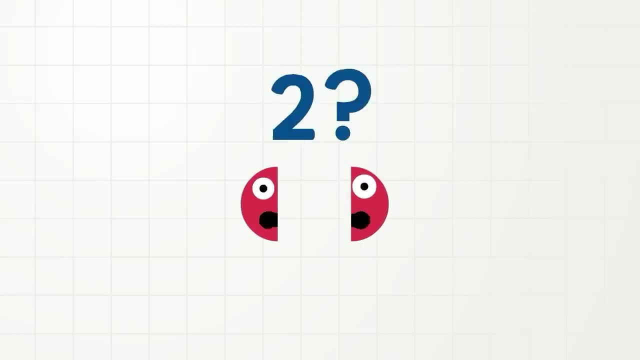 How many me's do you see? Are there two me's? No, not really. There are two parts of me, or two equal halves of me, One half here and one half here, And when we put one half and one half together, there is one whole me. 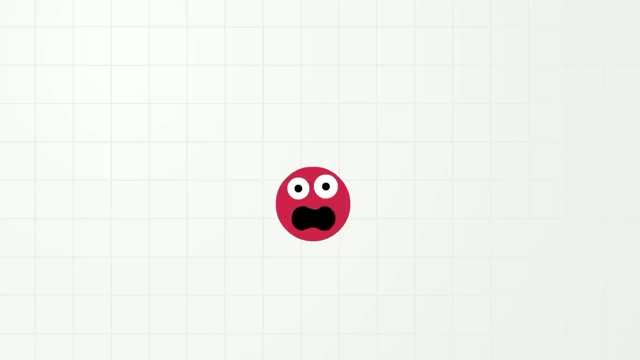 So in math, when we have parts of whole things like this, we can call these parts fractions, Fractions. OK, you did such a good job listening. it is now time to sing a song. OK, that's enough. So, as I just showed you, if I divide myself into two equal parts, then I have two halves. 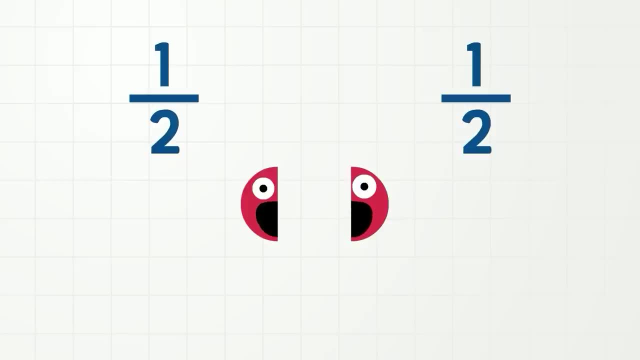 But what happens if these halves also get divided into halves? OK, watch, And don't worry, I am a cartoon, so it won't hurt. So now are there four of me? No, not really, but there are four equal parts of me. 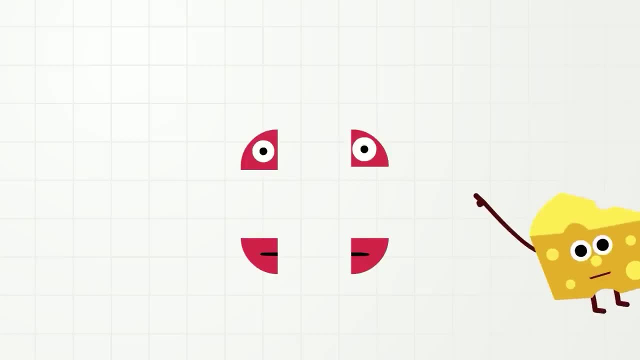 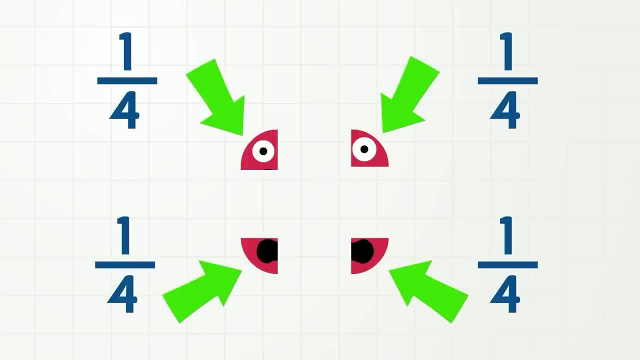 One quarter here, one quarter here and one quarter here, And if we put four quarters or four fourths of me together, there is one whole me. OK, let's review, because it might be a little confusing. Uh-oh, where did I go? 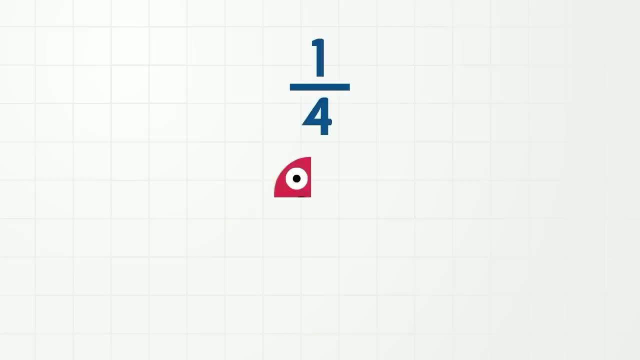 Don't worry. So this is one fourth of me, or one quarter. This is two fourths of me, or two quarters, And two fourths is also the same as one half, One half. This is three fourths of me, or three quarters. 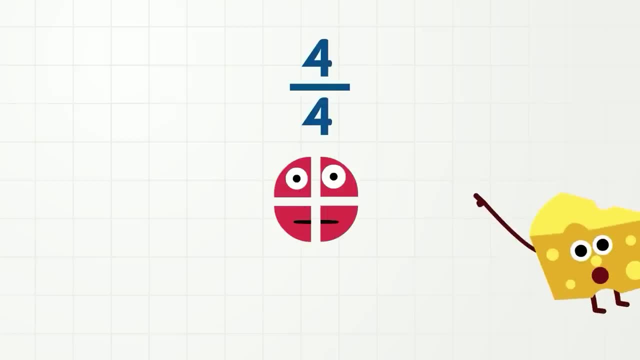 And this is four fourths of me, or four quarters, And four fourths is the same as one whole, One whole. Phew, you did such a good job listening. it is now time to sing a song. OK, that's enough. 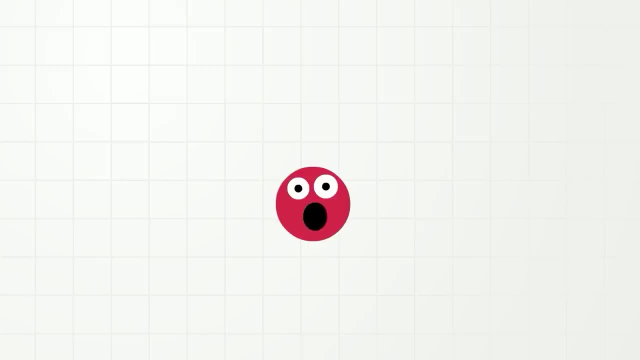 Let's talk about something else besides me. Do you know when is another good time to use fractions? When we are sharing something, Especially if we want to share something fairly and give everybody the same amount? Let's use something to help us explain. 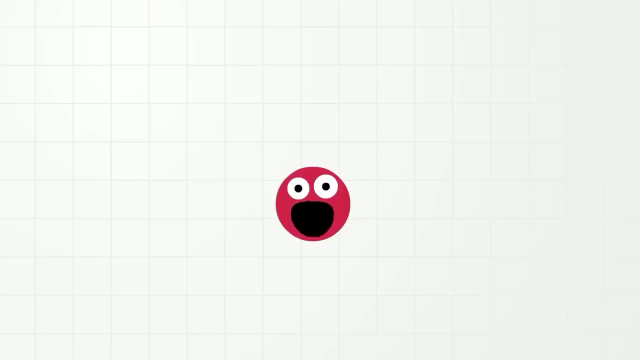 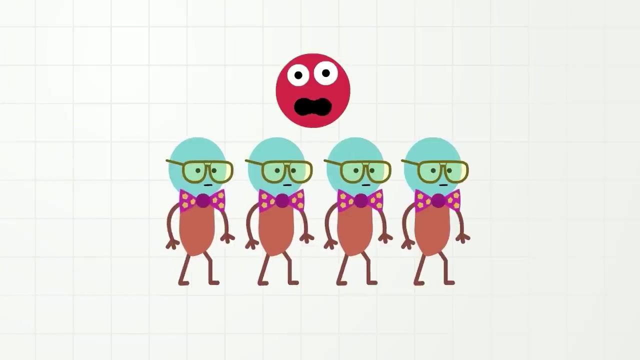 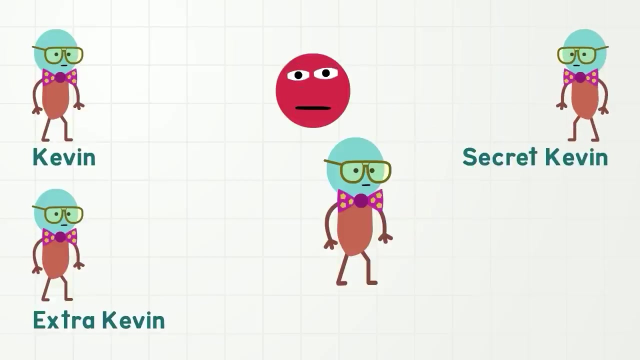 What can we use? Oh, I know How. about Kevin? I said Kevin. No, I want all the Kevins. OK, here we have four Kevins: Kevin, Extra Kevin, Secret Kevin and Funnest Kevin. 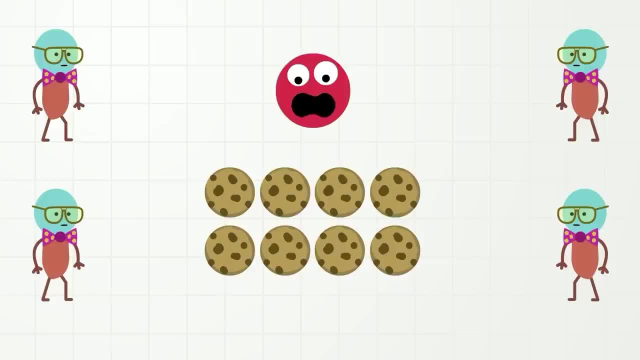 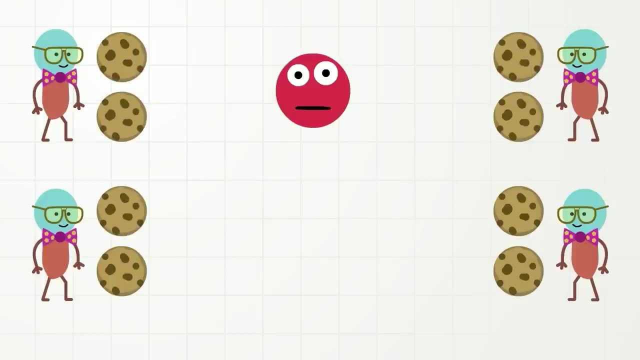 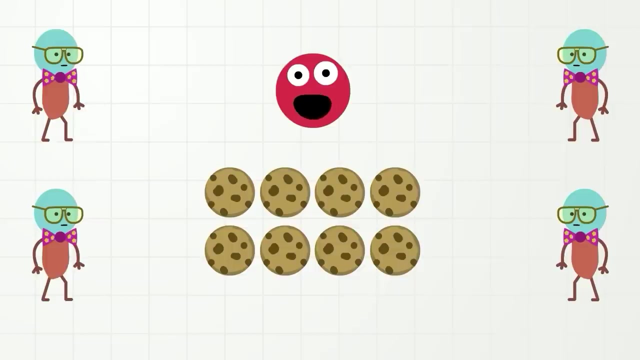 What if we have eight cookies and we want to share these cookies fairly to all the Kevins? Let's try Move cookies. OK, now each Kevin has the same number. One, two cookies. Come back cookies. Now what happens if two of these cookies disappear? 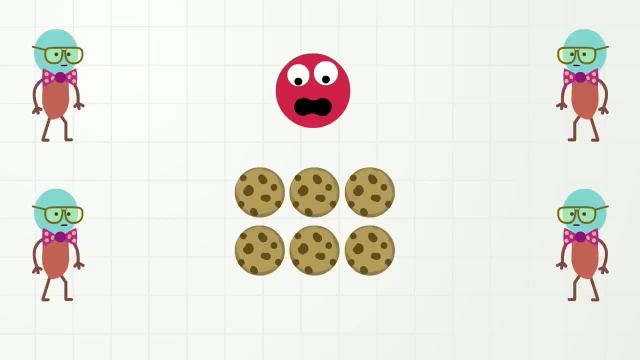 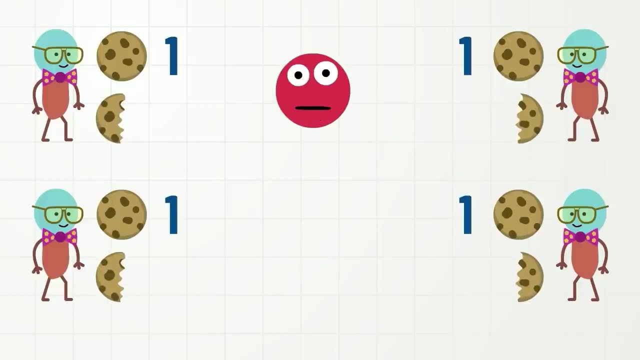 Well, that means we only have six cookies left. Let's try and share them Now. each Kevin has one cookie, but there are two cookies left. How can we share them fairly? It looks like we're going to have to make some fractions and break the cookies in half. 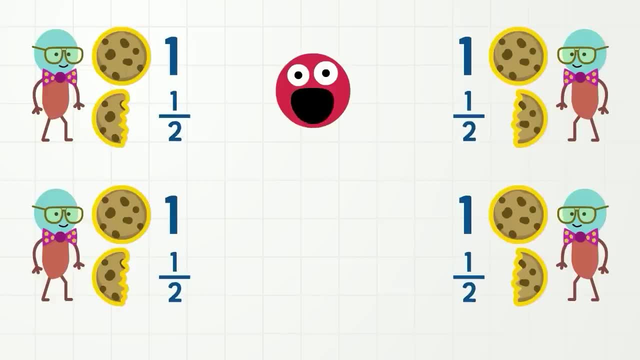 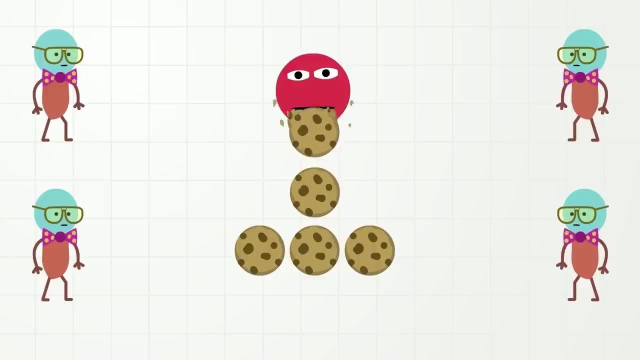 Now each Kevin has one cookie and one half of a cookie. One and one half cookies each. OK, come back cookies. OK, now what happens if um five more of the cookies disappear? Well, that means we only have one cookie left. 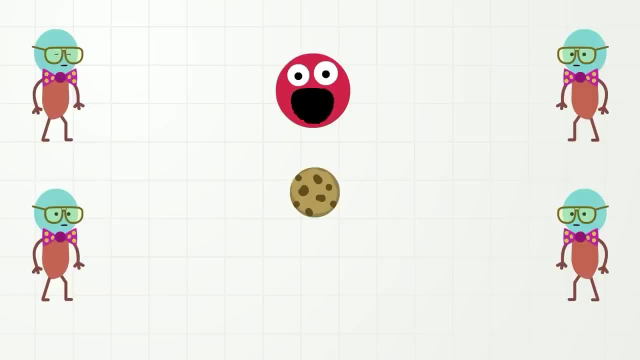 Let's try and share them. Hey, how can we share one cookie fairly? It looks like we're going to have to make some fractions and break the cookie into quarters. Now each Kevin has one fourth or one quarter of a cookie. 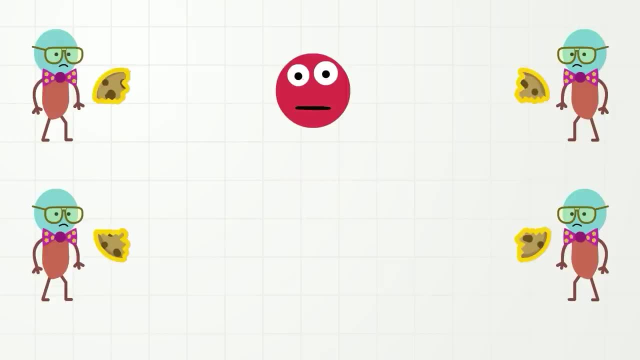 Don't be sad, Kevin. We're going to have to make some fractions and break the cookie into quarters. Don't be sad, Kevins. You got one quarter of a cookie, OK, that is all the time today we have for fractions. 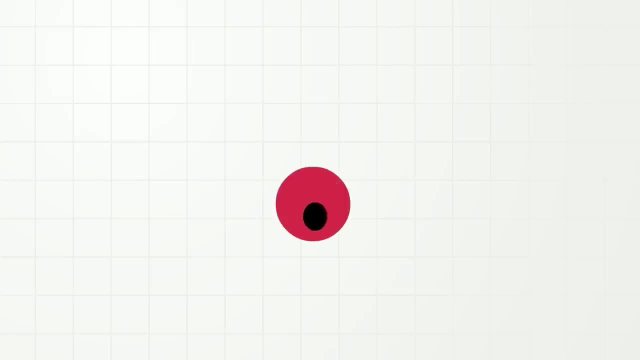 Oh, hi everybody. Today I am going to talk to you about numbers And measuring, And maybe even salamanders. Oh, I really like salamanders. So one thing we use numbers for is when we are measuring, Measuring. 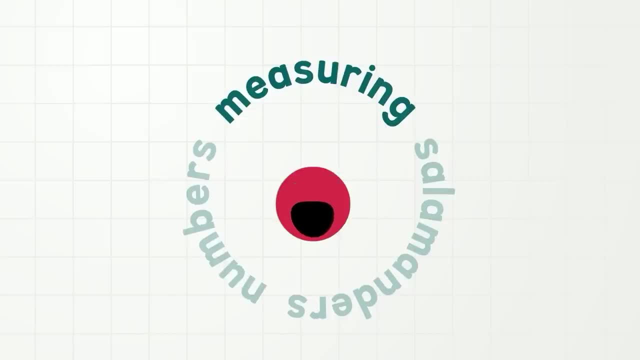 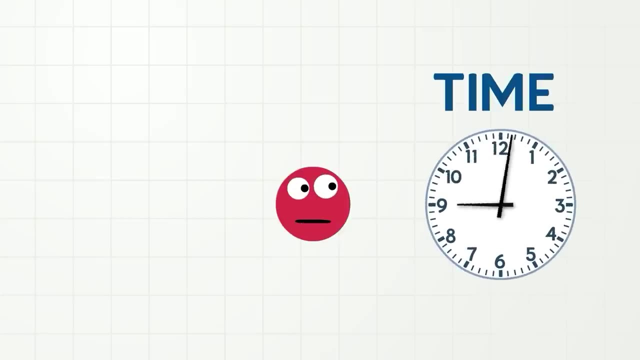 Measuring is finding out the size of something or the amount of something, And we can measure many things like time, weight, temperature or even speed. But today we are going to measure length- Length- Length is the distance between two points. 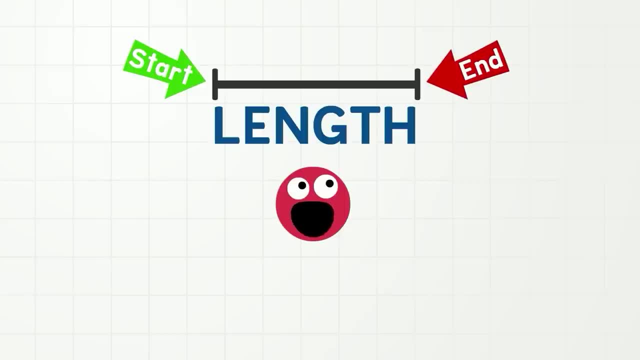 Like how far it is between the start and the end of something, And we measure length to find out how long something is And also how tall or wide or even how far away something is. OK, this might be a little confusing. 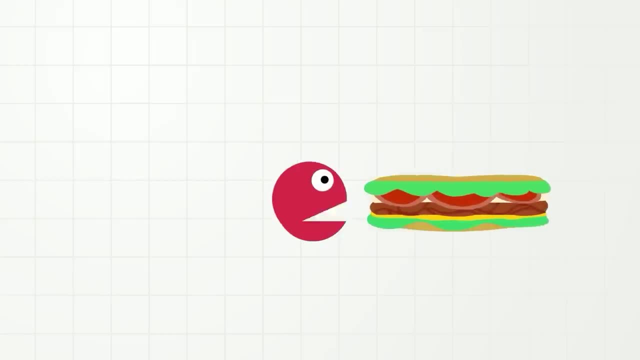 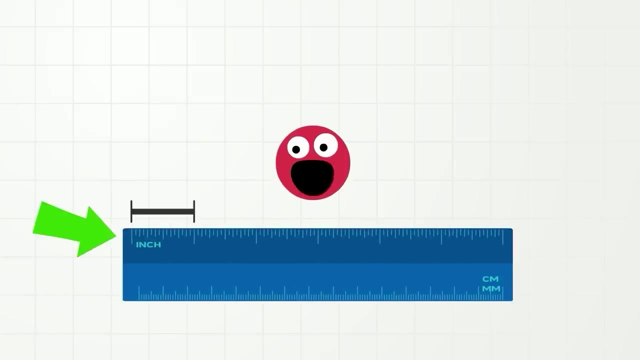 So why don't we take a break and have a snack? OK, that's enough. Anyway, when we measure the length of something, we measure with units Units. There are many standard units that you can use, like inches or centimeters. 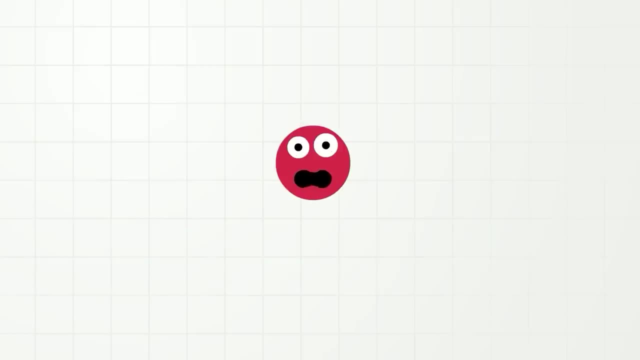 There are also many non-standard units that you can use, like paper clips. Today I want to use my favorite non-standard unit, The salamander. It's a salamander, So right now, salamander is going to be a unit that we can count and use to measure things. 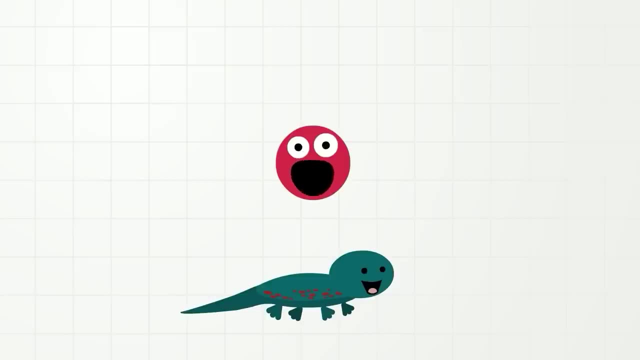 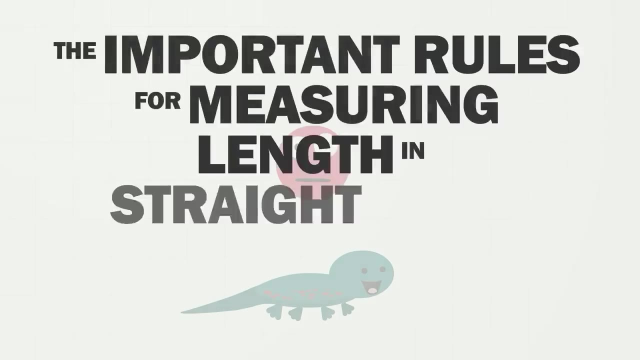 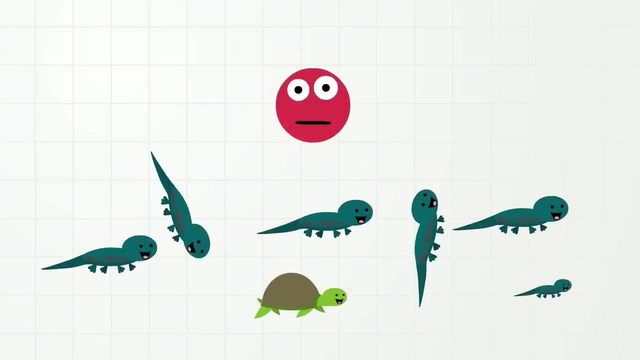 But before we do that, we need to talk about the rules for measuring, Which leads us to a new segment called The Important Rules for Measuring Length in Straight Lines with Non-Standard Units. Wow, that is a long title. Rule number one: 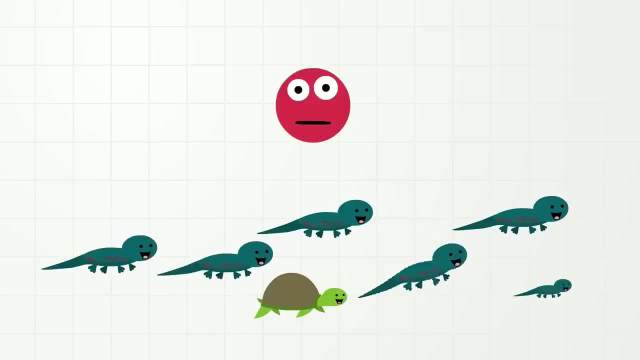 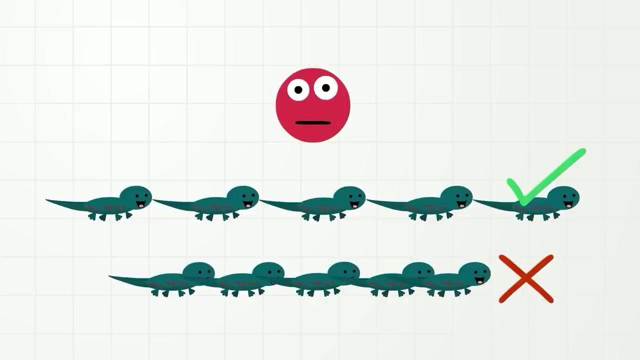 All of the units need to be the same size and direction. Sorry, super tiny salamander, Sorry turtle. Rule number two: All of the units should touch each other at the ends, but not overlap on top of each other, And they should also not be spread out. 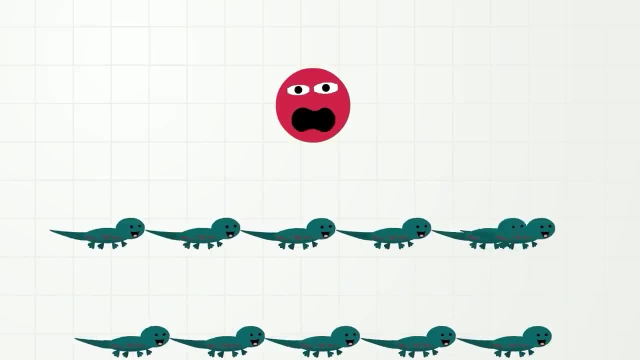 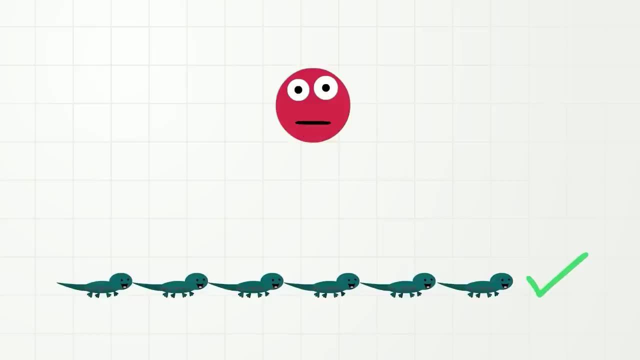 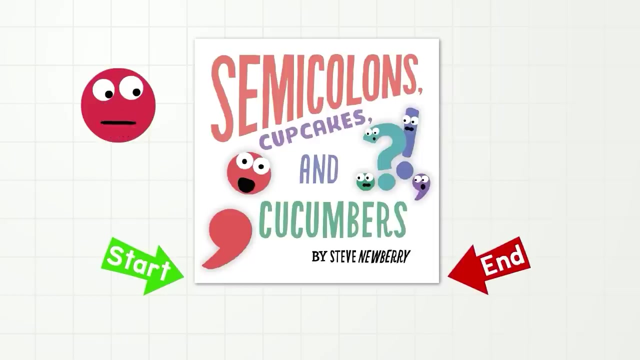 Salamanders come back. Rule number three: Usually the units need to make a straight line, Like this, But not like this. And rule number four: When measuring something, for example the length of this book, we start the units next to one end of the book and finish at the other end of the book. 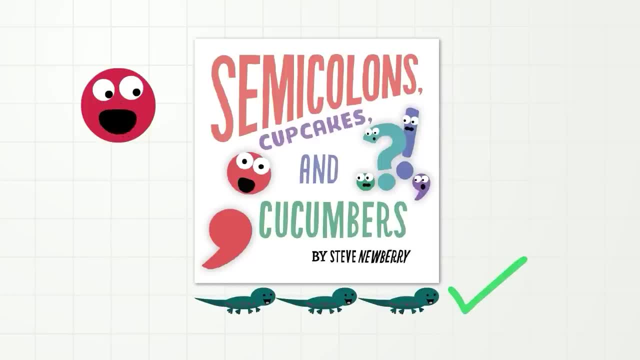 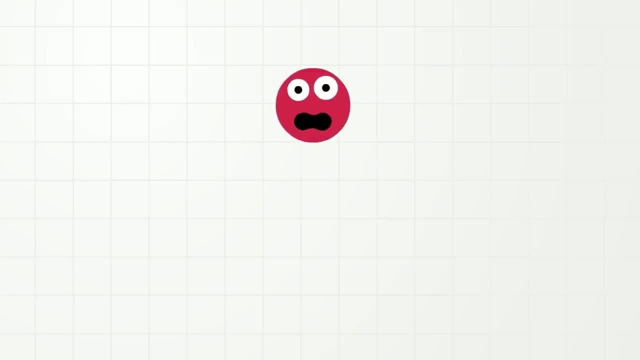 Like this, So we don't start from the center of the book and we don't start from over here or in some other place, like, uh, the beach. Okay, That now ends the part of the show called The Important Rules for Measuring Length in Straight Lines with Non-Standard Units. 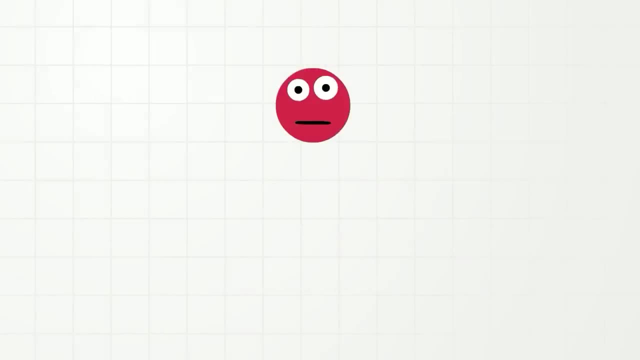 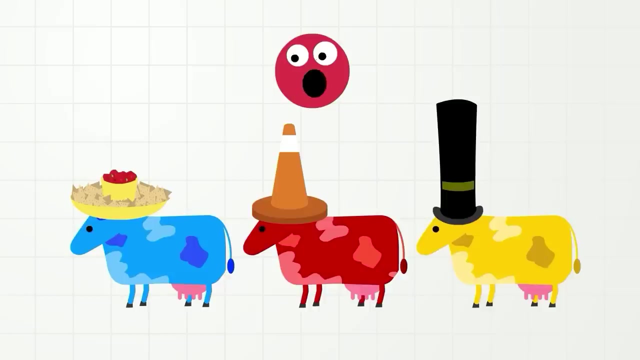 Okay, So now let's do some measuring. First, we need something to measure. What should we use? Oh, I know How. about cows With funny hats? Ha Okay, We have three cows: Blue cow, red cow and yellow cow. 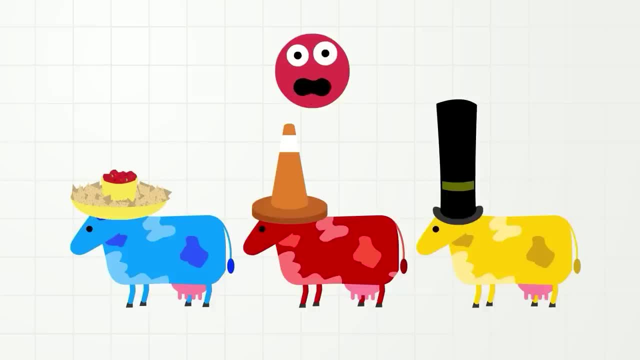 And they all have funny hats. But I want to know which cow has the tallest hat. So we will have to measure the length, or some might call it the height of each cow's hat, And first up is blue cow. Let's measure the height of blue cow's hat with salamanders. 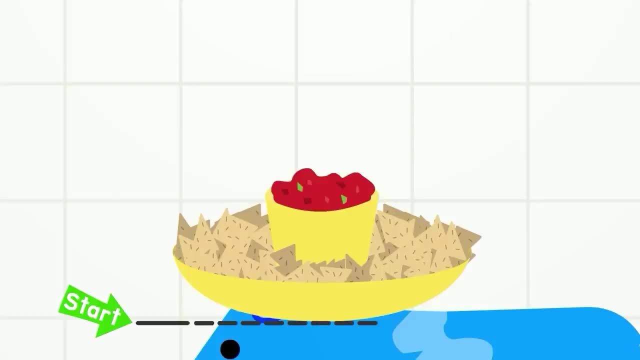 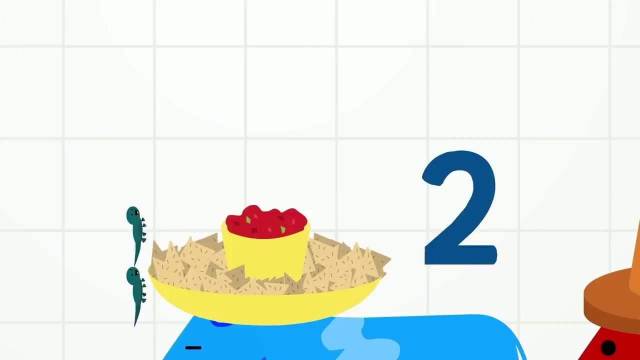 Remember we start measuring at one end of the hat and go in a straight line next to the hat all the way to the other end of the hat. So blue cow's hat is one, two salamanders long, Or we can also say two salamanders high. 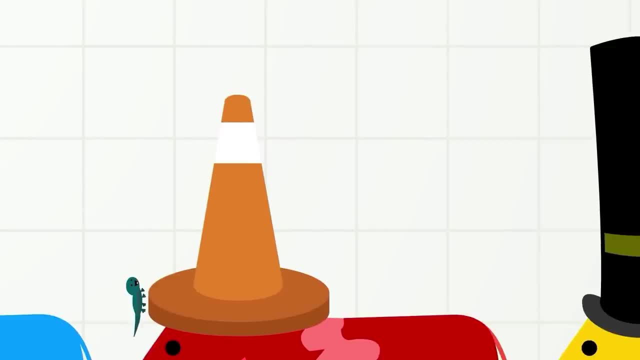 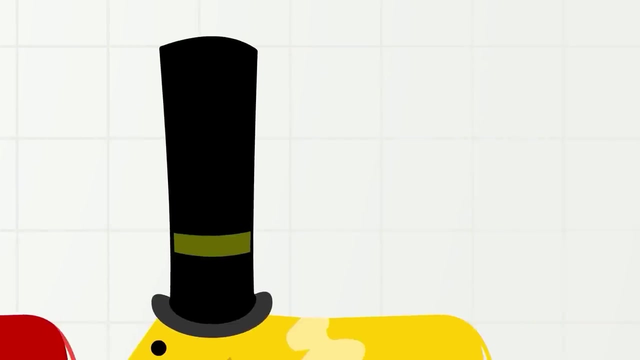 Okay, red cow. Red cow's hat is one, two, three, four salamanders long, Or we can also say four salamanders high. And last is yellow cow. Yellow cow's hat is one, two, three, four, five salamanders long. 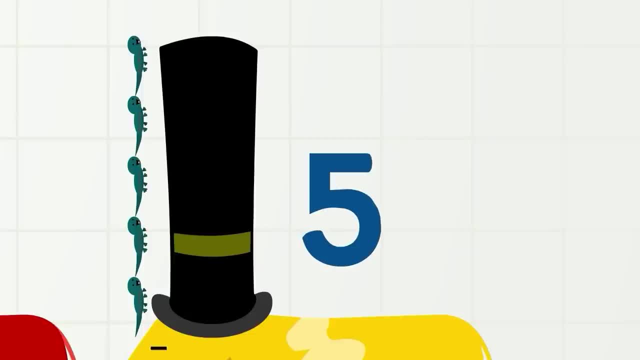 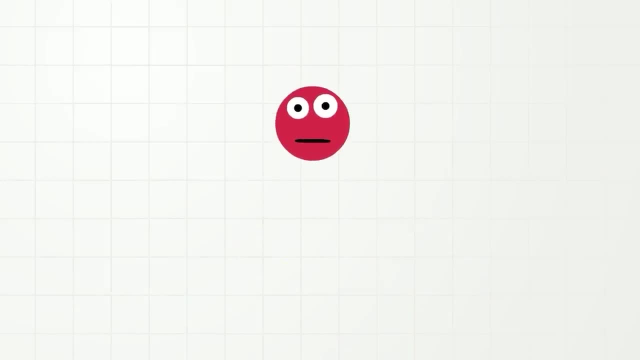 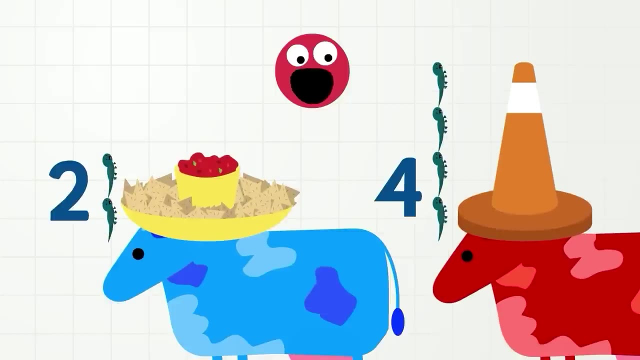 Or we can also say five salamanders high. Now let's compare hats, But first snack time, Hum, Hum, Okay, that's enough. So blue cow's hat is two salamanders high And red cow's hat is four salamanders high. 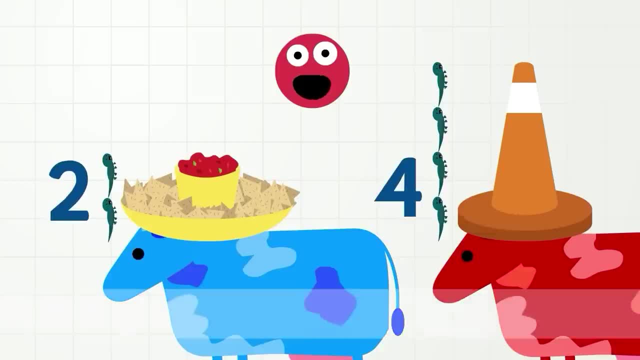 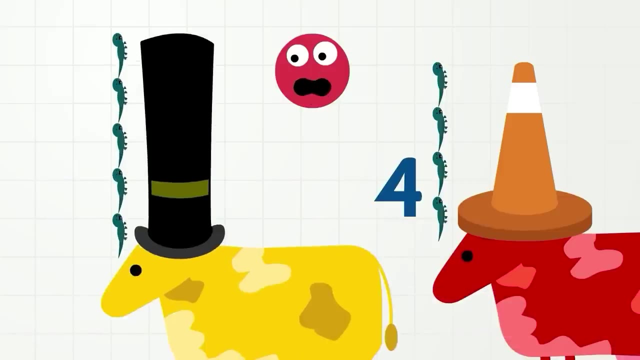 Four is a larger number than two, So that means that red cow's hat is taller than blue cow's hat, And the opposite is also true: Blue cow's hat is shorter than red cow's hat. Now if we look at yellow cow's hat, 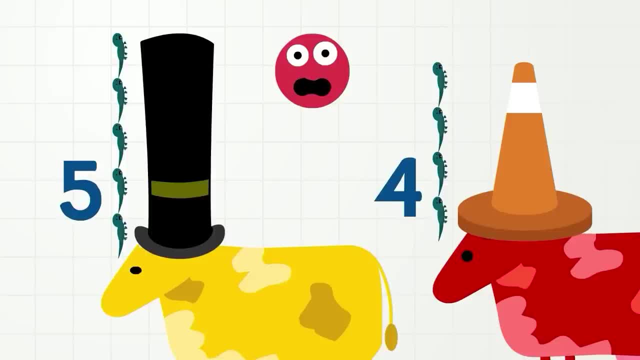 it is five salamanders. high Five is a larger number than four. So this means that yellow cow's hat is taller than red cow's hat, And the opposite is also true: Red cow's hat is shorter than yellow cow's hat. 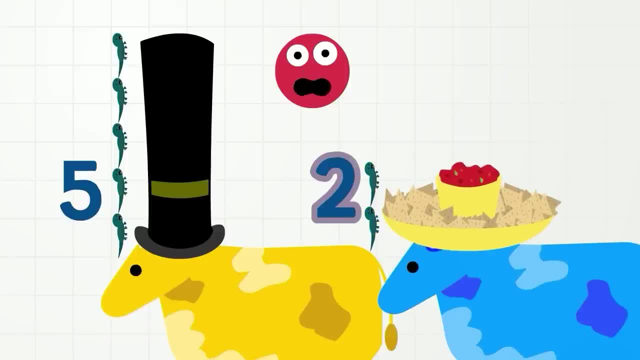 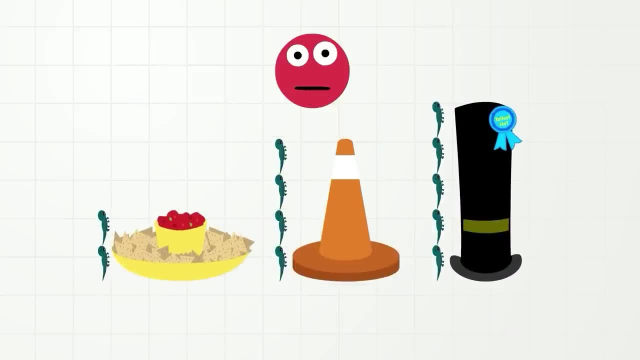 And five is also a larger number than two, Which means that out of all of the cow's hats that you can see right now, yellow cow's hat is the tallest Hat. Taller hat, Tallest hat- Yay, Okay, good job. 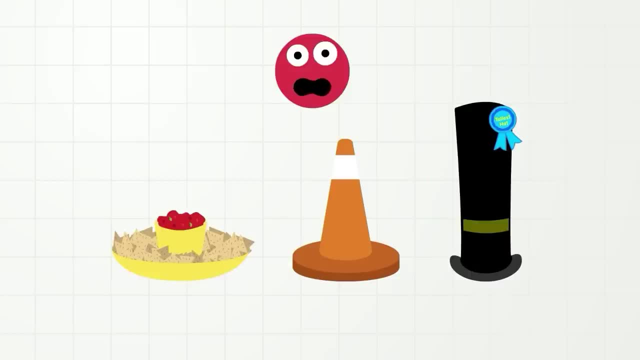 Now that you're getting better, let's measure how wide each of the cow's hats are. We call this the width Width, And instead of measuring up, we will measure from side to side, From left to right. Ready, Let's go. 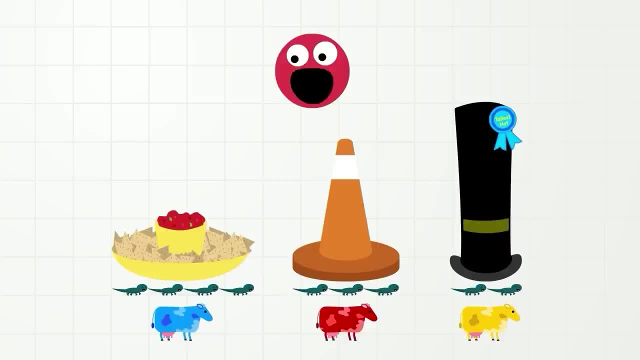 So how many salamanders wide is blue cow's hat, And how many salamanders wide is red cow's hat, And finally, how many salamanders wide is yellow cow's hat. So which cow has the widest hat? 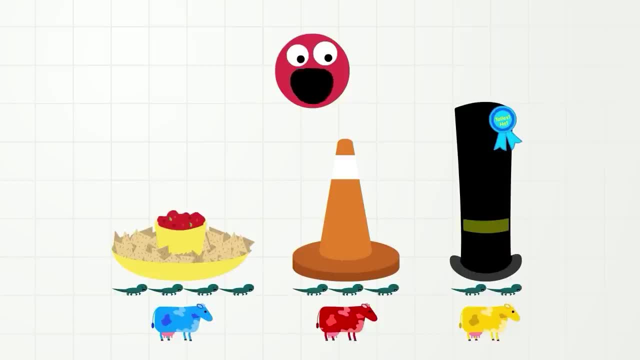 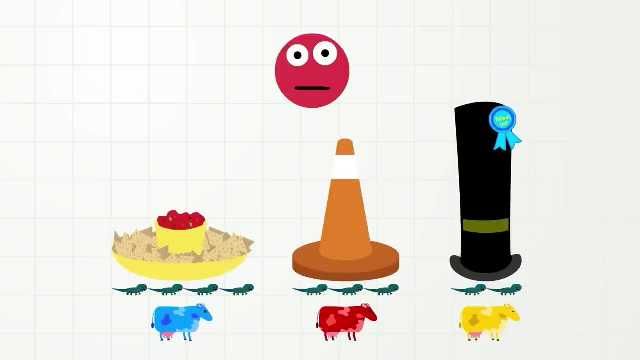 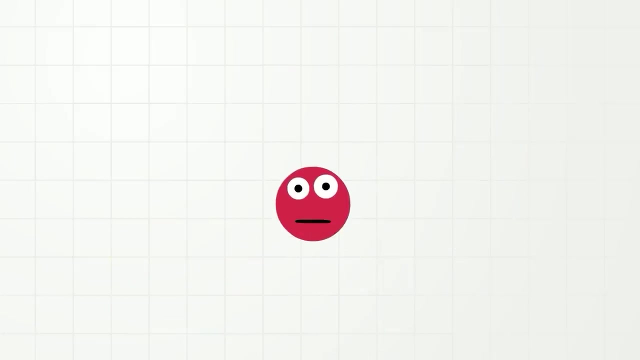 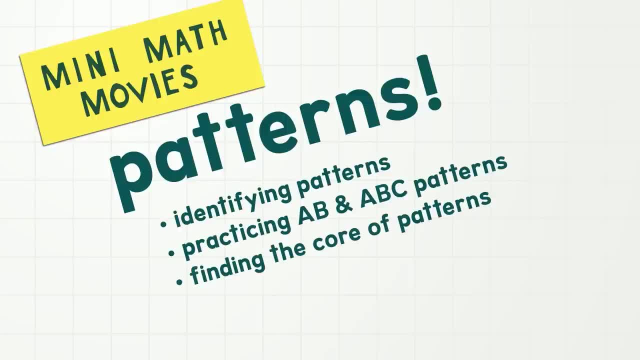 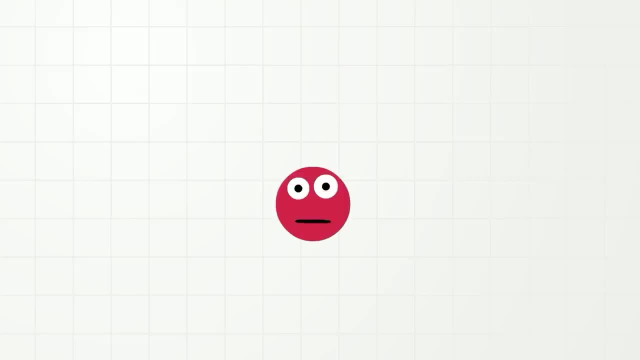 Oh, hi everybody. today I'm going to talk to you about patterns and patterns, and maybe even patterns- ha, I really like patterns. OK, so a pattern is something that happens again and again, and when something happens again and again, we say that it repeats, repeats, boop, repeats, boop, repeats, boop. 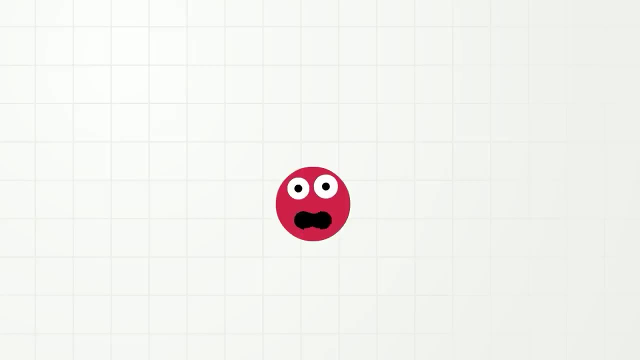 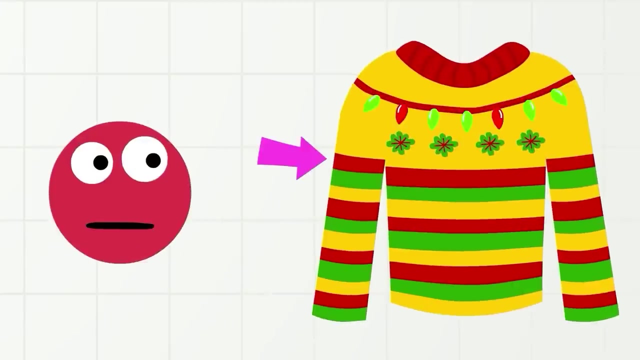 OK, that was a pattern that was made by repeating sounds and repeating actions. But did you know we can also see patterns? Oh, yes, we can. For example, look at this beautiful sweater. oh wow, If you look closely, the same kind of stripes happen again and again: red, green, yellow. 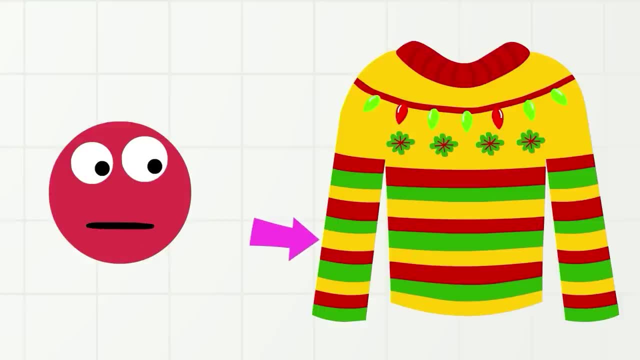 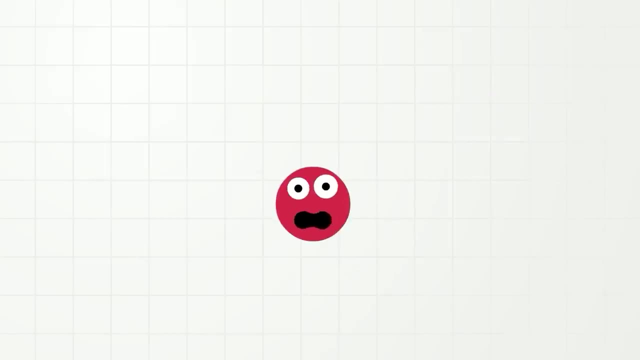 then red green yellow, then red green yellow, And when the same things happen again and again and in the same order, it is called a pattern. and a pattern always repeats, repeats, boop. OK, so let us practice some patterns together. 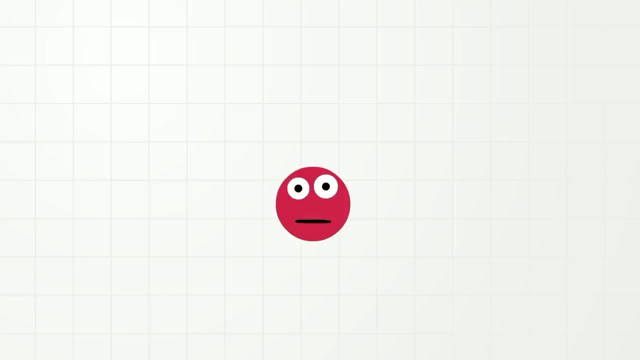 And first we are going to practice with our hands. Most people have two hands: a left hand and a right hand. Now let's make a pattern: When I say left, raise your left hand high. When I say right, raise your right hand high. 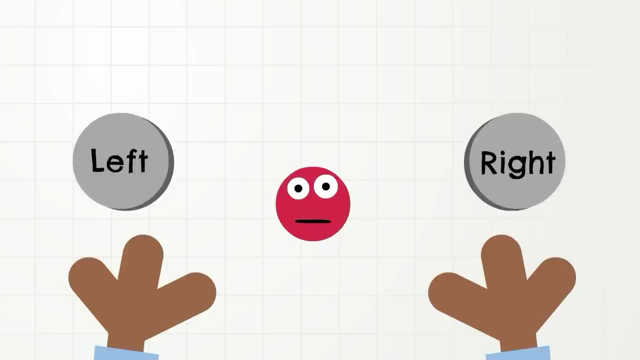 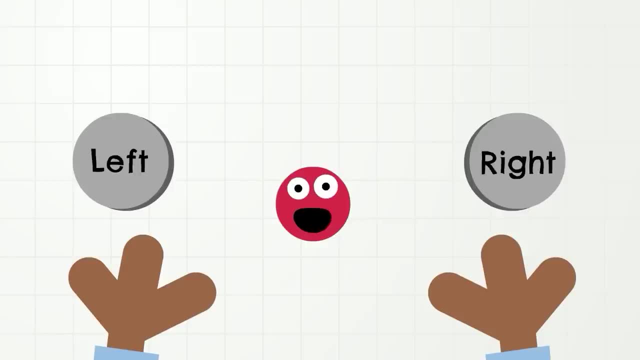 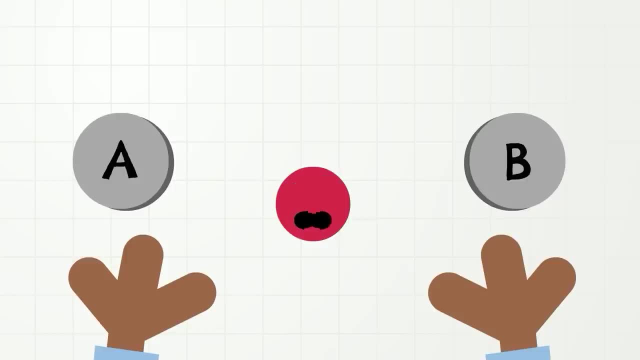 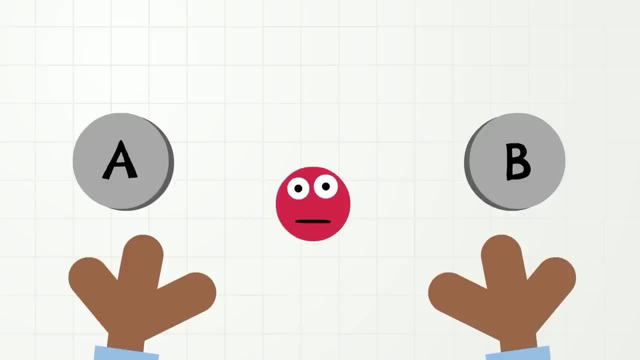 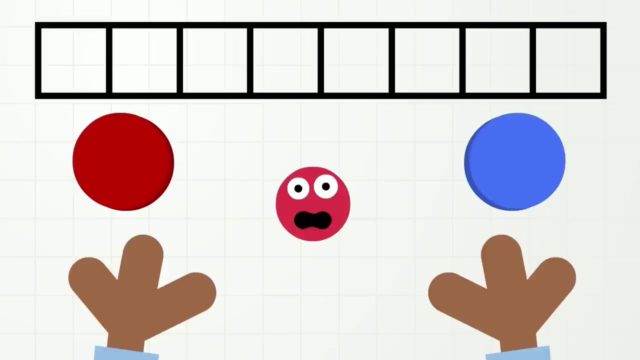 B pattern Fascinating. OK, now let's make an A B pattern, but with colors Red and blue, And we will also see what this pattern could look like too. at the same time, Ready, OK, go. Red, blue. 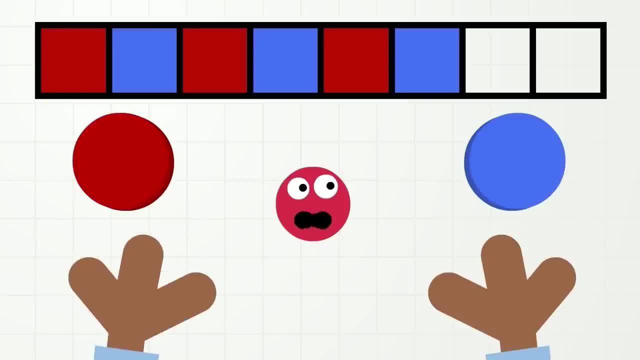 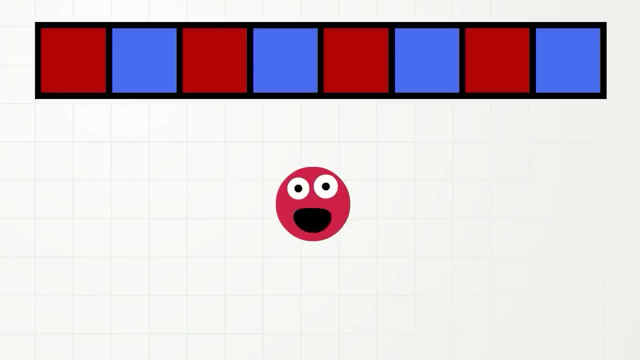 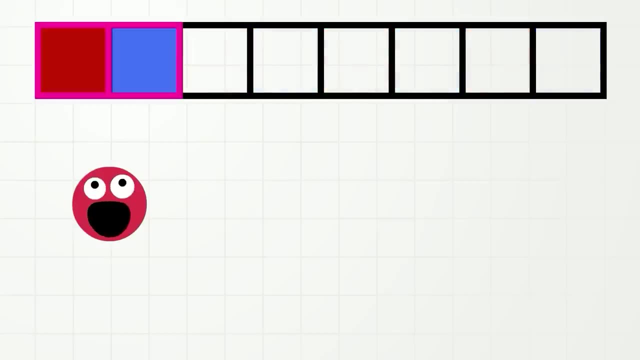 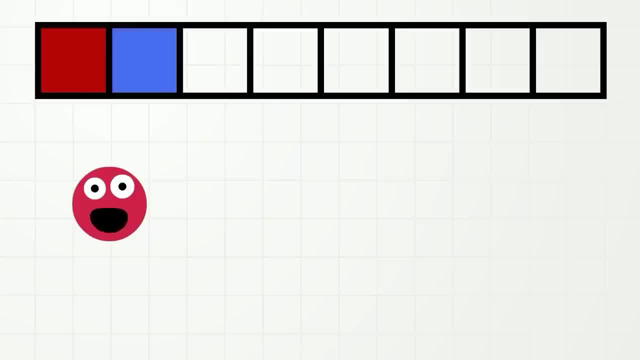 It is not just the red that happens again and again, and it is not just the blue that happens again and again. It is the red and the blue together, And it is this red and blue core that always repeats, Repeats, Boop. 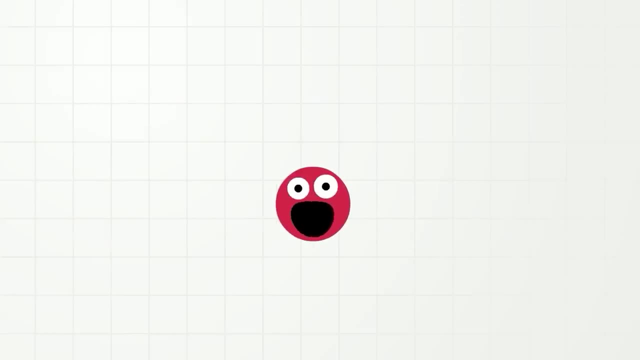 OK, you've done such a good job, it is now time for a break outside. OK, that's enough. Now let's make some more patterns, but this time, instead of two different things that repeat, there will be three different things that repeat. 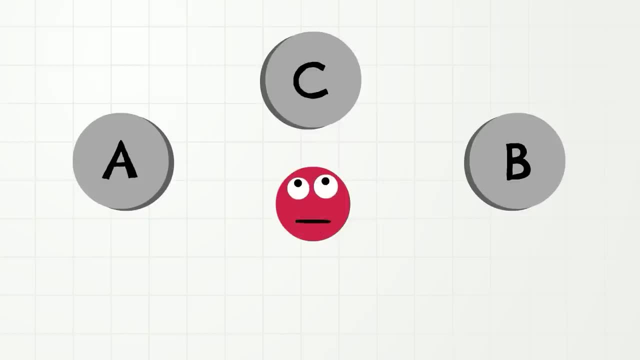 And this is sometimes called an A-B-C pattern. so let's use those letters Now. instead of the order going left and right, it is going to go left right up. Let's do this together with our hands and our voices. 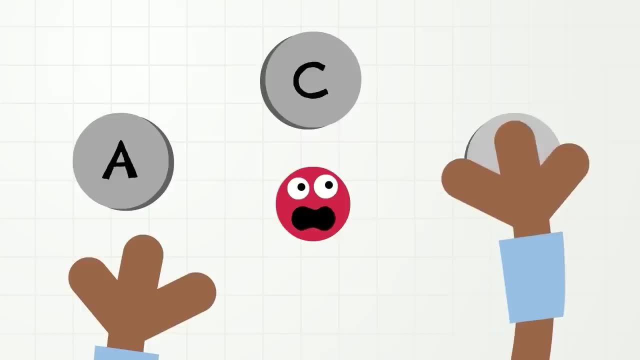 Ready. OK, go A-B-C, A-B-C, A-B-C, A-B-C. Wow, OK, let's do another three thing pattern, but this time with something else. What can we use? Oh, I know How. about Popcorn, Unicorn and Mustache? 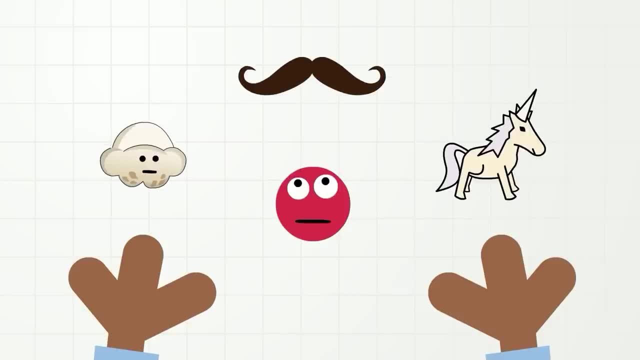 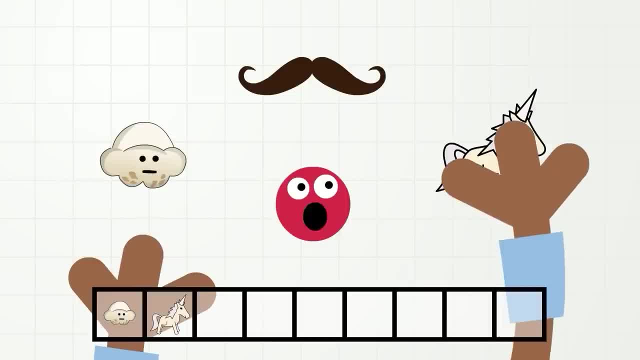 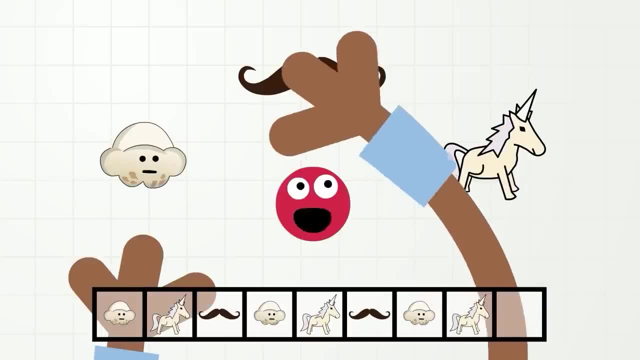 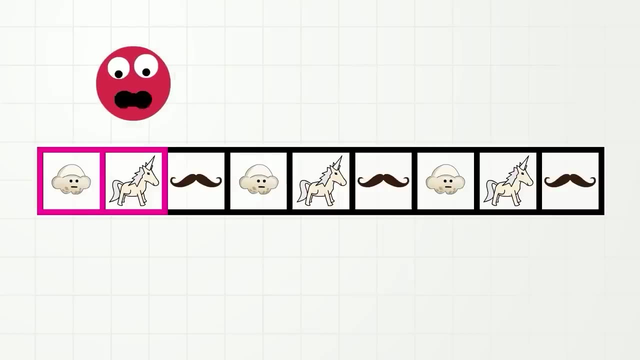 Ready? OK go. Popcorn Unicorn Mustache. Popcorn Unicorn Mustache. Popcorn Unicorn Mustache. OK, good job. So we know that this is a pattern with three things: Popcorn, Unicorn Mustache and that 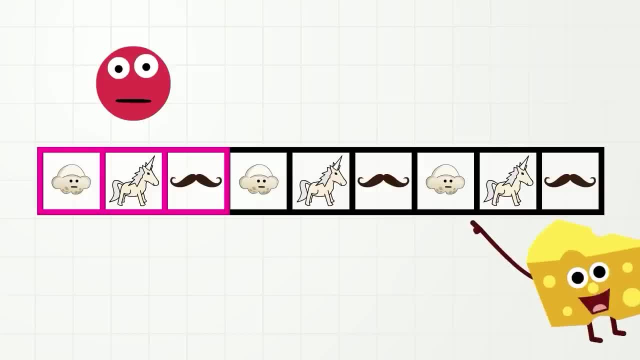 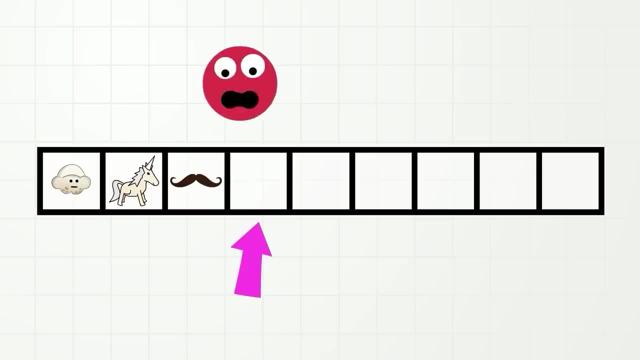 this is the core of the pattern Popcorn Unicorn Mustache. always repeats, Repeats, And now I have some questions. Question number one: Here is the core of the pattern Popcorn unicorn mustache. So what would come next? right here? 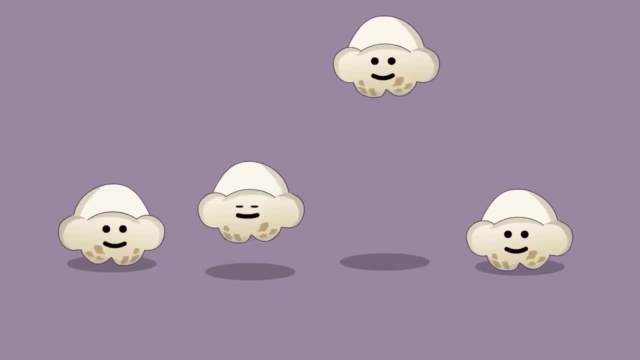 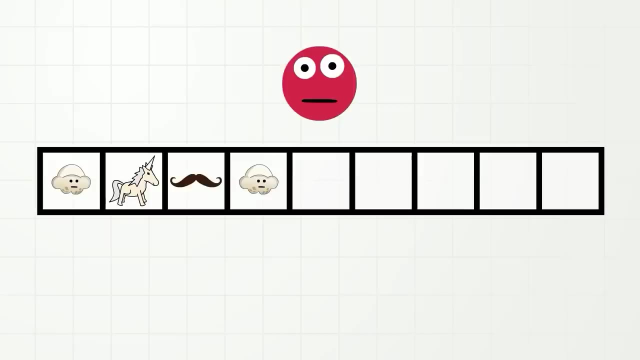 That's right, It would be popcorn, Yay, And after popcorn, right here, what would come next? That's right, It would be unicorn. Yay, And after unicorn, what would come next? That's right, It would be mustache. 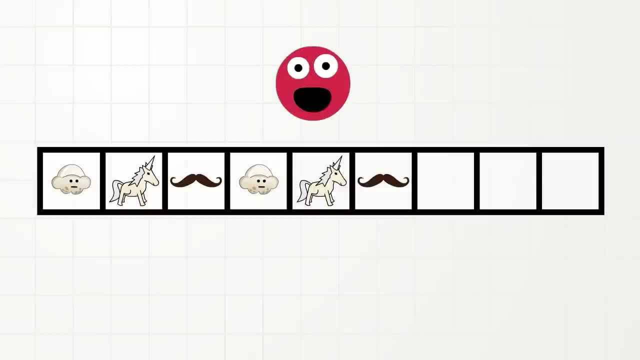 Yay. Question number two: What do you think would happen if the pattern keeps going? Do you think it would stay the same or be different? That's right, It would stay the same. The pattern would be the same before and after. 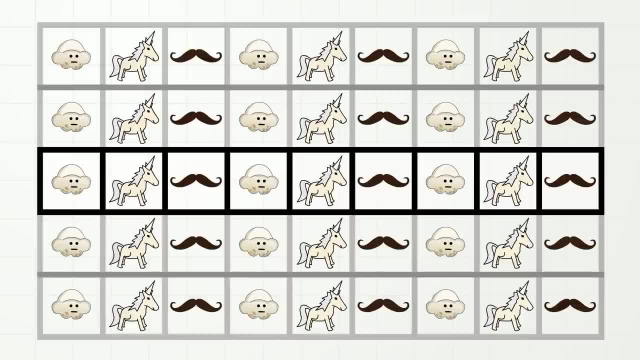 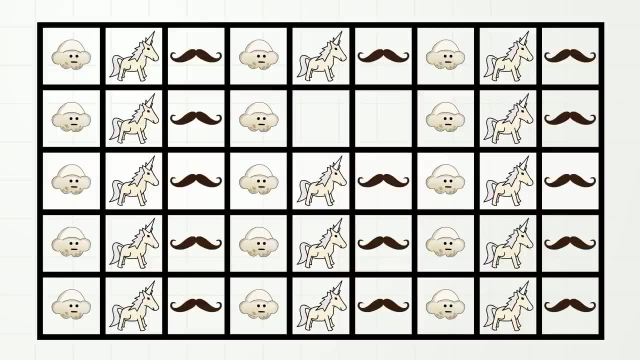 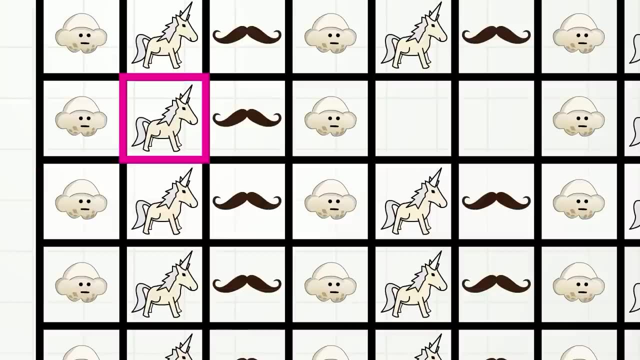 Watch, Ah, And last question: Oh Oh no, Some of the pattern is missing. Can you help me fill it in? Let's look. just before the missing spaces There is popcorn, unicorn mustache, Then popcorn. So here would be what. 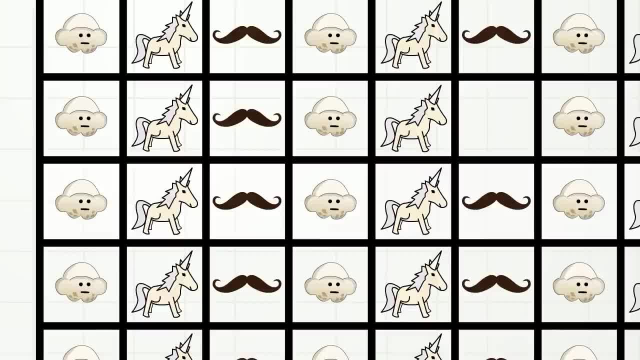 That's right, Unicorn, And let's try to figure out the The last space. So there is popcorn unicorn mustache, popcorn unicorn- orange juice. No, let's try again. OK, popcorn unicorn mustache. popcorn unicorn- a pink airplane with a funny hat. 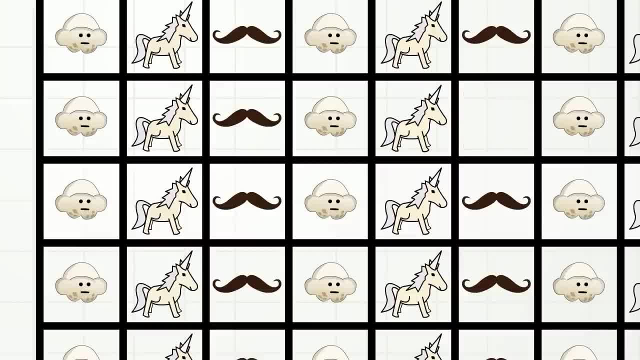 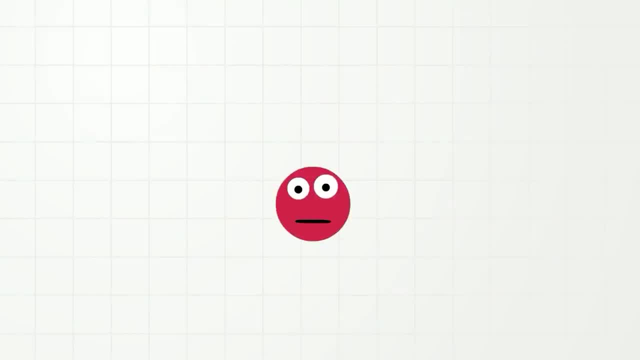 OK, OK, wait. no, let's try one last time. There is popcorn unicorn mustache. popcorn unicorn mustache. Yay, OK, you've done such a good job. it is now time for a break outside. 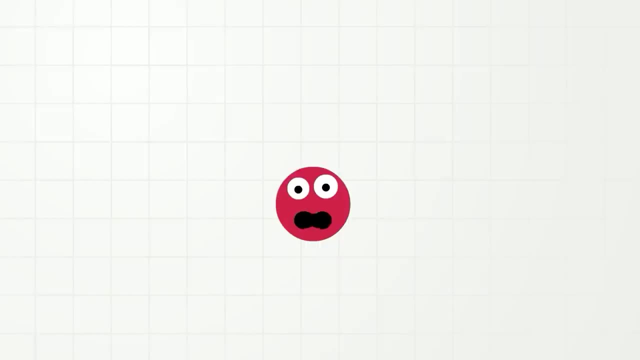 OK, that's enough. OK, that is all the time today we have for patterns. Oh, hi everybody. today I am going to talk to you about shapes and attributes, and maybe even rocket ships. Oh, I really like rocket ships. 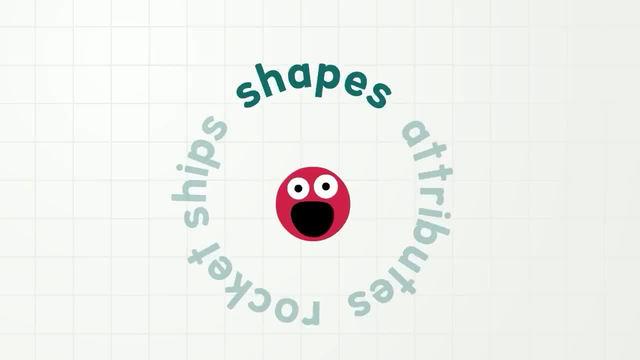 OK, did you know that shapes are all around us? Ahem, I said, did you know that shapes are all around us? Shapes come around me. OK, that's a matter, So let us practice the names of these shapes. 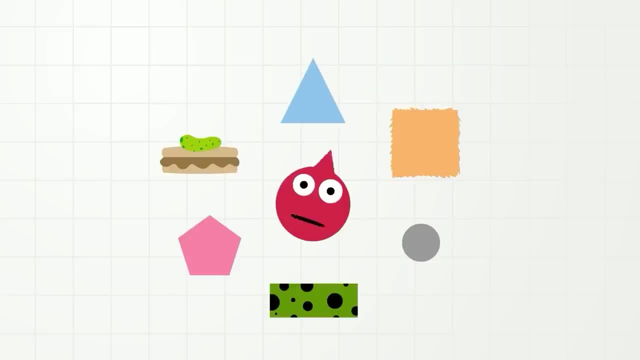 We will start with triangle, square, circle, rectangle, pentagon and peanut butter sandwich with a pickle on top. Shapes all have something we call attributes, Attributes. That's right. Attributes, Attributes, Attributes. An attribute is something about a shape or something that a shape has that makes it. 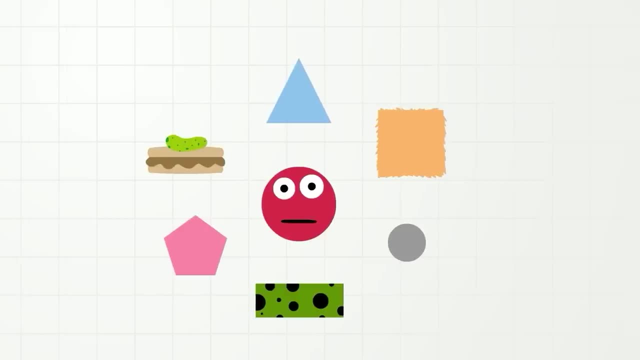 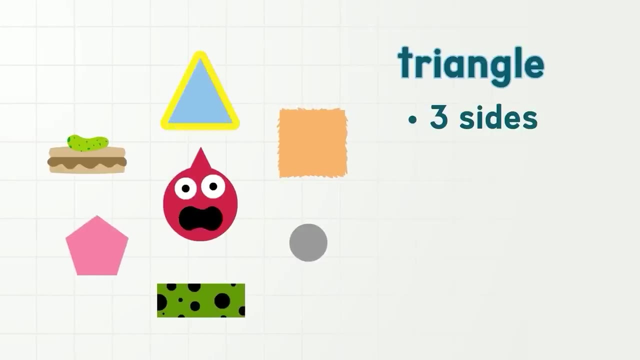 different or similar to another shape. For example, triangle has three sides- one, two, three- And is blue. Attributes: A square has four sides the same length: one, two, three Attributes, Attributes, Attributes. For example, rectangle has two sides- two, three, four- and is kind of furry. 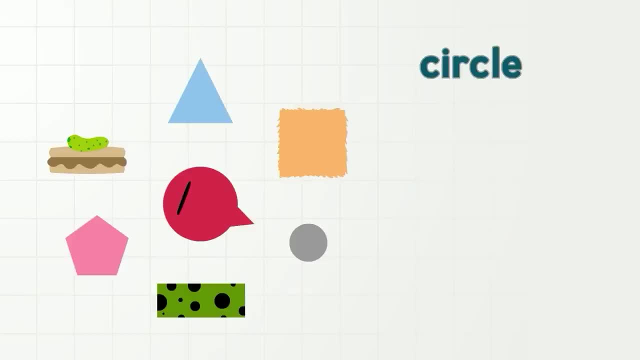 Attributes Circle. wow, what a great shape. It's kind of small, has zero sides and is grey. Attributes Rectangle has four sides: one, two, three, four- But the sides are not all the same length And rectangle has spots. 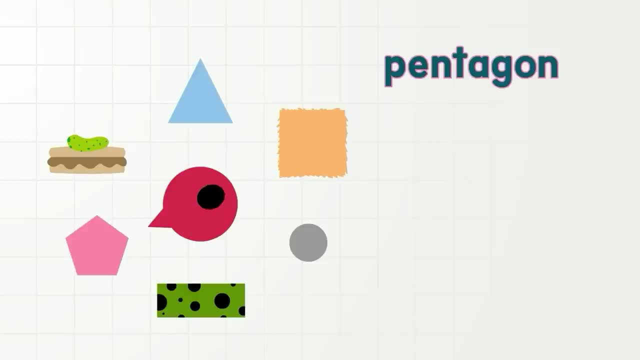 spots Attributes And pentagon has five- Wow, Five sides: One, two, three, four, five, And it's pink. Attributes And peanut butter sandwich with a pickle on top. Well, uh is brown and green and 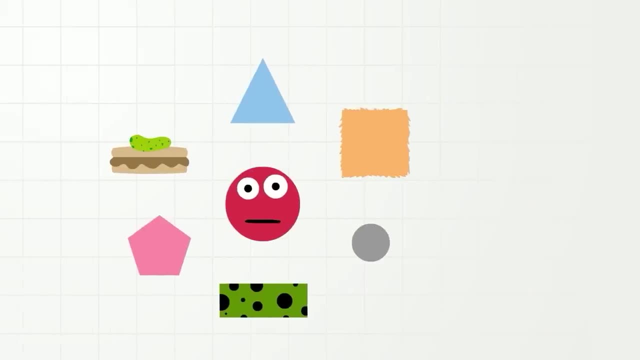 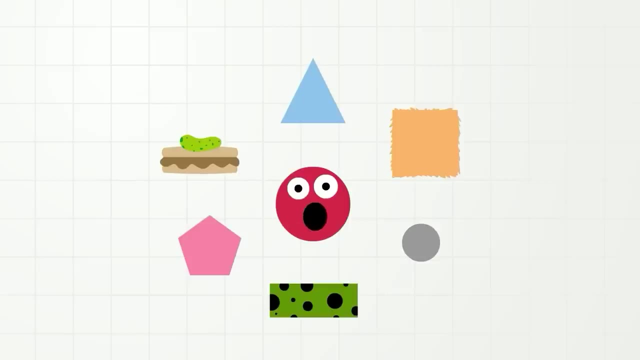 maybe delicious Attributes. And did you know that shapes can be sorted? Oh, yes, they can. When you sort things, you put them into different groups. For example, I want to sort all the shapes that are around me into two groups. I want all the shapes that are food to go to the right side. 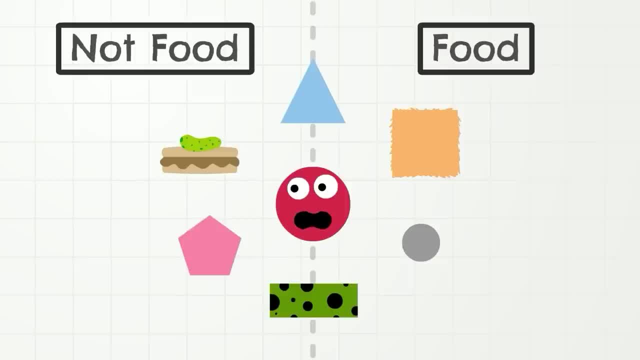 over here and all the shapes that are not food to go to the left side over here, Okay, shapes. And pentagon has five. Wow, Five sides: One, two, three, four, five, And pentagon has five. 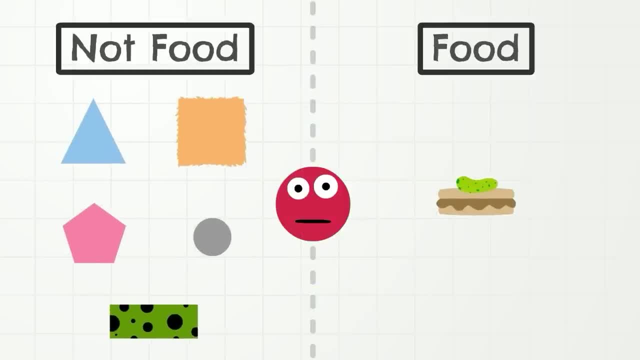 Shapes Sort Whoa. good job, Peanut butter sandwich with a pickle on top. Since you are kind of more like food and not a shape, you shouldn't really be here. Sorry, you need to take a rocket ship out of here. Oh, rocket ship, Thank you. Okay, so now I want to sort some shapes. 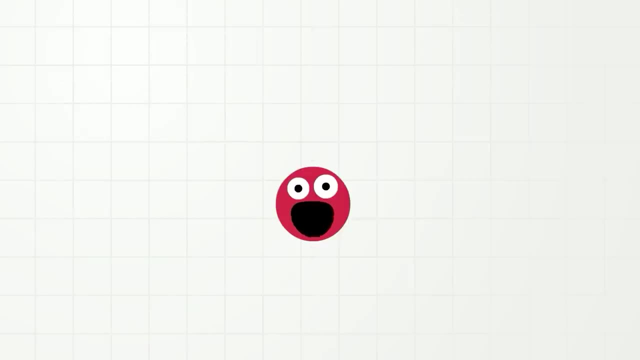 together. But first let's have a break and take a refreshing dip in the pool. Okay, that's enough. Let me introduce you to my new machine called the ShapeMaker 17 and 1 1⁄2.. The ShapeMaker 17 and 1 1⁄2 will make some shapes for us, but I need you to help me sort them. 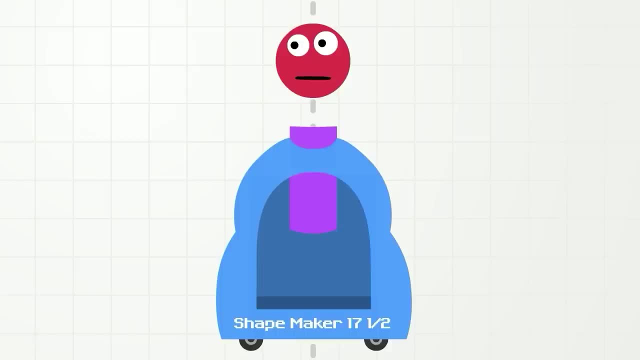 You can tell me which side- the right side or the left side- the shape should go according to an attribute- Attribute. The first attribute is color. If the shape is red, it should go on the right side. If the shape is yellow, it should go on the left side. If the shape is red, it should go. 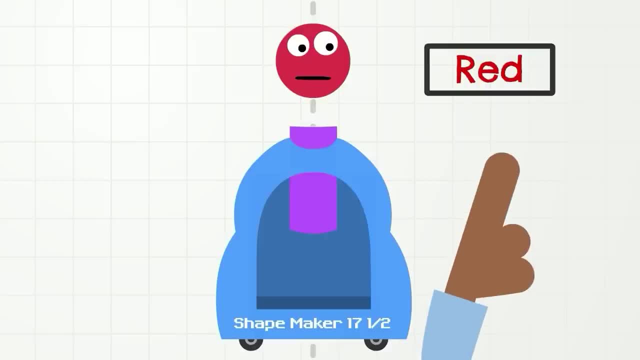 on the right side. So you can point to the right side like this: If the shape is green, it should go to the left side. So you can point to the left side like this: Okay, ShapeMaker 17 and 1 1⁄2, start. 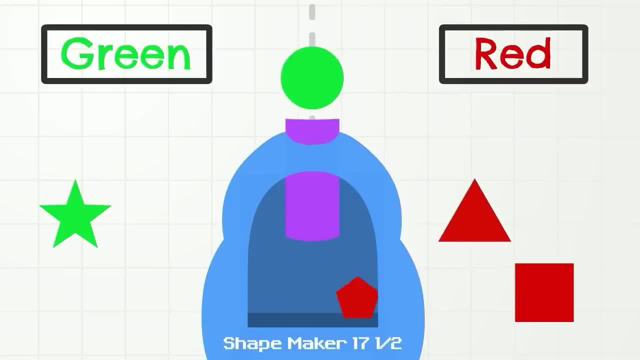 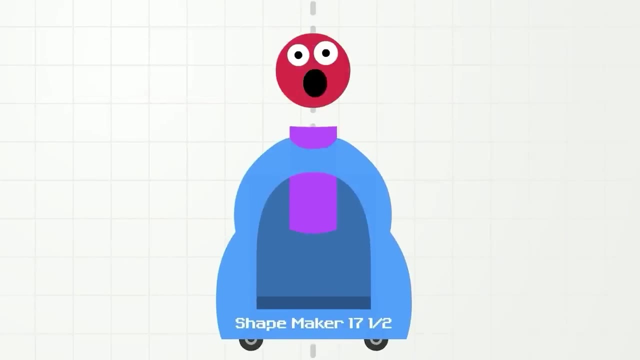 Wow, good job everybody. Okay, let's sort some more shapes. This time the attribute is number of sides. If the shape has the four sides, it should go on the right side, And if the shape has the three sides, it should go on the left side. So you can point to the right side like this, If the shape is. 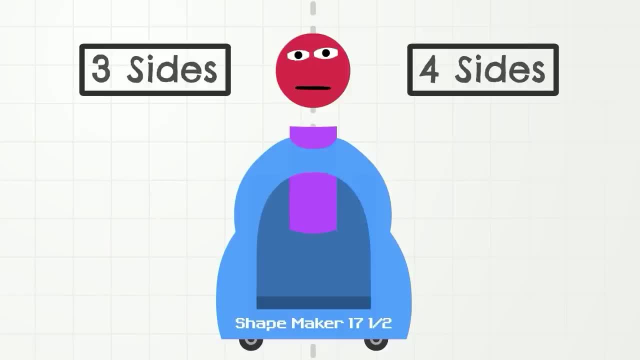 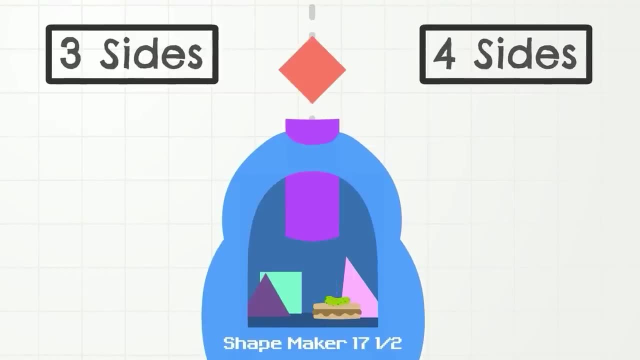 three sides. it should go on the left side. Okay, ShapeMaker 17 and 1⁄2, start. Or maybe we should do the first one together. This shape has one, two, three, four sides, So it should go on the right. 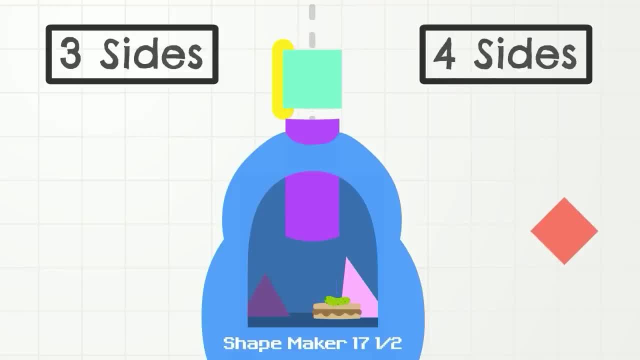 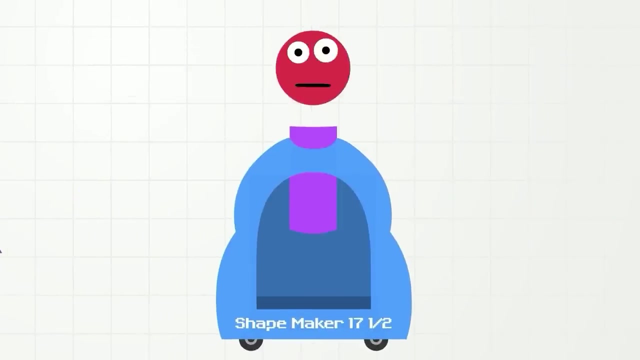 side. Yay, Hey, how did peanut butter sandwich with a pickle on top get there? Oh, rocket ship, Thank you, Wow, everybody's doing great. So now let's sort some more shapes one last time, but first let's have a break and take a refreshing dip in the pool. 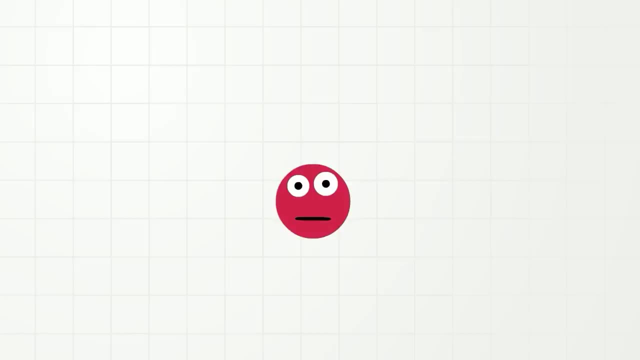 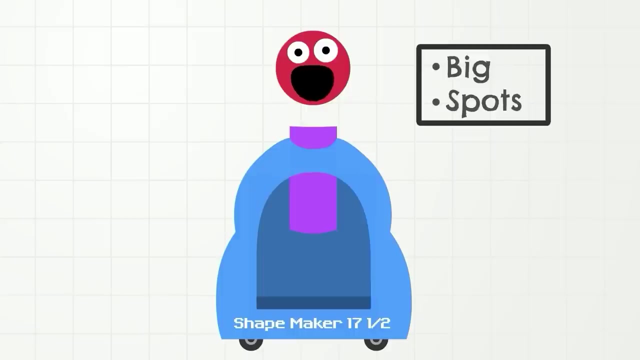 Backstroke Front crawl. Okay, that's enough. Did you know that you can sort by more than one attribute? Oh, yes, you can. This time the attributes are size and spots. So if the shape is big and has spots, 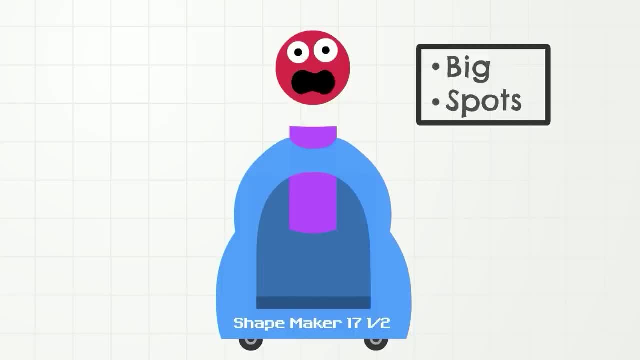 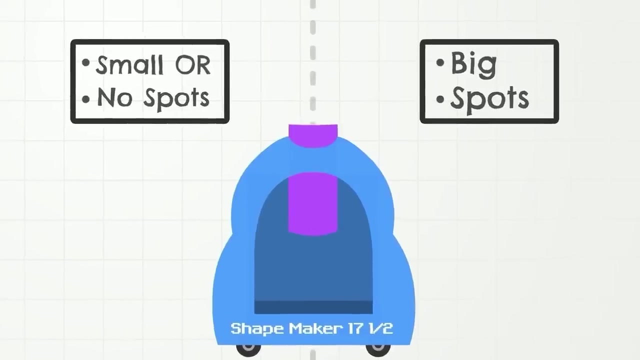 it should go on the right side And if the shape is small or doesn't have spots, it should go on the left side. Remember that the shape has to be both big and have spots to go on the right side. Okay, shape maker 17 to 1 half. 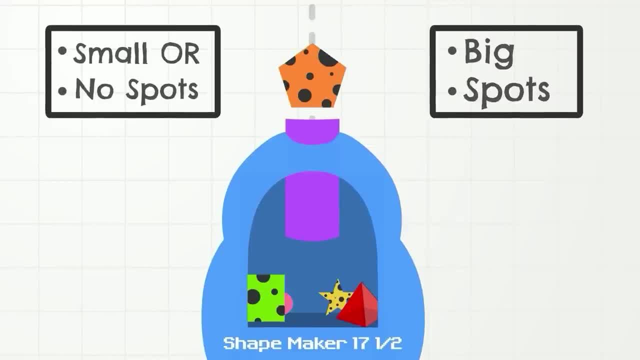 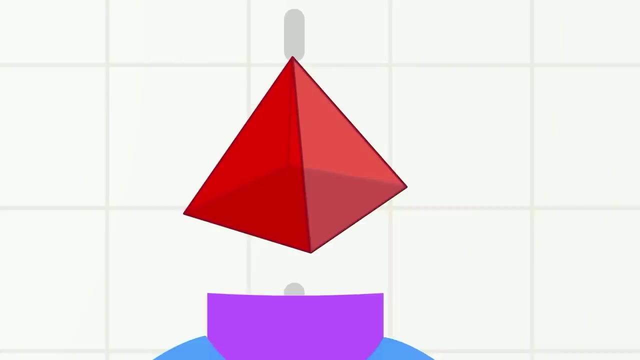 Start. Oh wait, what is this? Oh, I know. Does anybody know what this is? That's right, It's a pyramid And it is actually a 3D shape which we call an object. You can learn more about 3D shapes and objects. 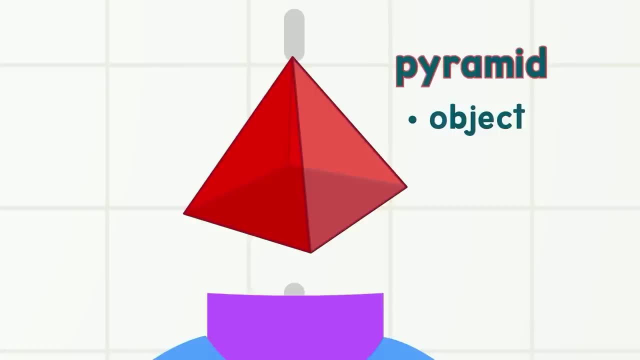 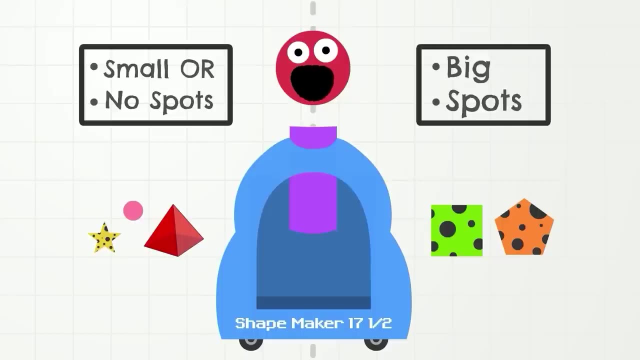 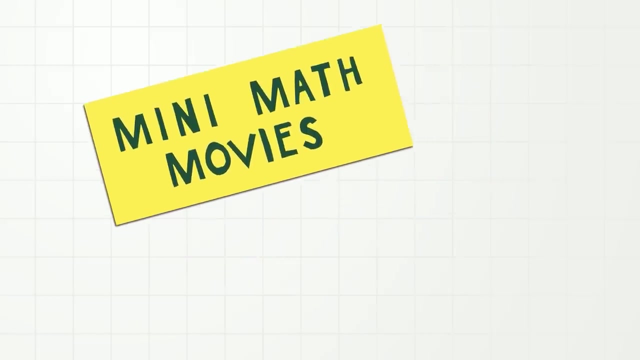 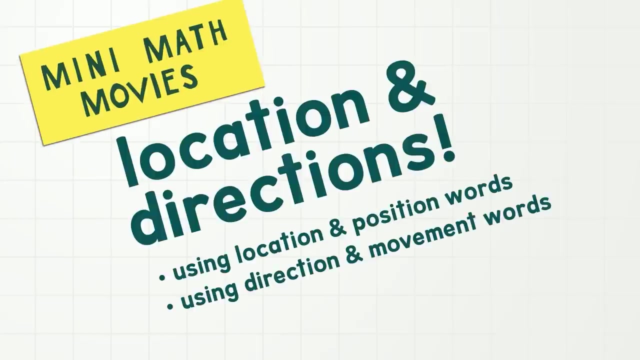 later. This pyramid is big, but it doesn't have spots Left side. Oh, great job sorting everybody. Okay, that is all the time today we have for sorting shapes. Thanks for watching. See you next time. Bye, Hi, everybody. 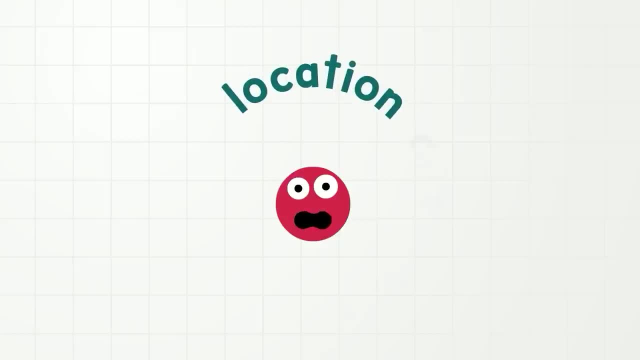 Today I am going to talk to you about location and directions and maybe even tiny robots. I really like tiny robots. So location is where something is Location. For example, somebody told me there is a monster in this video. Oh, monster. 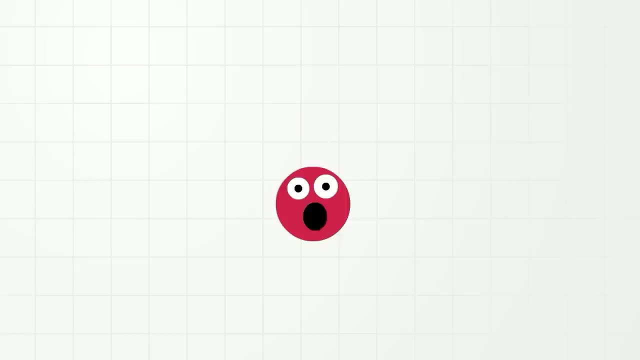 But I can't find it and I might need help locating it. Oh monster, Where is the monster? What's that? Oh, really, The monster is behind me, Behind you. Hey, I know, Is there anything behind you? 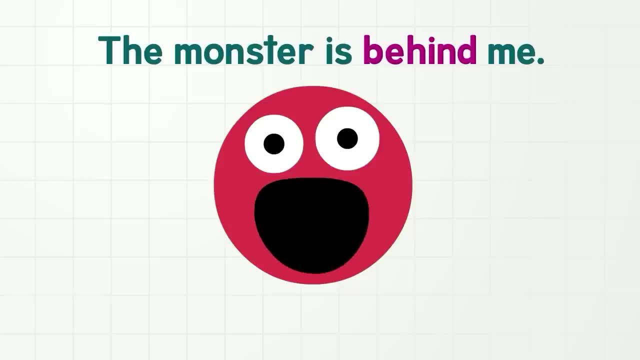 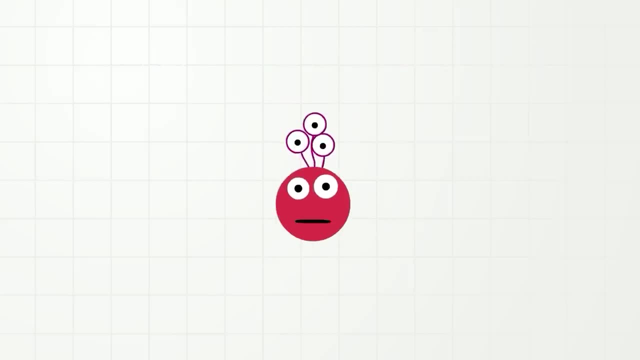 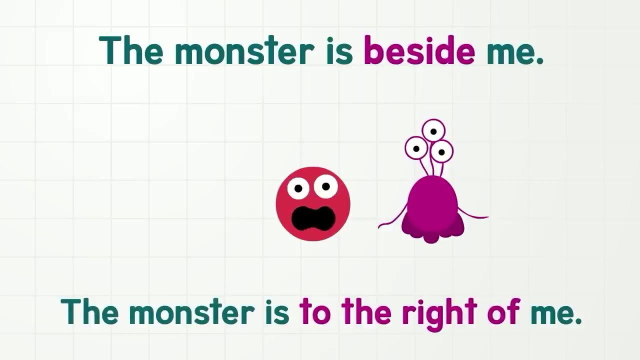 Why don't you look behind you, pick one thing and tell me what? it is? Okay, you can come on up monster. Now where is the monster? That's right. The monster is beside me. You can also say: the monster is to the right of me. 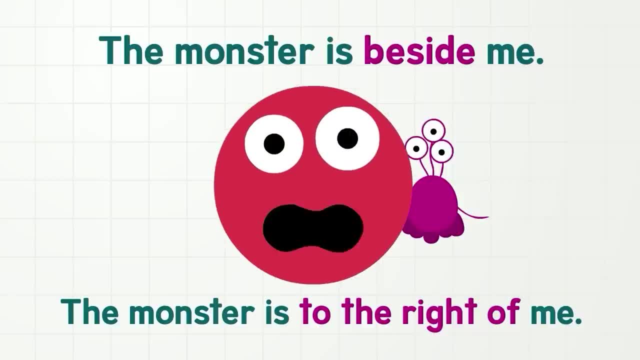 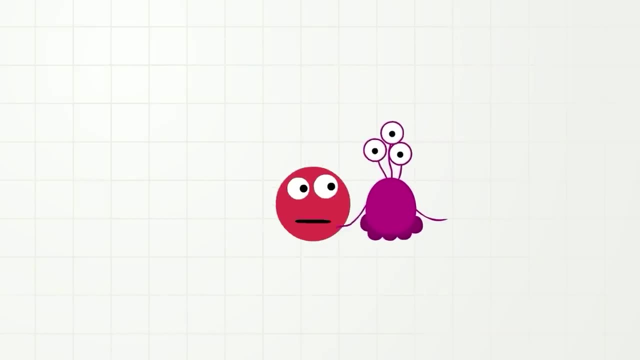 To the right of you. Hey, I know, Is there anything beside me, Beside you, On the right side? Why don't you look to the right, pick one thing and tell me what it is? Oh, now, where is the monster? 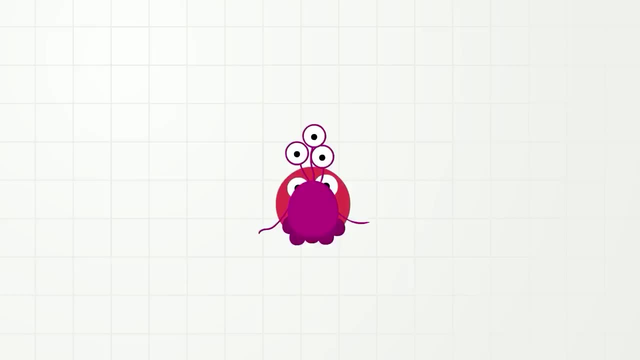 Oh hey, monster, Monster. I can't see anything. Monster, Where is the monster now? Yes, the monster is in front of me, In front of you. Can you please move, monster, I am trying to teach here. 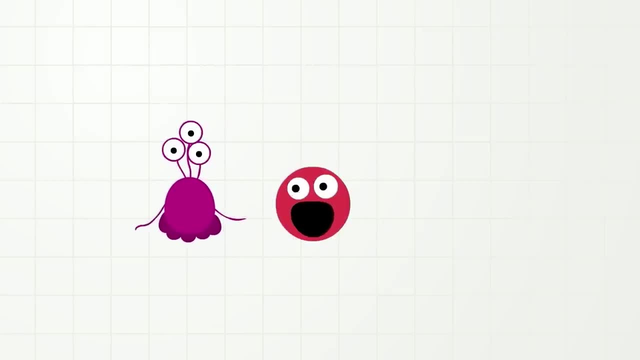 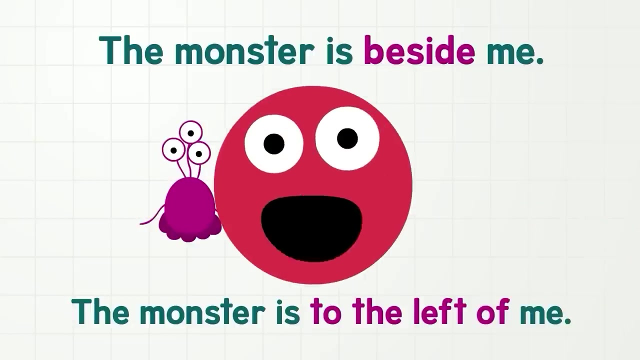 Okay, thank you. Okay, now, where is the monster? Again, the monster is beside me. You can also say: the monster is to the left of me, To the left of you. Hey, I know, Is there anything beside you? 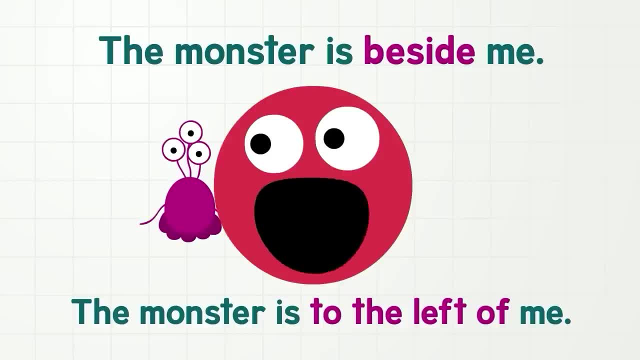 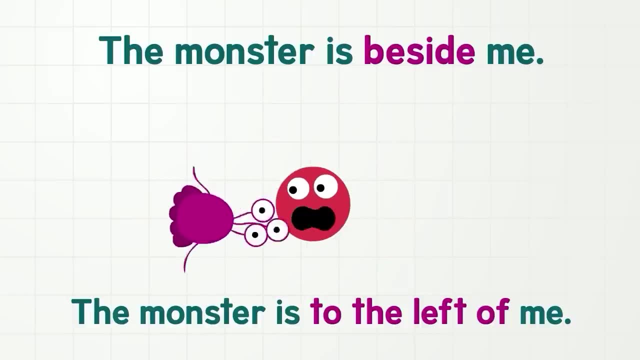 On the left side. Why don't you look to the left, pick one thing and tell me what it is? Hey monster, what are you do-? Oh look, The monster is upside down. It's still the same monster, though. 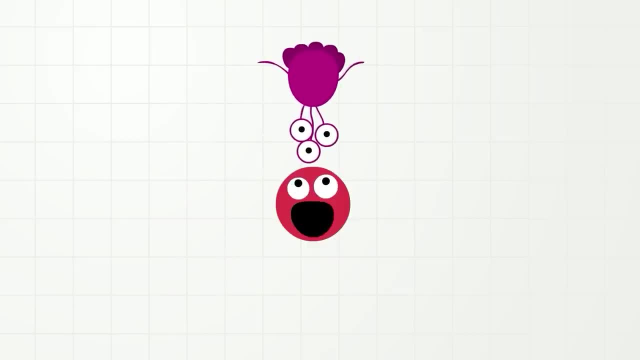 Okay, upside down monster. where are you go-? Oh, look Now, where is the monster? The monster is on top of me. Or we can also say: the monster is above me, Above you. Oh good, you are right side up again. 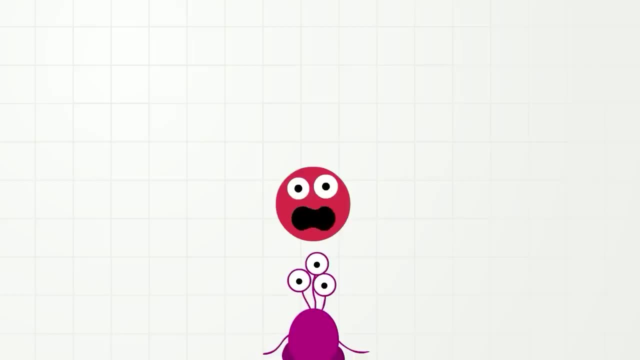 And now, where is the monster? Now, where is the monster? Yes, the monster is under me. or we can also say: the monster is below me, below you, Ok, and now the monster is above me. oh, and now the monster is below me. and now it is. 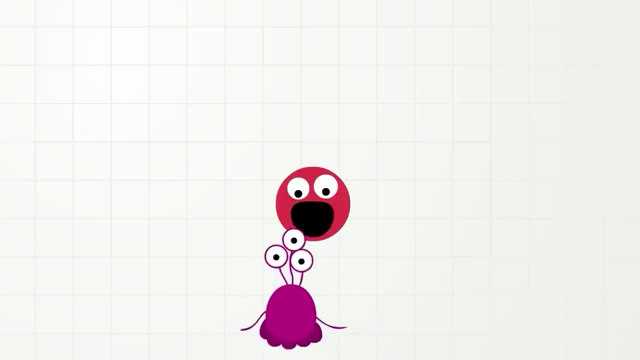 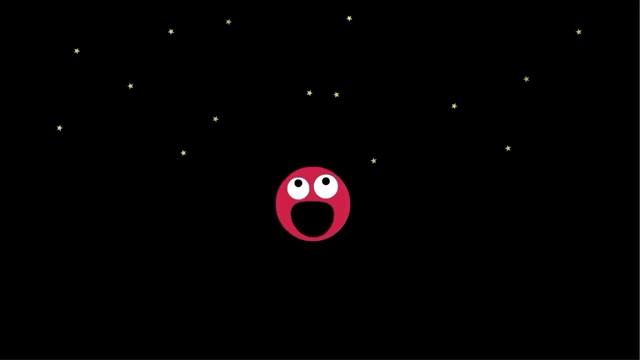 above, and now it is below, above, below, above, below, oh, and now the monster is tired. It's ok, monster, you can take a break now. And speaking of breaks, let's all take a break Under the stars. oh, so beautiful. ok, that's enough. 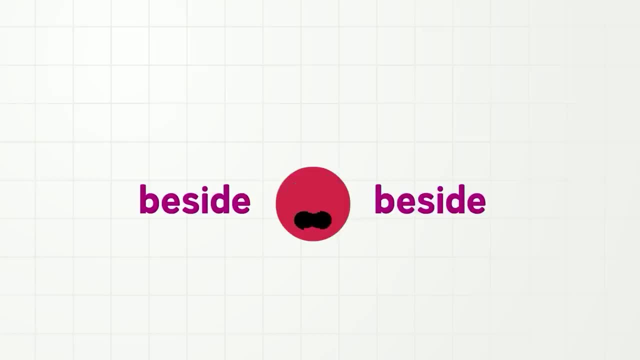 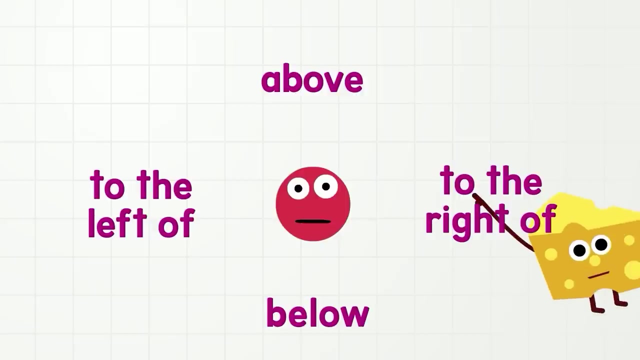 So you see, all of these words like beside, above, below, and to the left of and to the right of, these are all great words to say where something is, you know: location, location. Ok, now let's play a game. 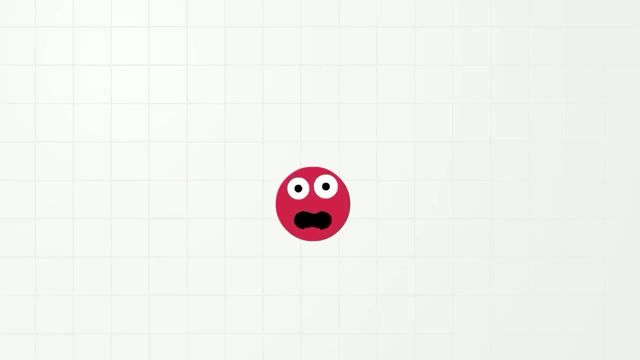 This is a game about location and directions. Directions are ways to go, And when we give directions, we tell someone with our voice which way to go. So first we need something to give directions to. hmmm, oh, I know how- about Tiny Robot? 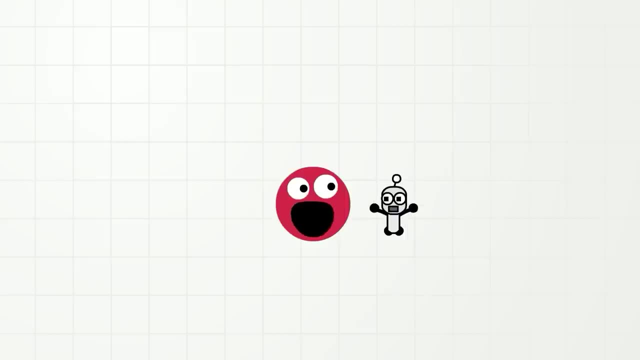 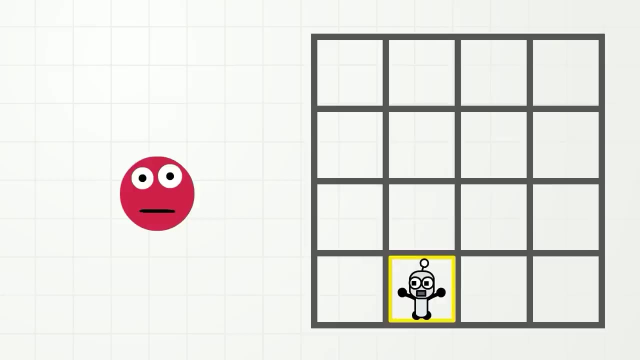 Ha hi, Tiny Robot. So Tiny Robot will start here. Ok, So we need to tell Tiny Robot how to get to the number of squares. and the Tiny Robot is hungry. Luckily, there is a plate of spaghetti here. We need to tell Tiny Robot how to get to the plate of spaghetti using these four different 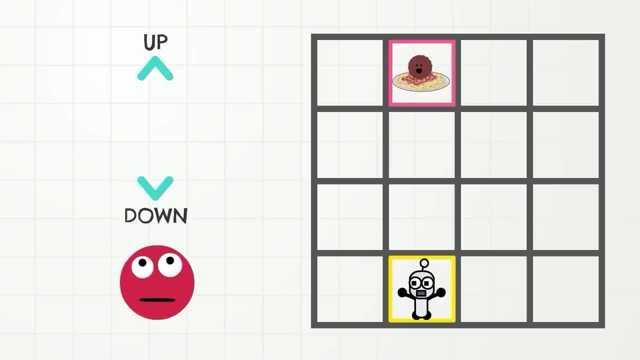 directions: Up down, left and right, And we need to tell Tiny Robot the distance or how far to go using the number of squares. Ok, now Which direction should Tiny Robot go? Maybe we could do the first one together. 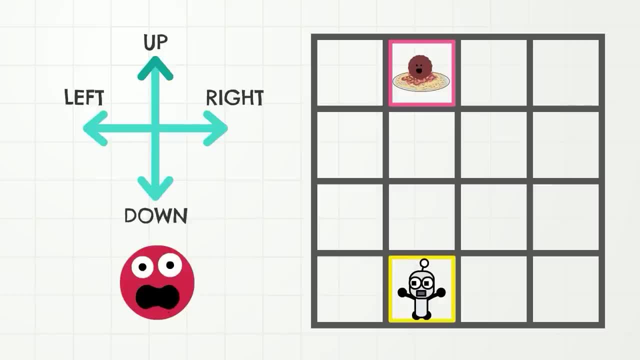 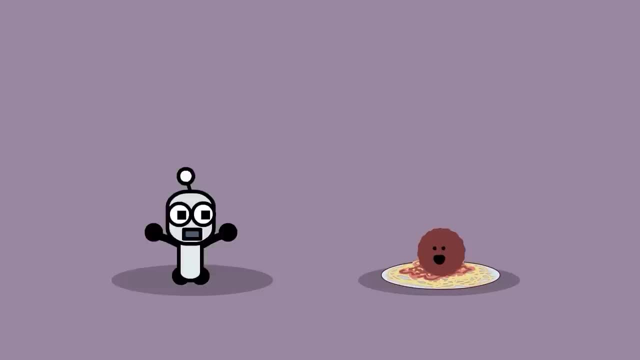 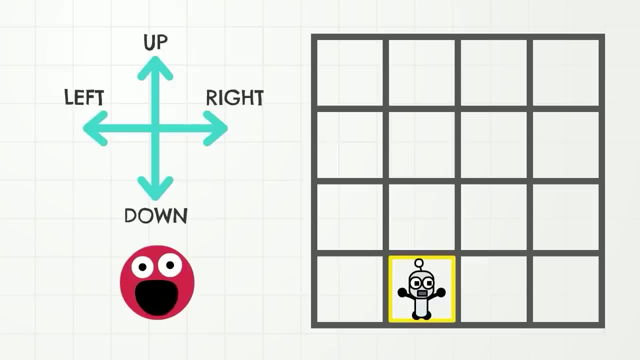 I think Tiny Robot should go up three squares: One, two, three, Yay, Good job, Tiny Robot. Now let's play again. Tiny Robot is still hungry and wants another plate of spaghetti, But this time Tiny Robot has to watch out for the other plate. 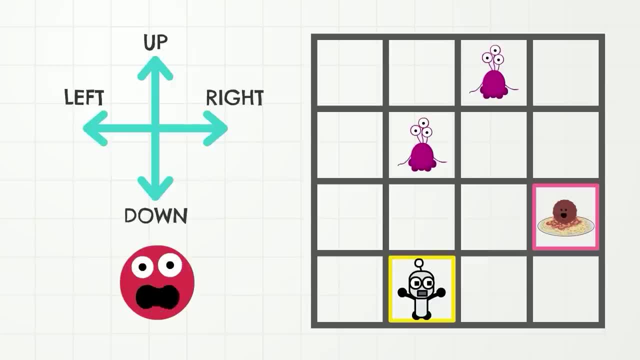 But this time Tiny Robot has to watch out for the other plate of spaghetti. But this time Tiny Robot has to watch out for the other plate, has to watch out for monsters and cannot go on the squares with the monsters. So what way should? 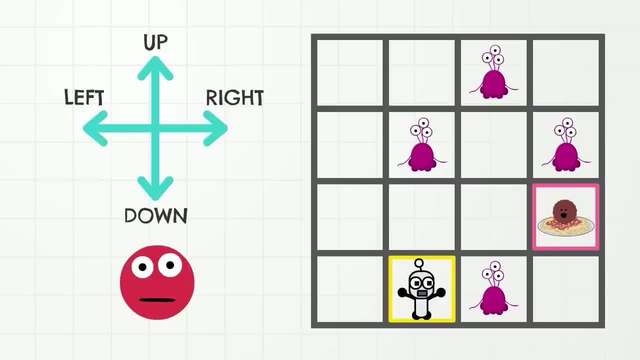 Tiny Robot go first. Yeah, I think Tiny Robot should go up. But how many squares? Yes, One square. So now, what direction and how many squares should Tiny Robot go? What's that? OK, Tiny Robot go right. two squares. 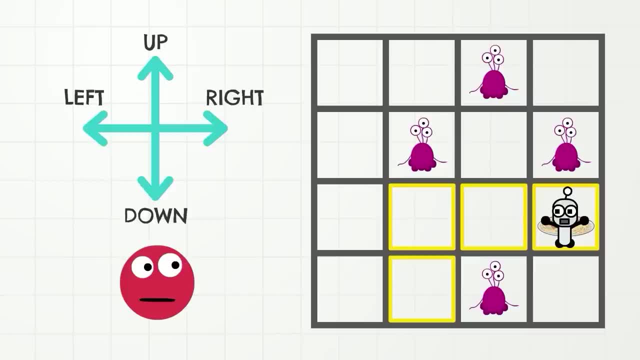 One, two, Yeah, Good job Tiny Robot. OK, let's play one last time. And Tiny Robot is still hungry for spaghetti. Wow, This time it is going to be more difficult, because Tiny Robot has to watch out for monsters, volcanoes. 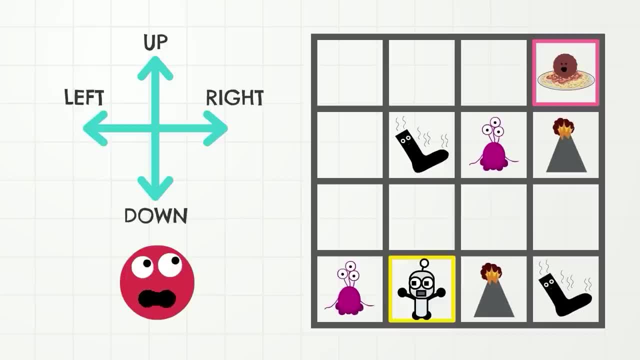 and stinky socks. Oh, so stinky. Now I need you to tell Tiny Robot where to go. Remember to say the direction and also how many squares. OK, go First. Tiny Robot should go, which direction Up And how many squares. 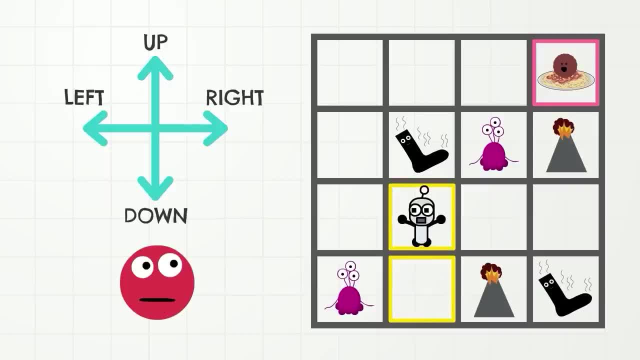 One square. Now Tiny Robot should go. which direction Left. And how many squares? One square. And now Tiny Robot should go which direction Up? And how many squares? One, two squares. And now Tiny Robot should go which direction? 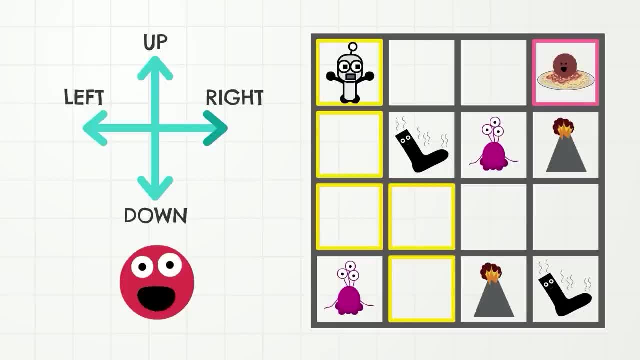 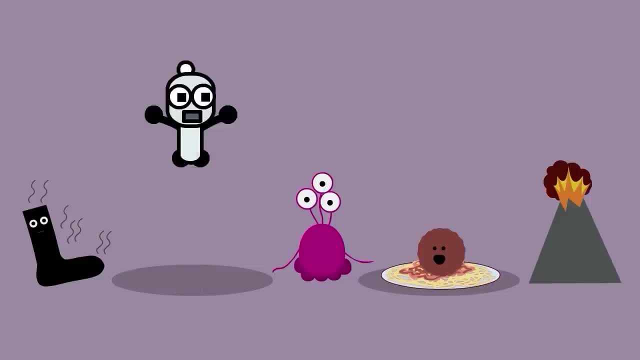 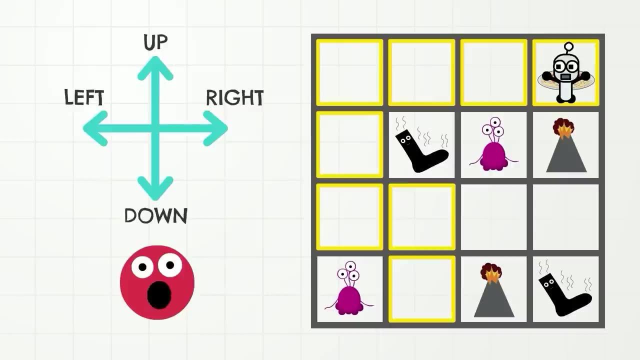 Right. How many squares? One, two, three squares. Good job, Tiny Robot. Good job everybody. I'm so happy you did not touch the stinky socks, So stinky. OK, that is all the time we have today for location. 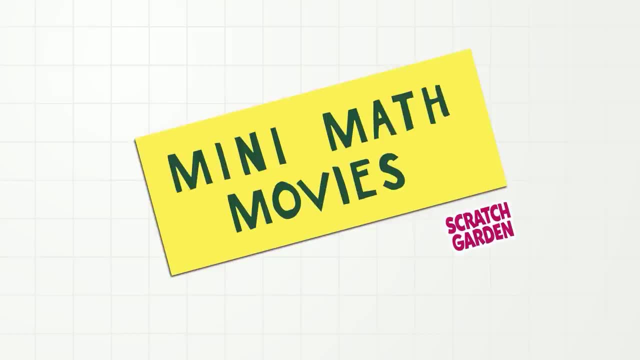 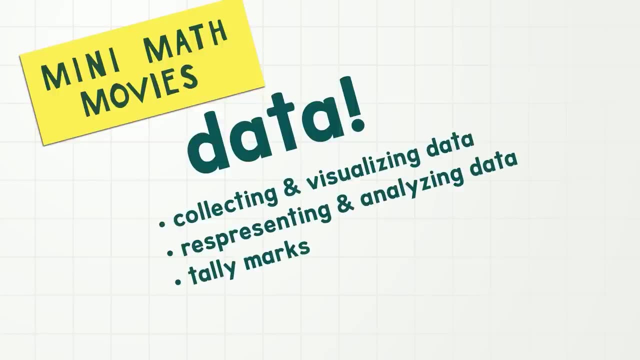 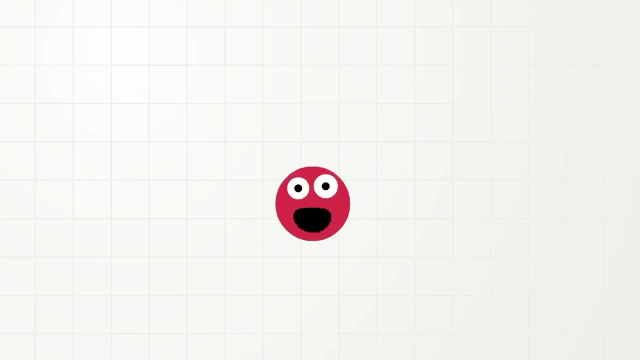 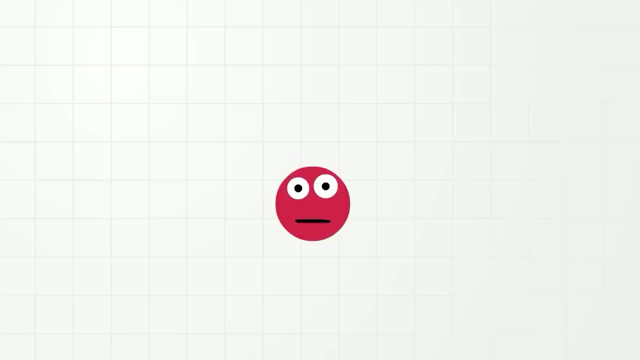 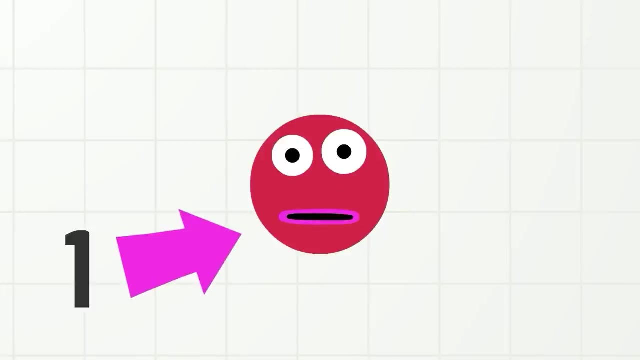 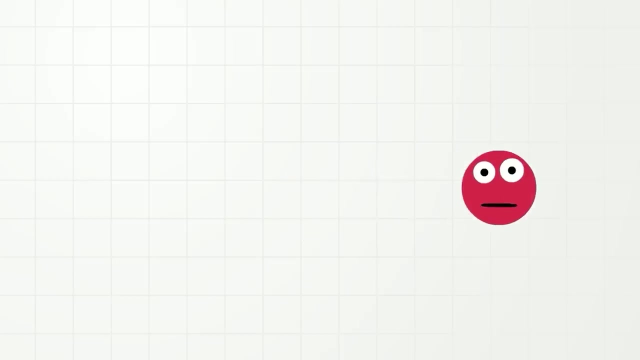 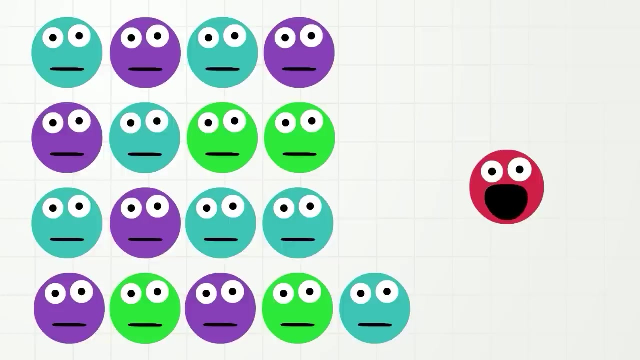 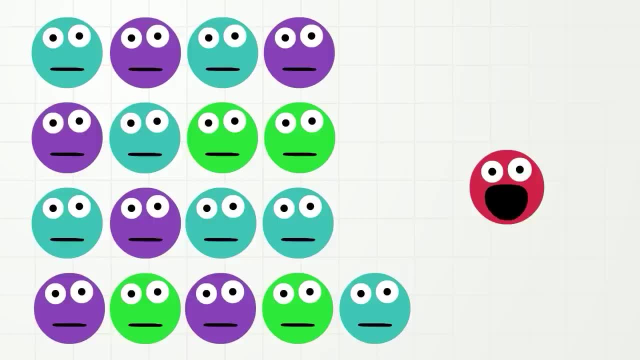 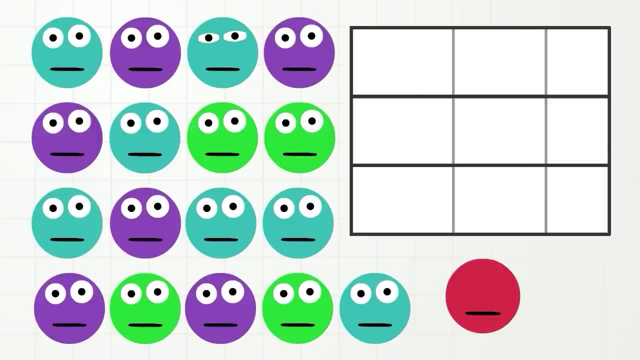 what color they are. Do you want to help me? Okay, great, We can use a chart and write down the numbers beside the words of the color up here. First up is purple. So how many brothers and sisters are purple? Let's count one, two, three, four, five, six, six. hey, do you know what these are? 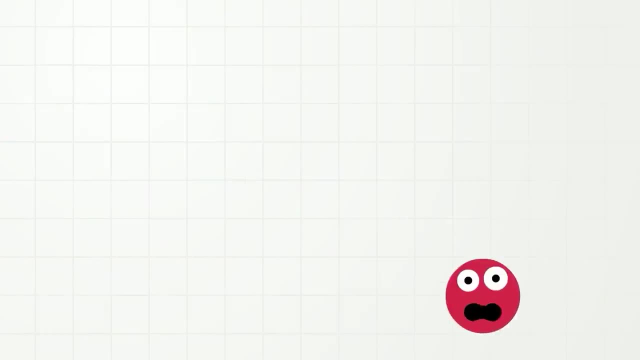 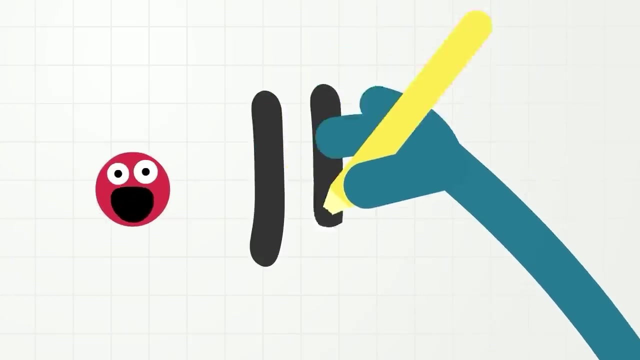 These are tally marks, Tally marks. Tally marks are like a way of counting using special lines. When we count with tally marks, we make one up and down line for each number, up to four, like this, And then, when we get to five, we make a side to side line. 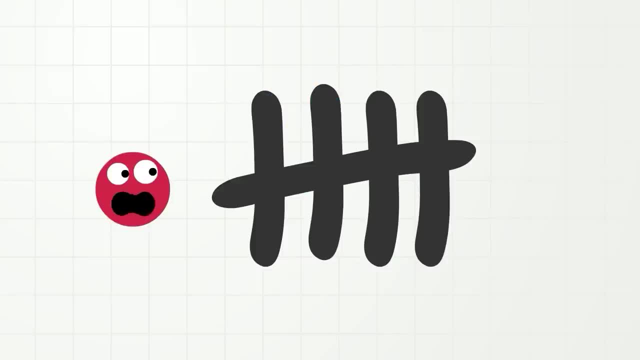 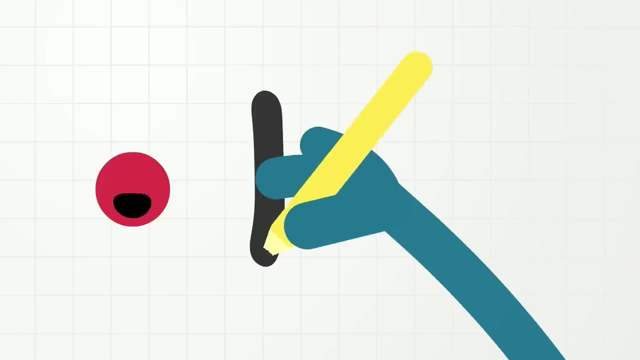 Side line through like this: And now we know we have a group of five. But after five, well then, we start all over again and make a new group. So when we count up to six, this is how we do it with tally marks. 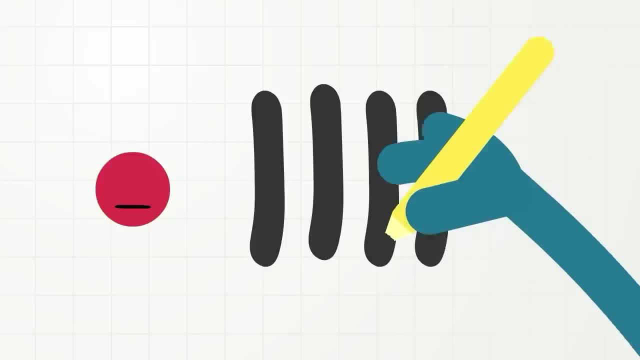 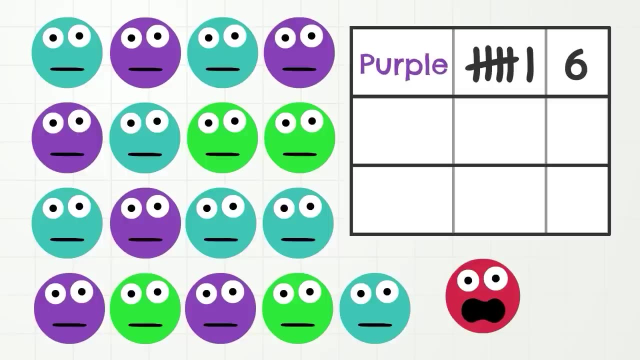 One, two, three, four, five and six. Okay, moving on. The next color is green. How many brothers and sisters are green? Let's count one, two, three, four, four And, finally, how many brothers and sisters are blue? 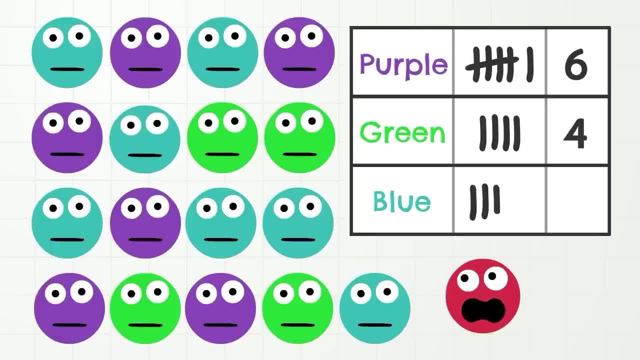 Let's count one, two, three, four, five, six, seven, seven. Good job, everybody. We have now collected all the data about the color of my brothers and sisters. Yay, Okay, you've done such a good job. it is now time to take a stretching break. 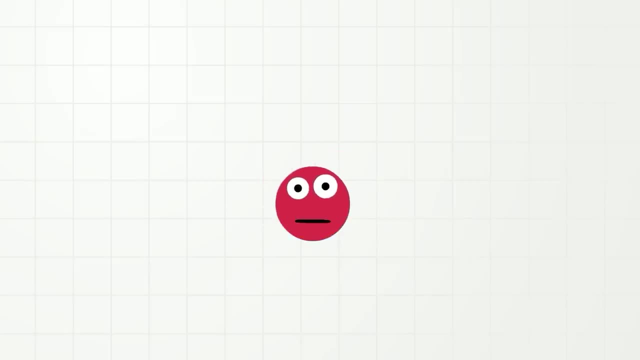 Ugh, Yeah, Okay, that's enough. So we just saw that we can collect data and understand things by observing with our eyes, But did you know that we can also collect data and understand things by asking questions with our voice? Oh, yes. 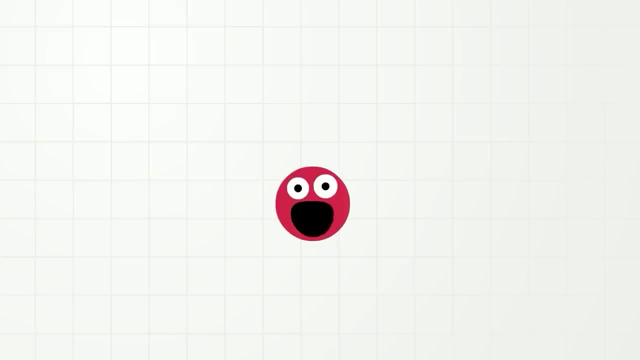 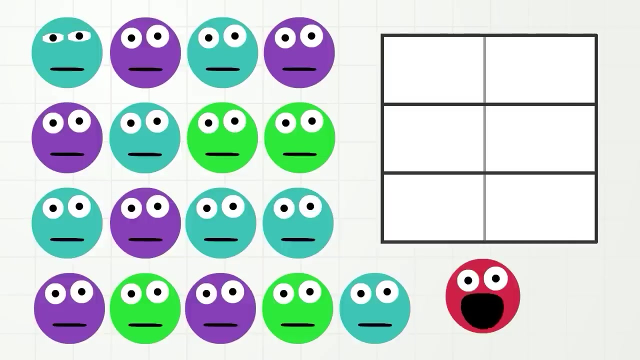 Yes, we can. Okay, let's ask my brothers and sisters some questions and collect their answers with tally marks. Okay, what should we ask them about? Hmm, Oh, I know, bugs. I said bugs. Okay, there are three different kinds of bugs here. 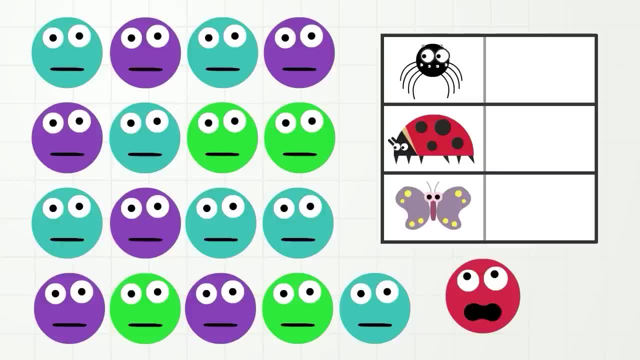 Spider, ladybug and butterfly. I want to know which one is which, Which one is which, Which one is which, And I want to know which bug they like the best. So we just saw that. Hey, who's talking? 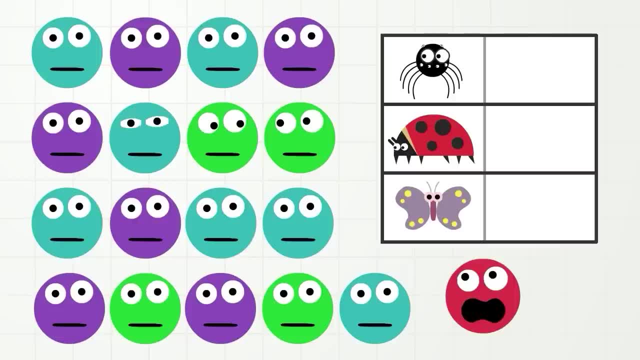 Ugh, Francis and August, you need to separate. Please move. OK, that's better. Now, brothers and sisters, I want you to raise your hand when I say the name of the bug that you like the best, And remember you can only choose one bug and raise your hand one time. 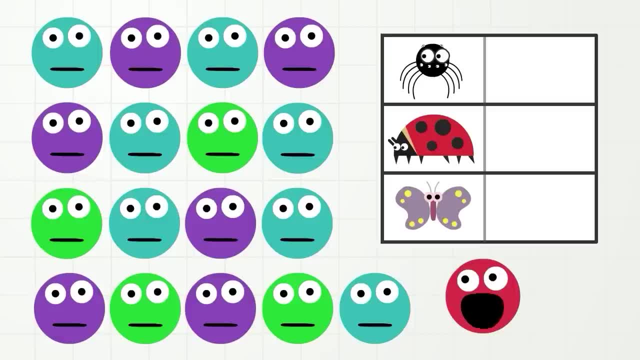 That's right, Okay, I'll do it. Okay, Okay, please raise your hand. if you like spiders the best, Let's count One, two, three, So three brothers and sisters like spiders the best. Now raise your hands. if you like ladybugs the best. 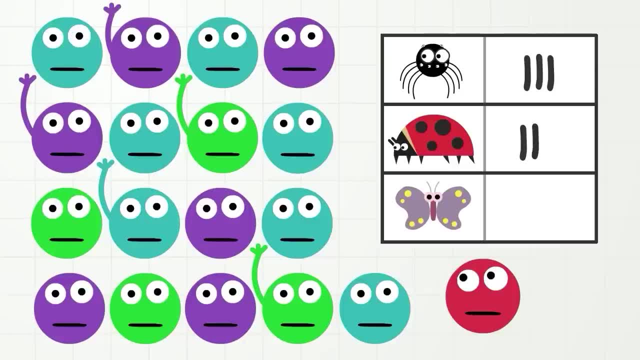 Let's count One, two, three, four, five. So five brothers and sisters like ladybugs. the best. Now raise your hand if you like butterflies, the best. Let's count One, two, three, four, five, six, seven, eight, nine. 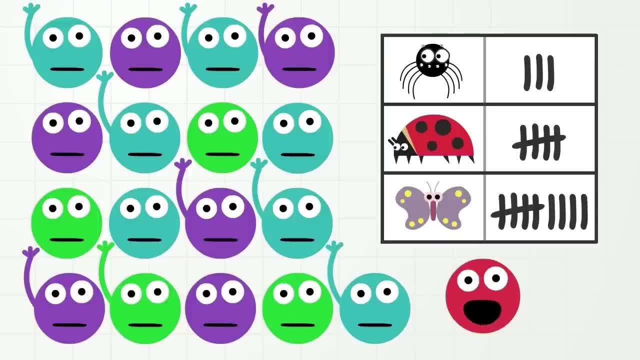 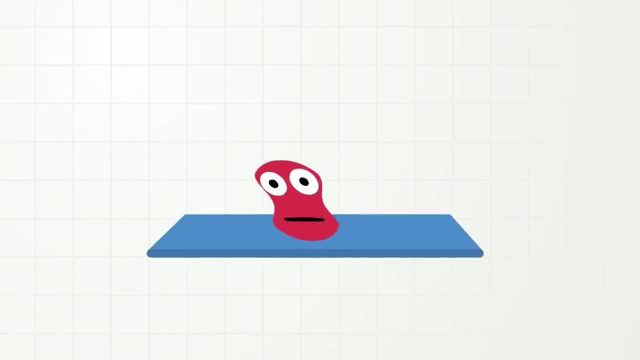 So nine brothers and sisters. like a butterfly, the best, Wow, Great, collecting data everyone. Now let's take a look at the next one. Let's take a break and do some stretching. Oh yeah, Feels good. Okay, that's enough. 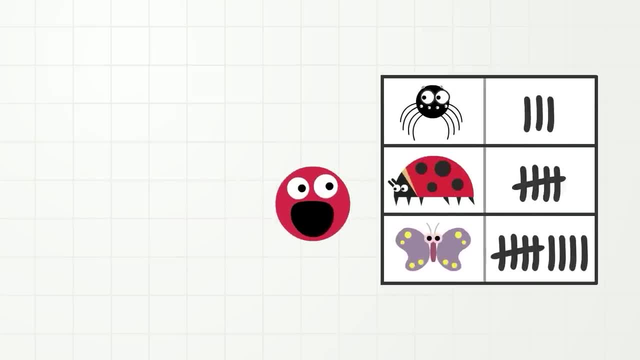 Now let us show this data in a different way. Instead of using tally marks, we will take the numbers and put them into something we call a pictograph. Pictograph- A pictograph is a way to show data with pictures. Okay, so remember how many brothers and sisters like spider best. 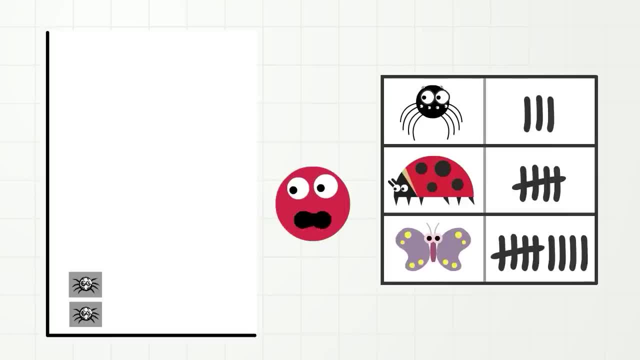 That's right three, One, two, three. And how many like the ladybug the best? That's right five, One, two, three, four, five. And how many like the butterfly the best? That's right nine. 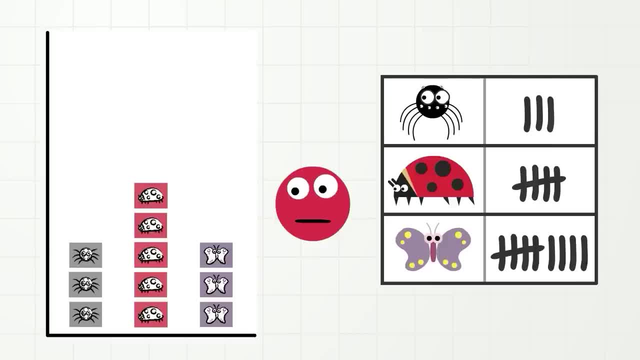 One, two, three, four, five, six, seven, Eight, nine, And now our pictograph is complete. So, looking at the pictograph data, which bug do most of my brothers and sisters like the best? That's right, it's a butterfly. 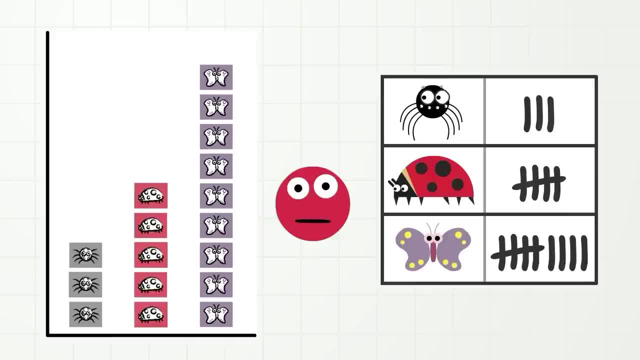 Yay, There are more butterfly pictures than anything else. So we have learned that among my brothers and sisters, the most popular bug is the butterfly. And which bug? The most popular bug is the second most popular bug. That's right, it's a ladybug. 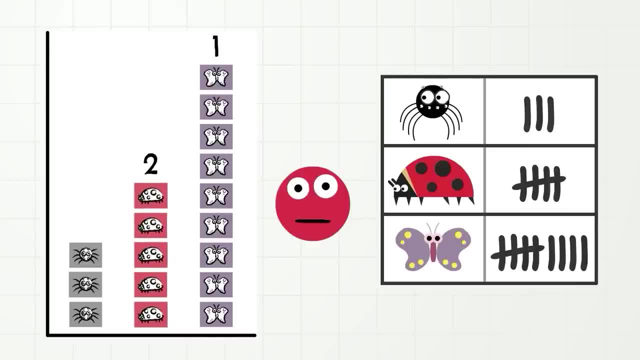 Yay. Oh, here's a question: How many more ladybugs would we need to have in order to equal the amount of butterflies? If you said four, you are right. Yay, And finally, what is the third most popular bug? 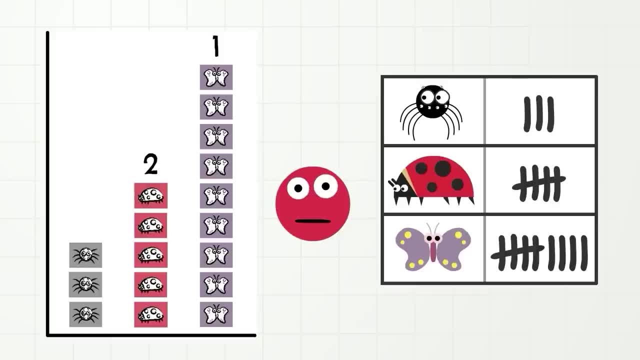 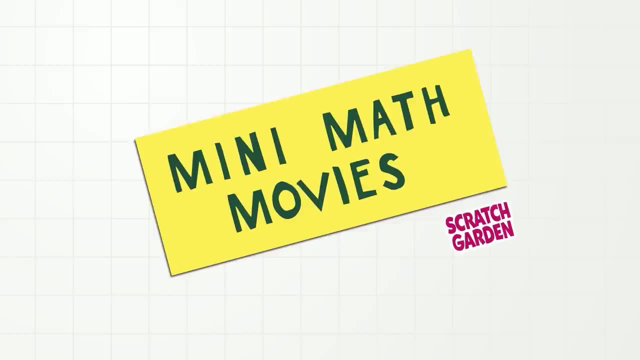 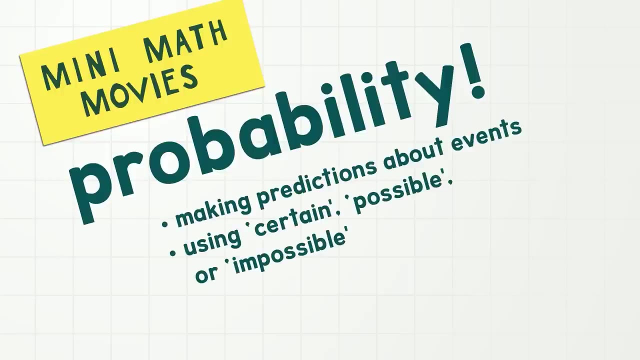 Or we can also say the least popular bug. That's right, it is spider. It's okay spider. I still like you. Okay, that is all the time today we have for data. Oh, hi, everybody Today. 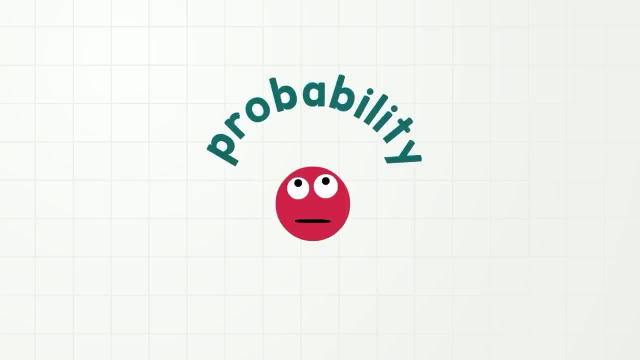 I'm going to talk about the most popular bug, the spider, And today I'm going to talk to you about probability Probably, No, not probably. Probability Probably, Actually, you say it like this: Probability, Probability, Yay. 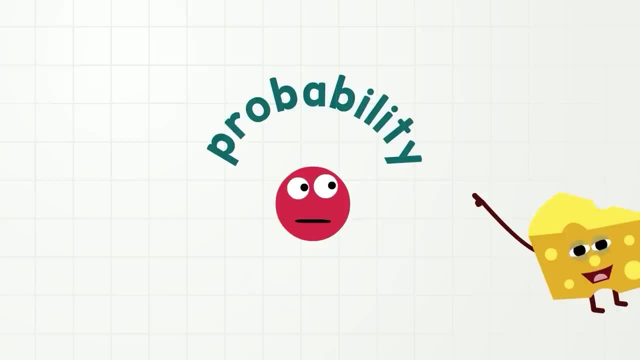 You got it Okay. So probability is kind of like thinking about if something will happen or won't happen or will happen Okay. So what will maybe happen? For example, tomorrow I will eat dinner. I know that this is true because I eat dinner every day. 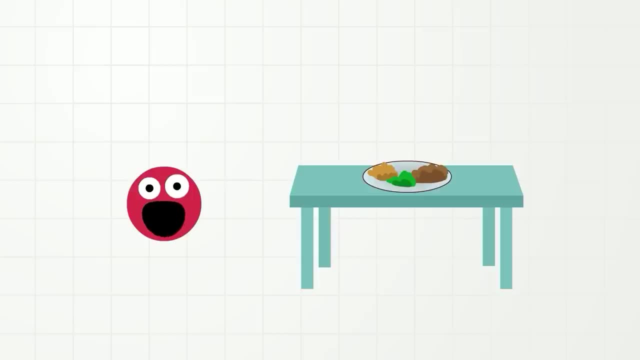 And if we know that something will happen, we can also say that it is certain. Certain, Let's say it together: Certain, Yes, One more time Certain. But I wonder what I will eat for dinner. Hmm, What about rocks? 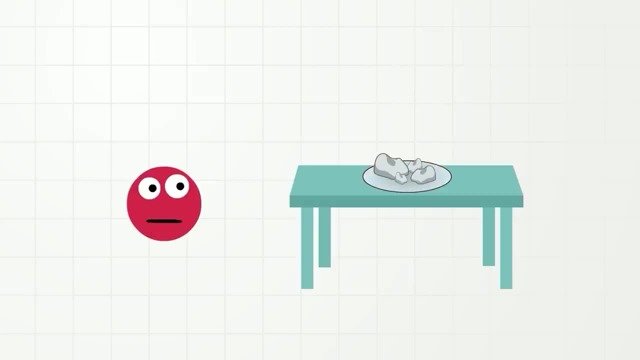 I say rocks. Do you think that I will eat rocks for dinner? No, I won't eat rocks for dinner. I know this because rocks are hard and they do not taste good and they could be very dangerous to eat. So I know that I definitely won't eat rocks. 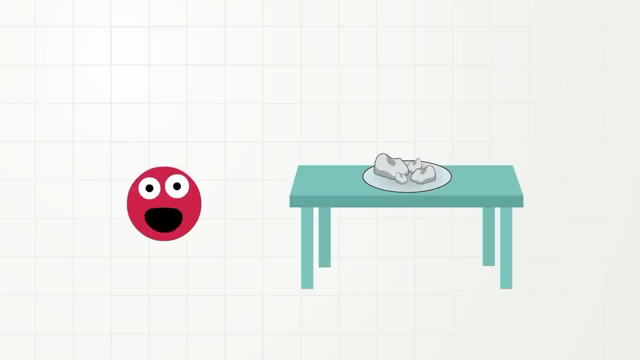 And if we know that something won't happen, we can also say that it is certain. So let's say that it is impossible. Impossible. Let's say it together: Impossible. Yes, One more time: Impossible. So if I'm not going to eat rocks for dinner, I wonder if I will eat a plate of spaghetti. 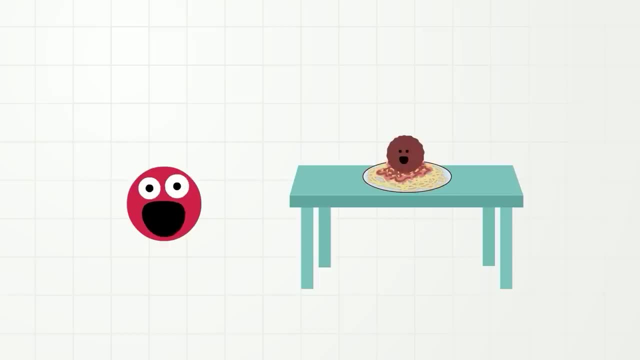 You know, I have had spaghetti before for dinner and I like to eat spaghetti. so I think that maybe I could eat spaghetti for dinner, And if we know that something will maybe happen, we can also say that it is possible, Possible. 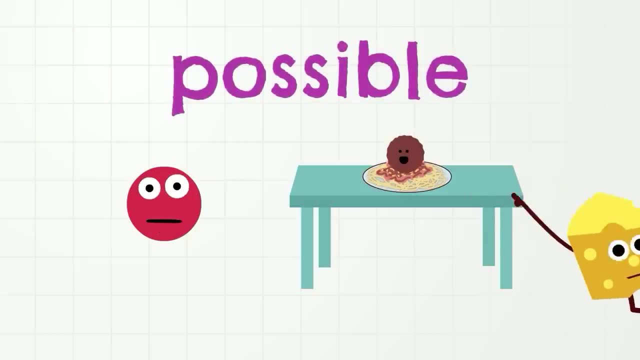 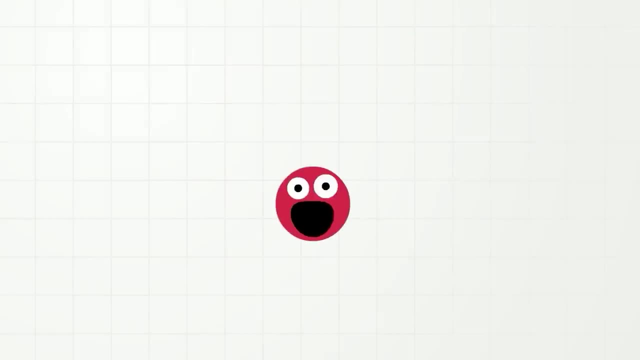 Yeah, Let's say it again: Possible? Yeah, One more time Possible? Okay, Let's take a break. I think it is a good time to… Juggle. Okay, That's enough. So I am now going to tell you some things that are not possible. 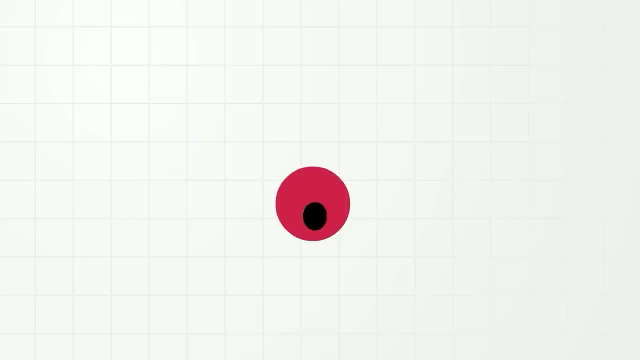 Possible, Possible, Possible, Possible. I want to tell you some things that could happen after dinner, And I want you to tell me if you think that it is certain that it will happen, or if it is possible that it could maybe happen, or if it is impossible, which means it won't. 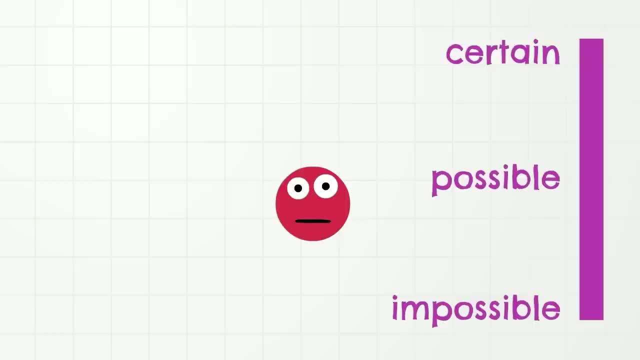 happen. Oh and, by the way, there are also many other words we can use when thinking about probability, For example, likely and unlikely And many others, But today I want to practice mostly the words certain, possible and impossible. Okay, ready. 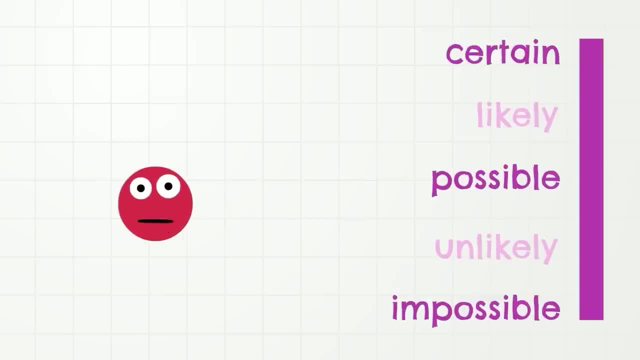 Situation number one: After dinner, I will fall asleep. Do you think that this is certain, possible or impossible? Well, I fall asleep every night, So I think that this is something that is certain. Situation number two: After dinner, I will fly to the moon and meet a dwarf named Betty. 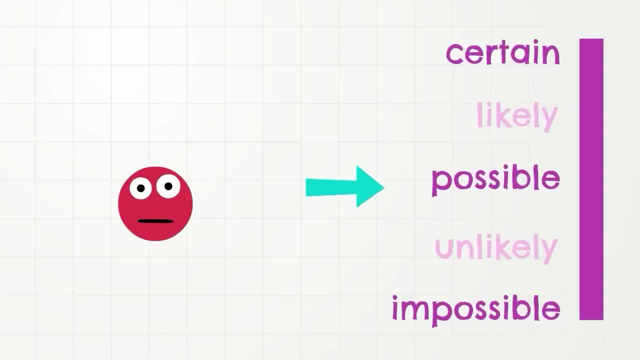 Do you think that this is certain, possible or impossible? Well, I've never been to the moon before, And I don't have a rocket ship, And I don't think dwarves live on the moon, So I think that this is something that is impossible. 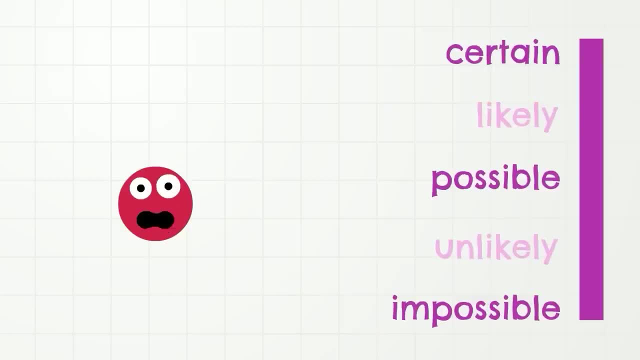 Situation number three: After dinner, I will read a book. Do you think that this is certain possible or impossible? Well, I sometimes read a book before I go to bed, So I think that this is something that is POSSIBLE. 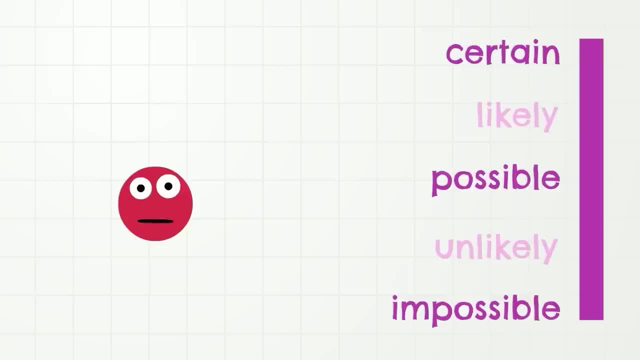 Okay, I now have some probability situations for you, But first let's take another break and Juggle, As I was saying. now I am going to say some things about what you could do after your dinner And you can tell me whether they're certain. 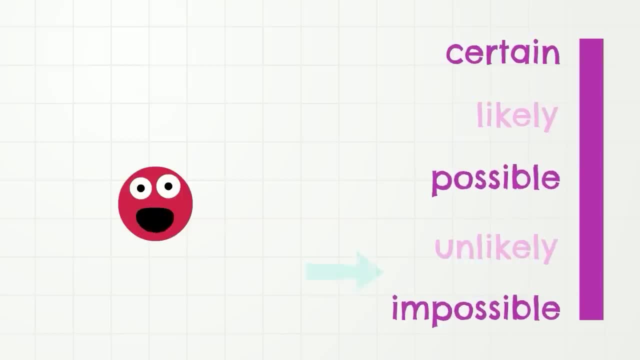 Possible or impossible. 1. After dinner, you will have dessert. 2. After dinner, a unicorn will carry you to bed. 3. After dinner, you will brush your teeth. 4. After dinner, you will dream about unicorns. 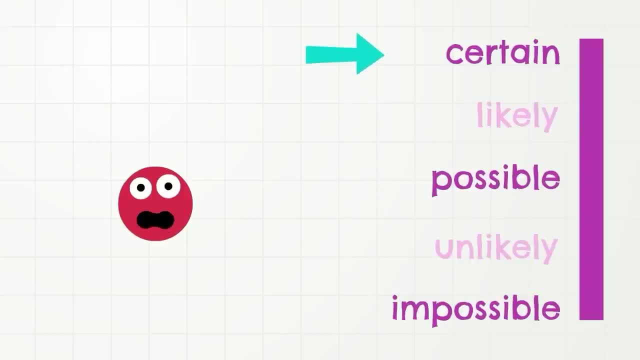 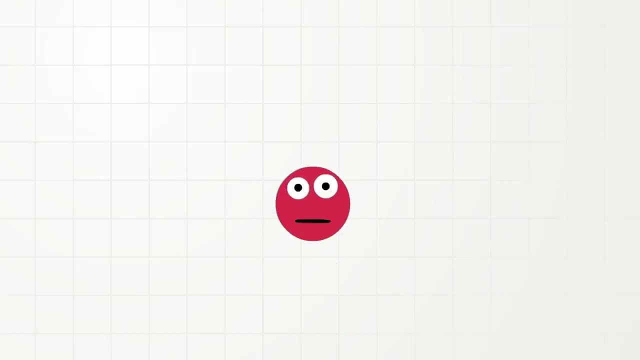 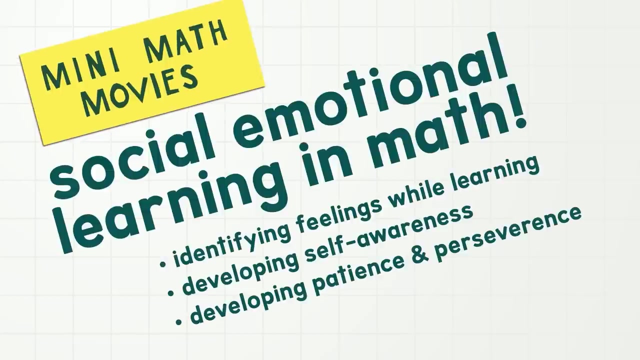 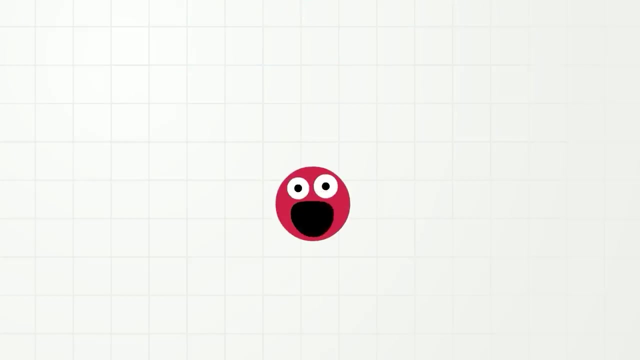 Okay, great answers everybody. And one thing I know for certain is that right now it is time to juggle. Okay, that is all the time today we have for probability. Probability- Oh, hi everybody. Today I am going to talk to you about math and feelings, and maybe even fish tanks. 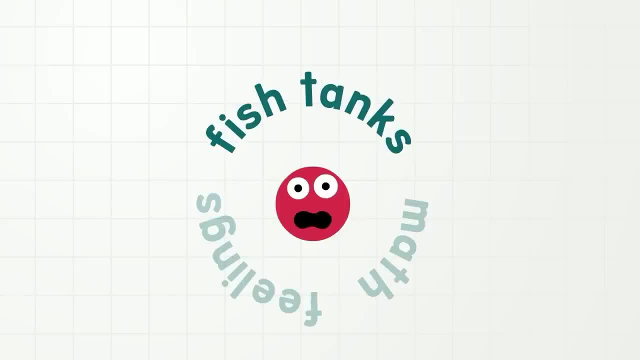 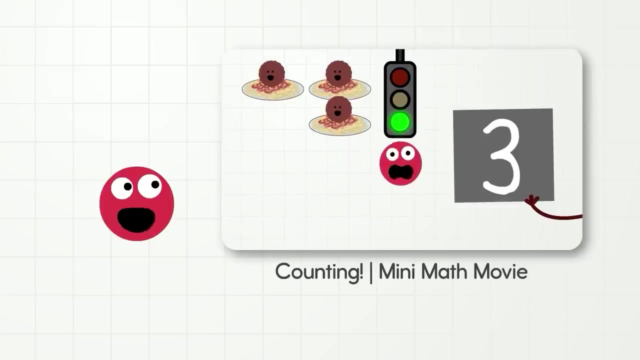 Oh, I really like fish tanks. Okay, everybody knows that math is just a game. It's just about numbers, right? Actually, nope, Math is about so much more than numbers. Math is about many things like counting plates of spaghetti. 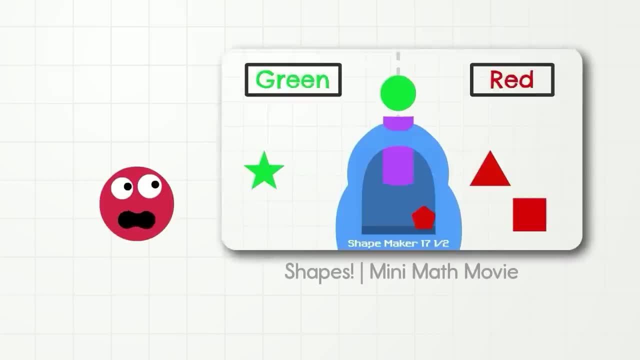 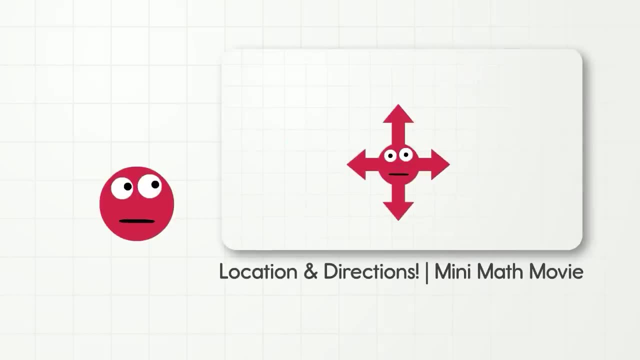 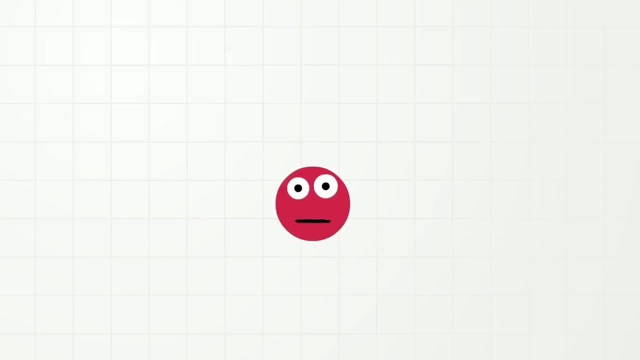 patterns, sorting shapes, adding donuts, directions, subtracting donuts, tally marks and so many other things. And did I say donuts? And just like there are many different things to learn in math, there are also many different ways to learn math. 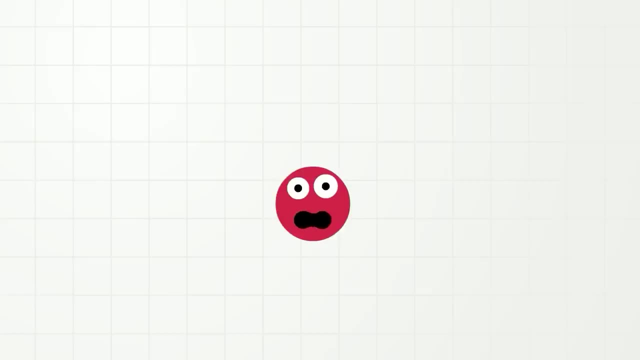 And no, I'm serious. For example, do you know how to count to five? Yes, of course you do. Let's count to five together. Are you ready? Go? 1,, 2,, 3,, 4, 5!. 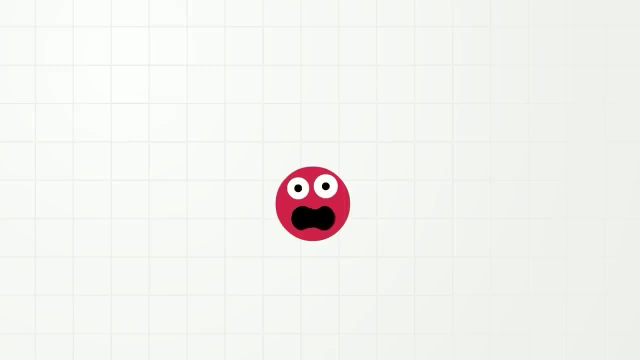 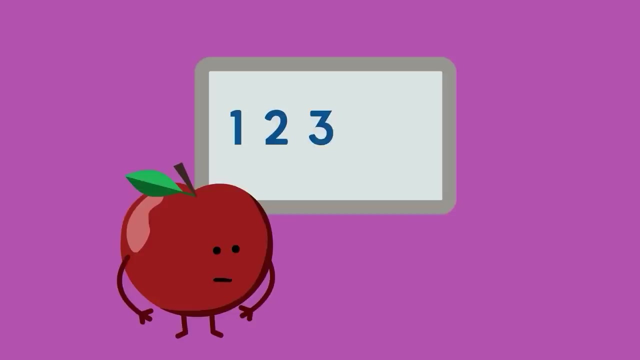 Yay, Good job. So we just counted to five out loud with our voices. But there are other ways to count to five too. For example, when counting to five, Apple likes to look at the numbers 1,, 2,, 3,, 4,, 5!. 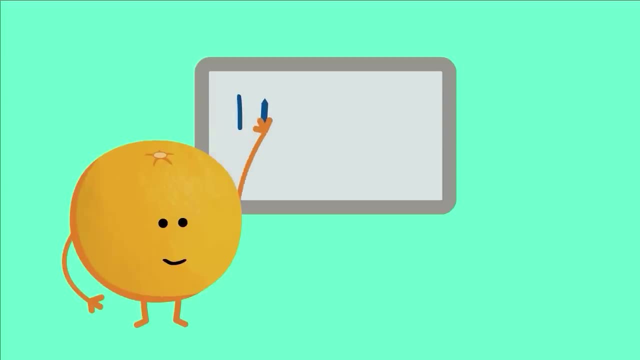 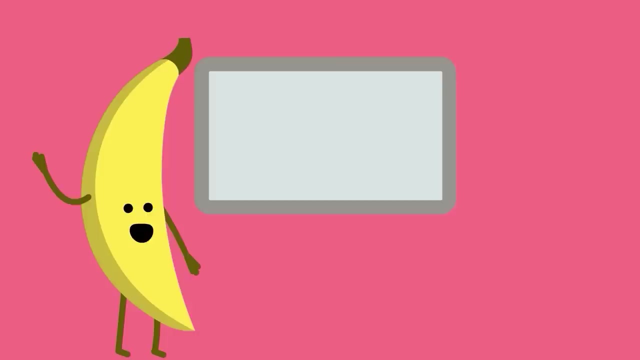 Orange likes to write the numbers 1,, 2,, 3,, 4, 5!. Ladybug likes to see the words of the numbers 1,, 2,, 3,, 4, 5!. Banana likes to use five squares. 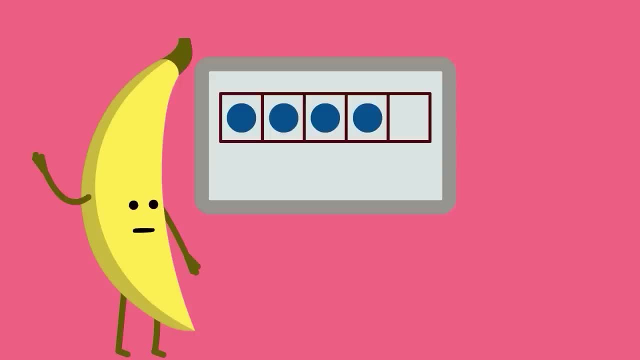 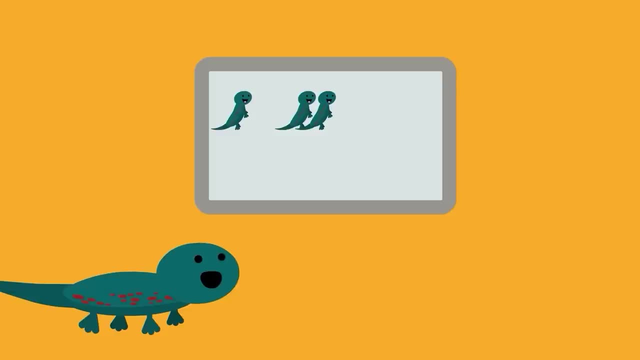 1,, 2,, 3,, 4,, 5! Salamander likes to count salamanders: 1,, 2,, 3, oh, I think that is too many salamanders for three. Yeah, That's better Salamander. 4, 5!. My brothers and sisters like to count out loud and together with each other: 1, 2,, 3,, 4, 5!. A sloth likes to count quietly by itself inside its head: 1,, 2,, 3,, 4, 5!. A scratch garden likes to count with a dog: 1,, 2,, 3,, 4,, 5!. A scratch garden likes to count with a dog: 1,, 2,, 3,, 4,, 5!. A scratch garden likes to count with a dog. 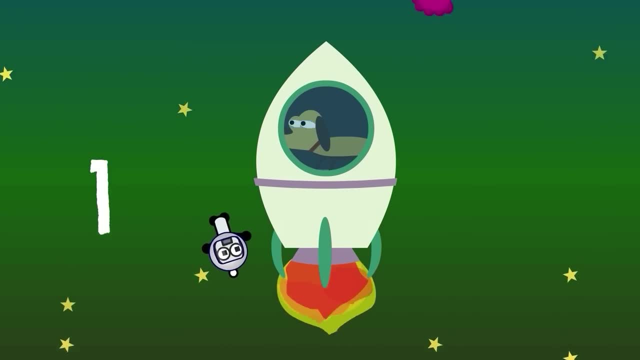 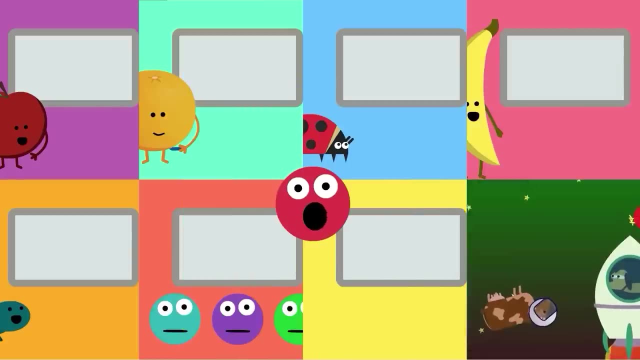 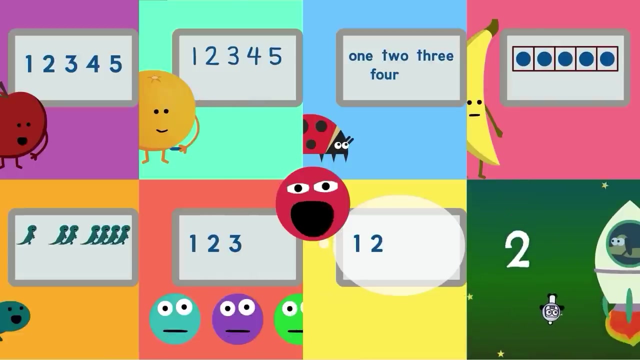 in a rocket ship and with music: 1,, 2,, 3,, 4,, 5!. Wow, Look at all the different ways to count to five. There are so many different ways, And guess what? All of these different ways are great ways to count to five. 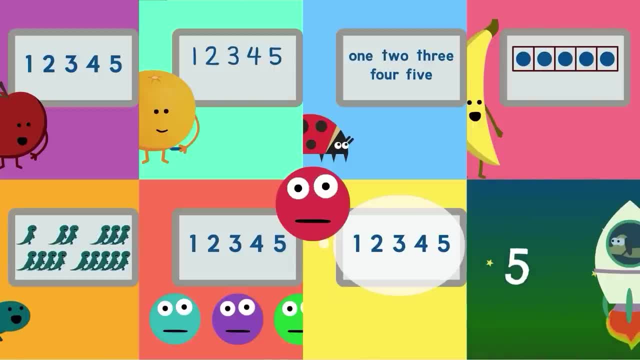 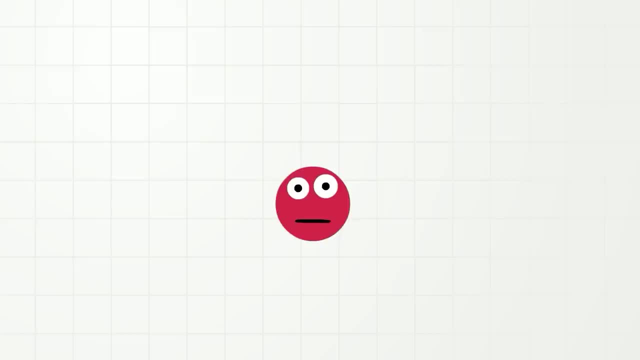 And they are all the right way to count to five. Have you ever thought about which is the best way for you to count to five? A fish tank. Sometimes I like to take a deep breath and watch the fishes, just to think, Ah. 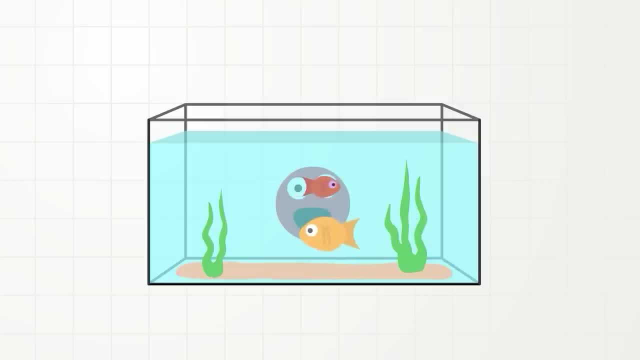 Hmmm. Which way is the best way for you to count to five? Hmmm, And why don't you look around you? Are there other people near you? I wonder what way the like to count to five. count to five, Hmm. Okay, that's enough, And now I have another question. Have you ever thought about 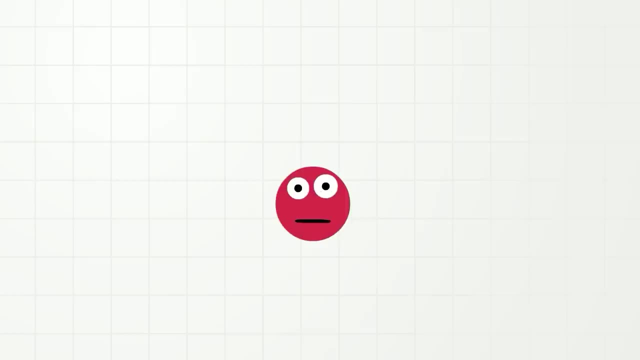 how you feel when you are counting and doing math. Maybe sometimes you love numbers and are happy when you are doing math And maybe sometimes you are sad or frustrated if you don't understand math. But guess what? It is okay to be happy or sad or frustrated And if you can try and understand, 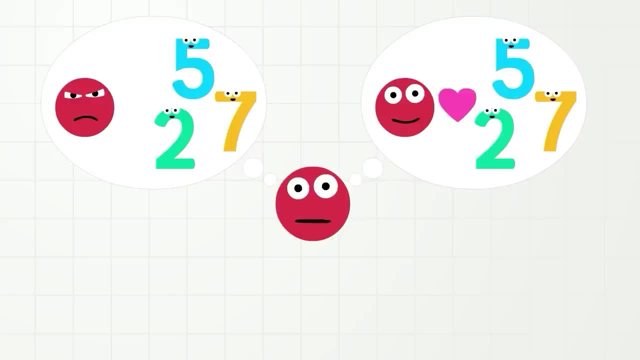 how you feel and talk about how you feel. that is great. Excuse me, Sometimes I don't like doing math because I get nervous if I have to answer questions in front of everybody. Oh, thank you for telling me that That is totally normal. Later we can talk about ways to maybe help you. 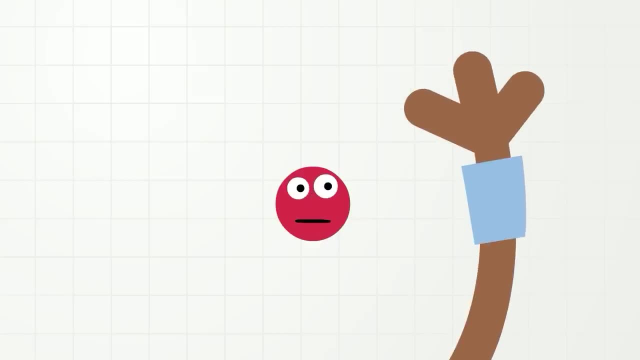 when you are feeling nervous. Also, uh, can I go to the bathroom? No, you may not, Okay. I also want to say that learning math can take a long time. It is okay if you don't understand something right away. It's just like when you were little: You couldn't talk with words. 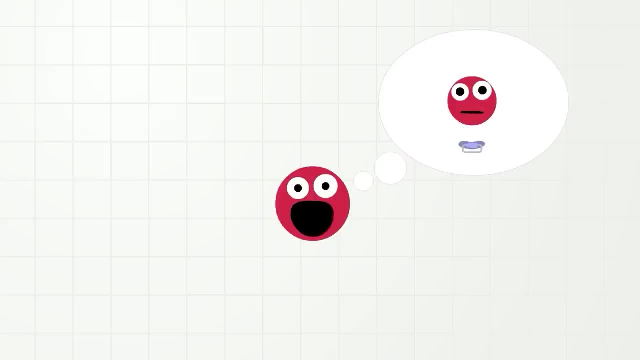 right away. First you just made sounds that sounded like a goo goo ga ga goo, And then you slowly made sounds that sounded like a goo goo ga ga goo. And then you slowly made sounds that sounded like a goo goo ga ga goo. And then you slowly made sounds that sounded like a goo goo ga ga goo.